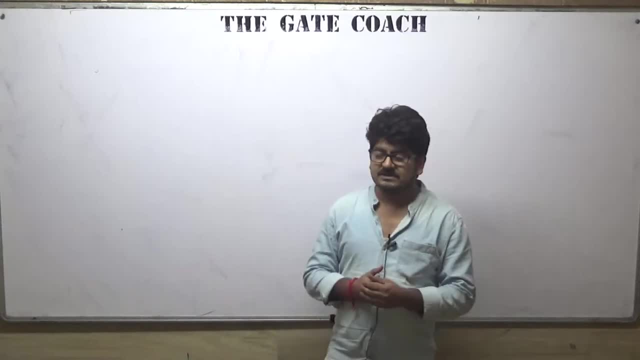 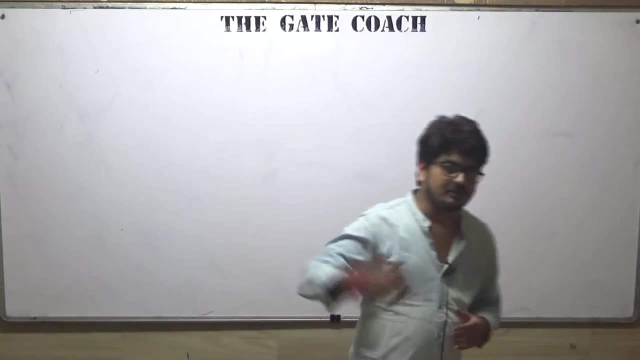 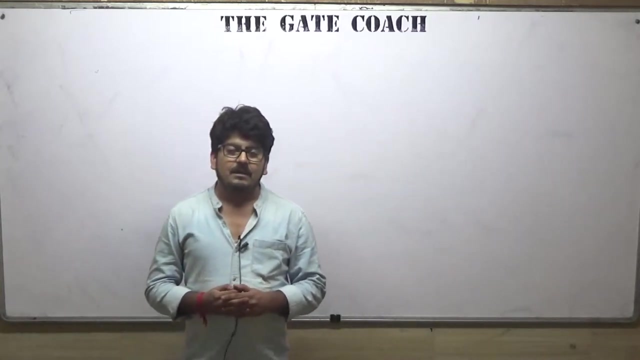 So, guys, next we end on weekends. Obviously, Sunday there is off in our coaching, So we, after this lecture, the second lecture will be on Monday, and then Tuesday, Wednesday, Thursday onwards. Okay, so we will try to cover up this syllabus for GATE 2021 exam. 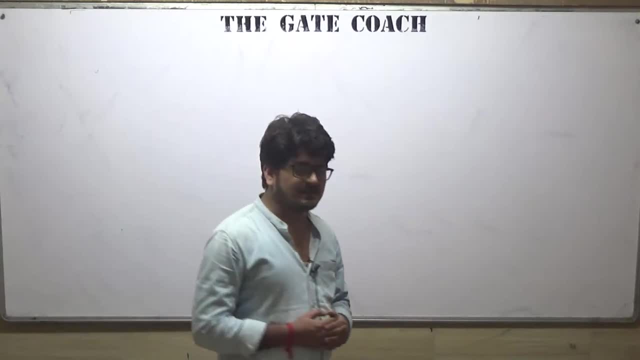 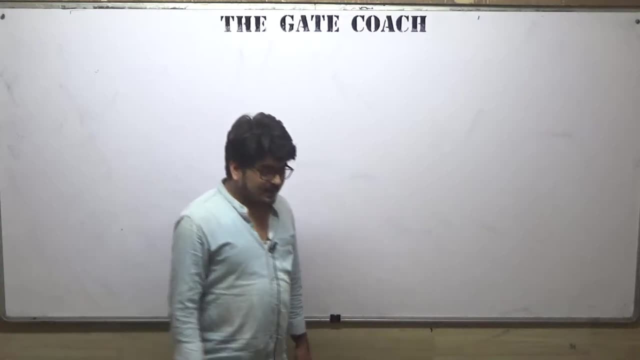 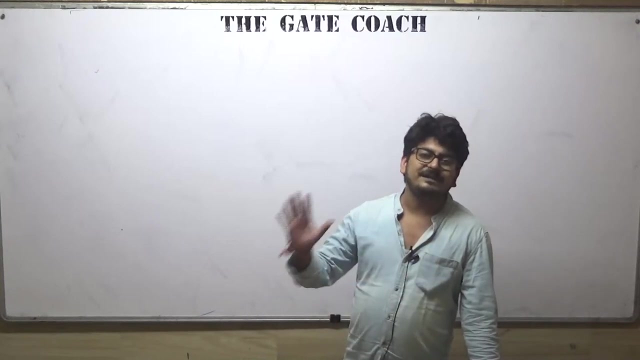 In next four or five classes, And I think it should not be more than four or five hours. It should not take more than four or five hours, but we will see to it. Okay, Here we will discuss the basic idea. Today is the first lecture, that is, that will be completely. 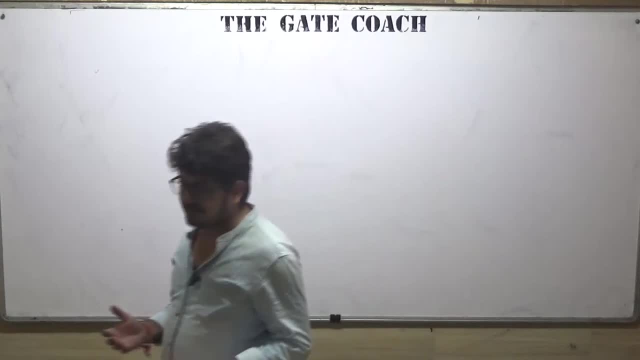 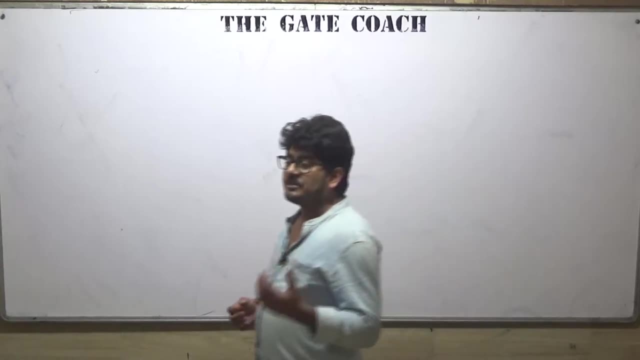 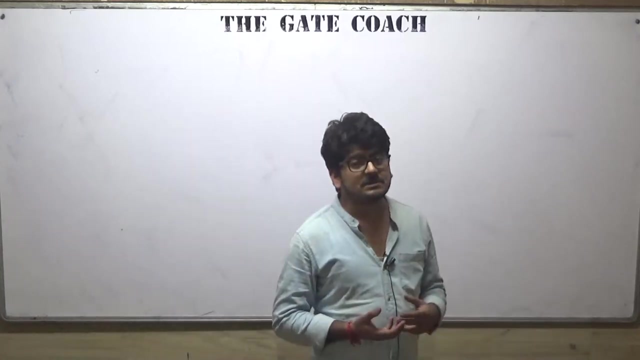 the introductory lecture, where we will discuss about the separation processes: What are the mechanism behind the separation processes, How the separation processes can be classified, What are the basis, What are the methods we use for the separation processes in industries. And then, after all, the membrane separation part, And in this part we will also discuss 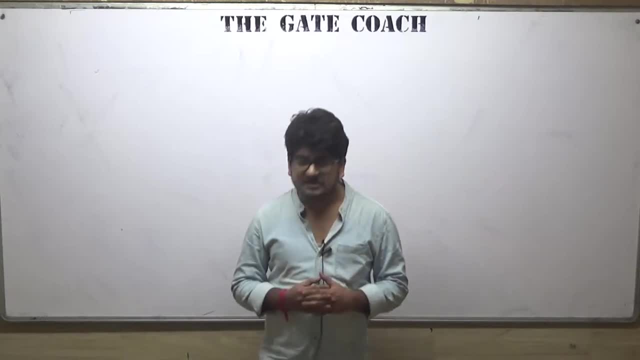 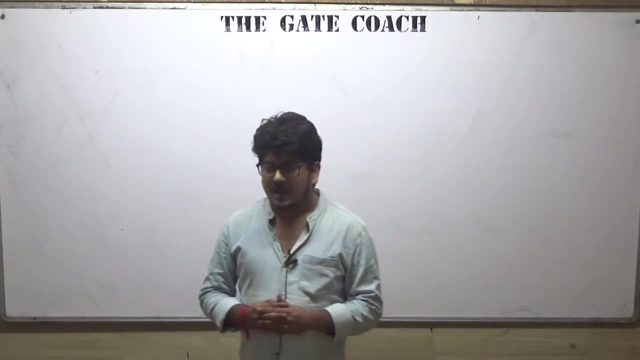 some of the numericals. Okay, as I was seeing the literature, so we have some numericals in our literature, in our books, So we will see to it. okay, I don't know that whether you will get any new kind of numerical or not. 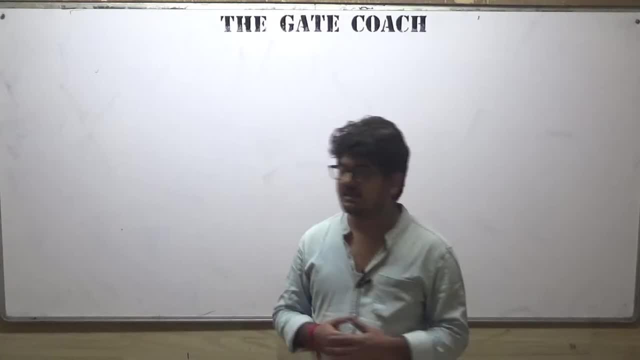 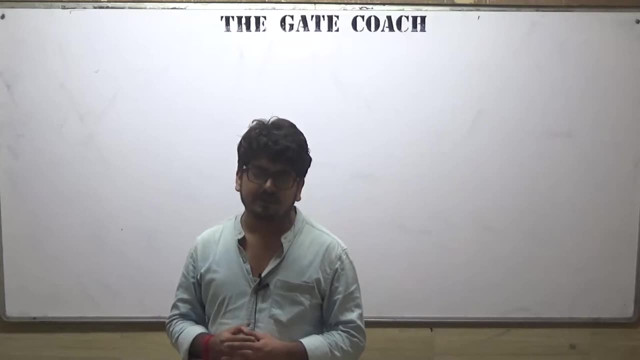 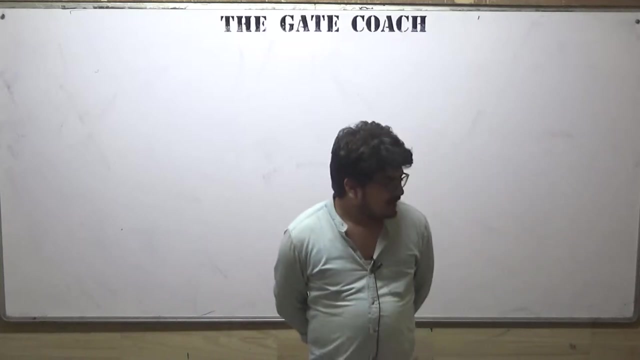 on membrane separation in GATE exam or not, But since it is in your in the books, so we will try to discuss that part as well: The numerical part related to membrane separation. Okay, And if I talk about the books, yeah, this video is live on YouTube and it will. 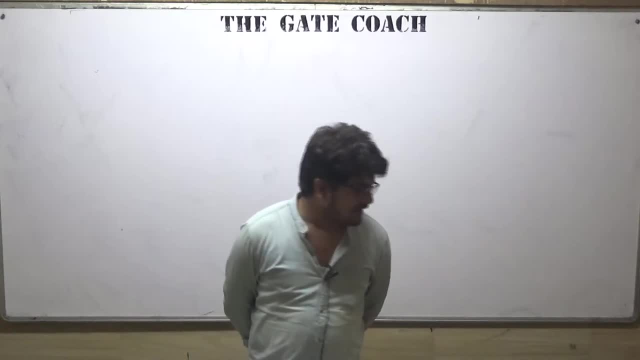 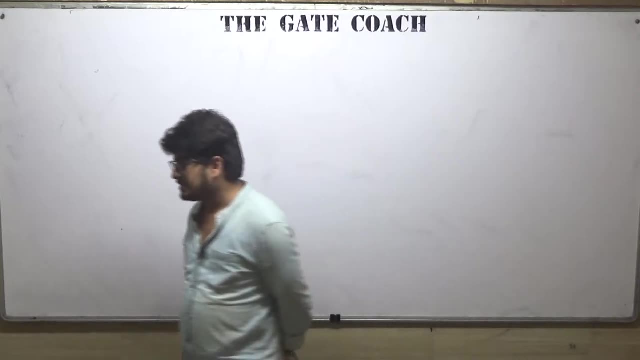 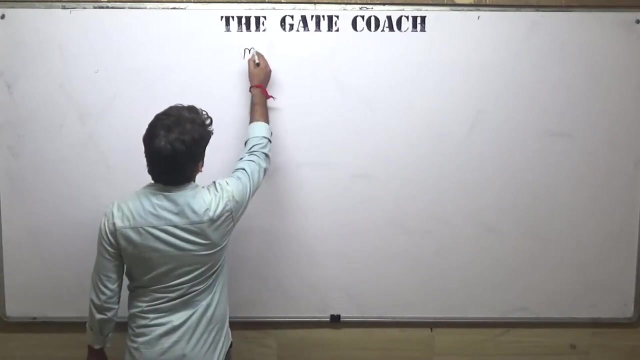 be available on YouTube in the recorded form as well. Okay, And if I talk about the books, what are the books you can refer for the GATE exam, For the membrane separation part? So, guys, let me write the title first: Membrane separation. 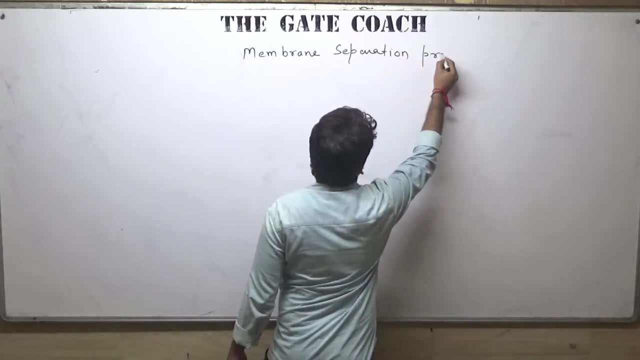 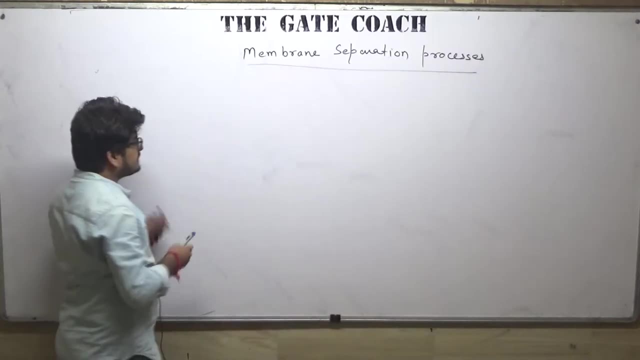 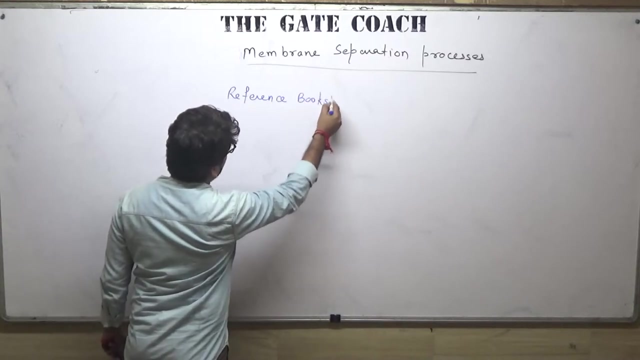 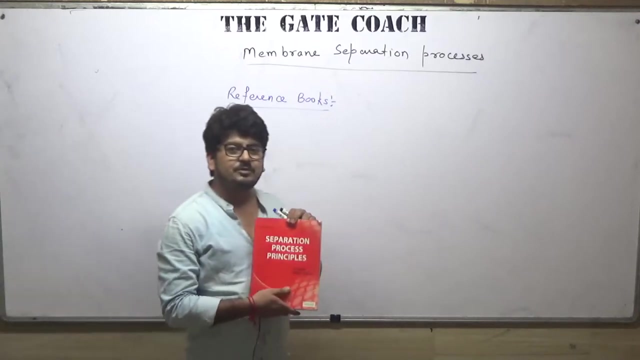 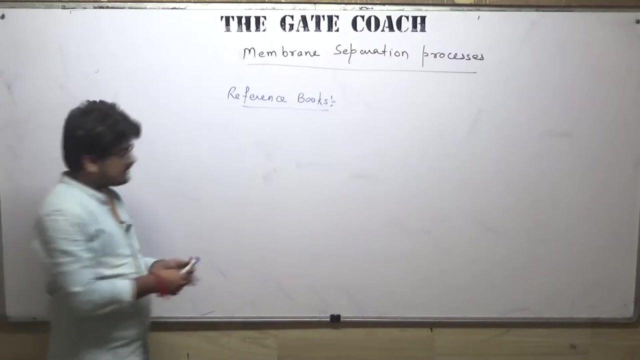 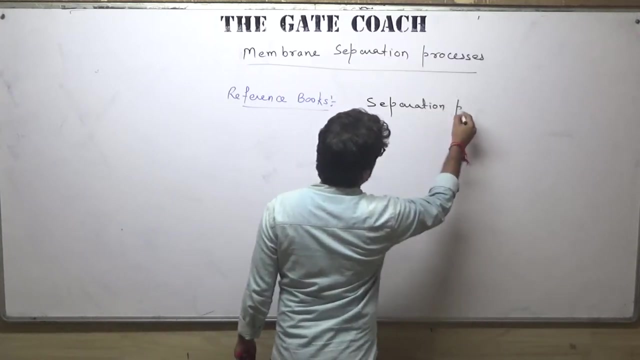 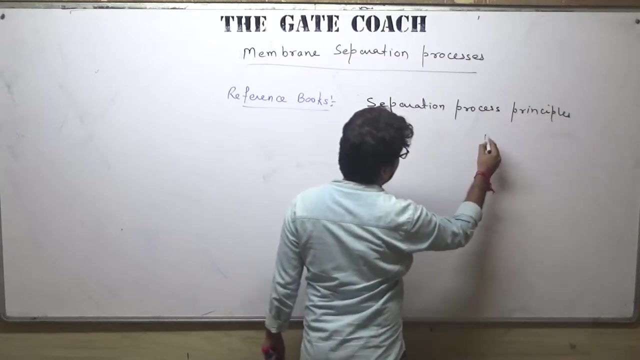 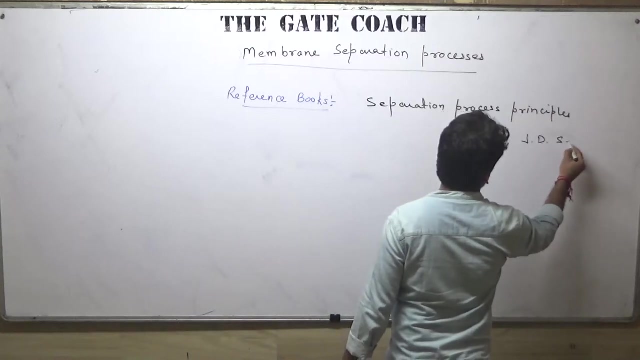 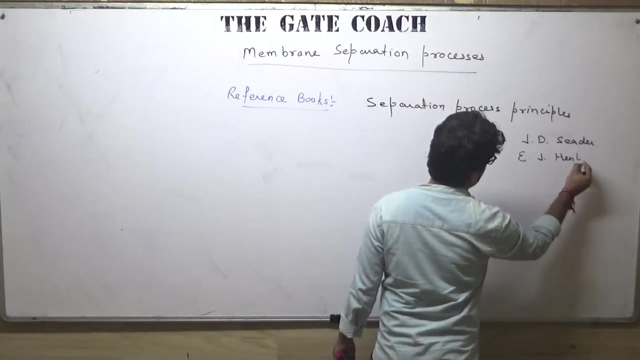 processes, So the reference books which you can follow. The first book is separation process principles by Seder and Henle. Okay, I'm writing the title Separation Process Principles By what is the complete name: JD Seder and EJ Henle. The second book which you 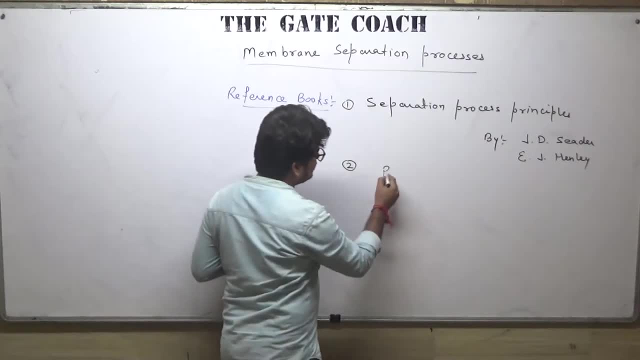 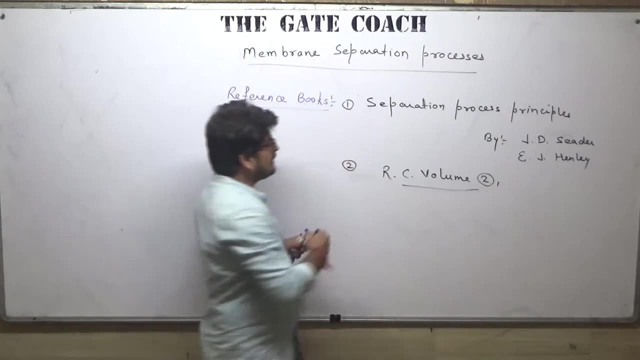 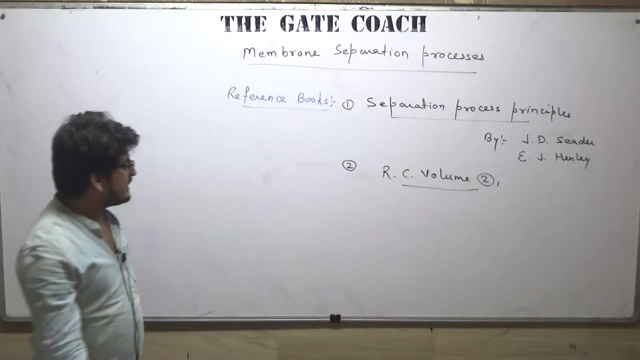 can refer other than this. that is RC volume two. Okay, Okay, Okay, That is separation processes and particle technology. Okay, RC volume. I hope all of you know that is the series of Coulson Richardson's chemical engineering books, The second part. 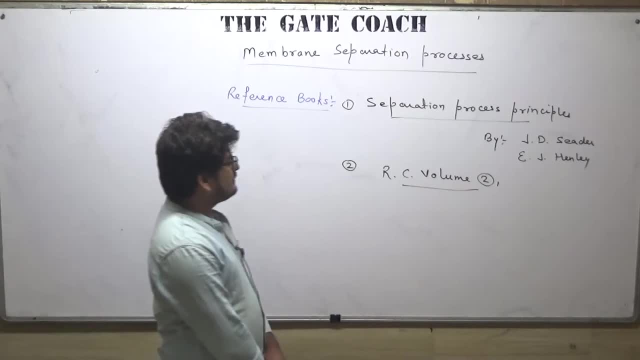 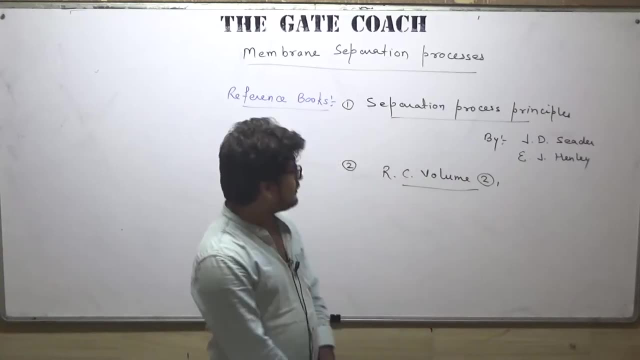 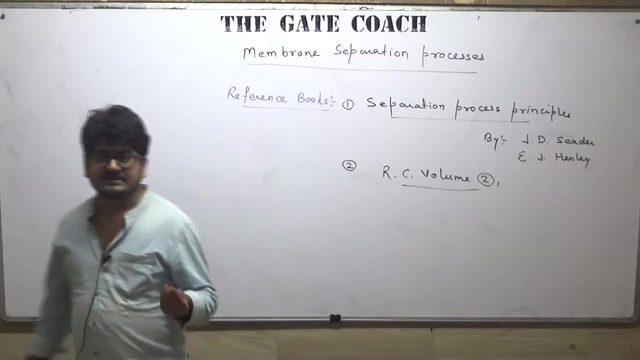 second volume of that series where they have mentioned so many things about the separation processes And for membrane separation. I will suggest to all of you guys to go to the book. And why I'm talking about these two books only? Because the reason is very simple. 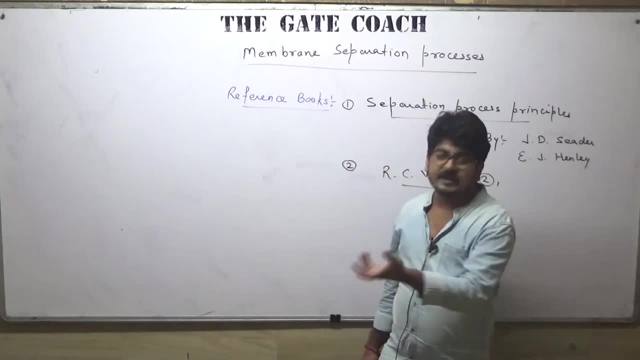 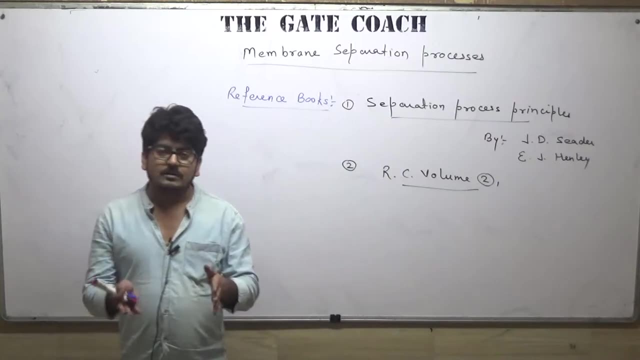 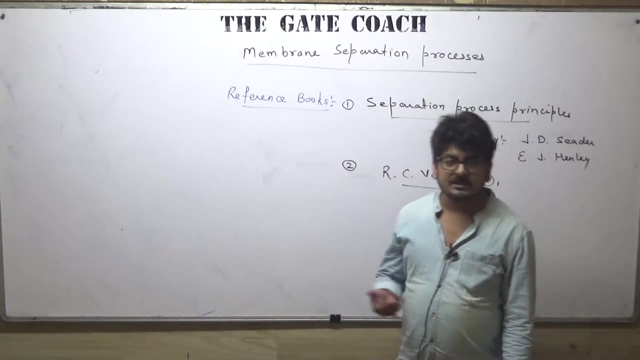 Just try to put yourself in the shoes of a faculty, Okay, Like if you see in your colleges as well, in your university, when I talk about the sessional exams, so there are many faculties, professors who teach us. So if I talk about the sessional internal exams, so obviously 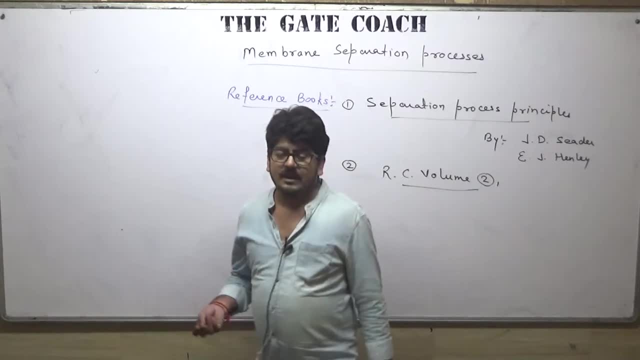 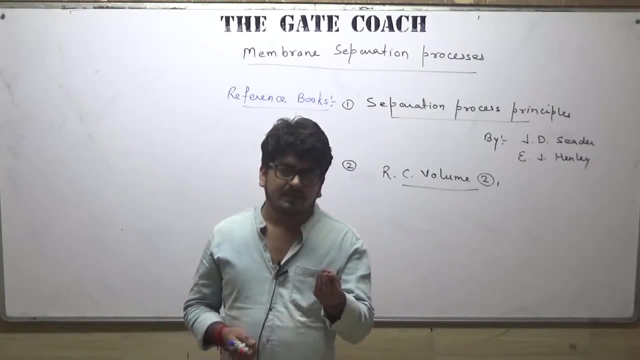 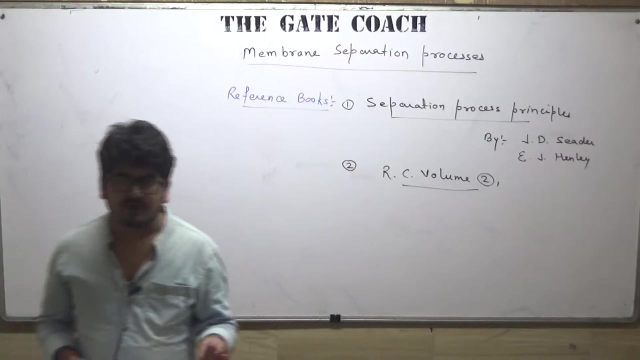 the paper question paper will be set by your own faculty And if I talk about the number of questions, so obviously that faculty will take the questions from the books he is using. he is referring to all of you. Okay, If there is a faculty, for example, who refers to the tray ball for mass transfer in their 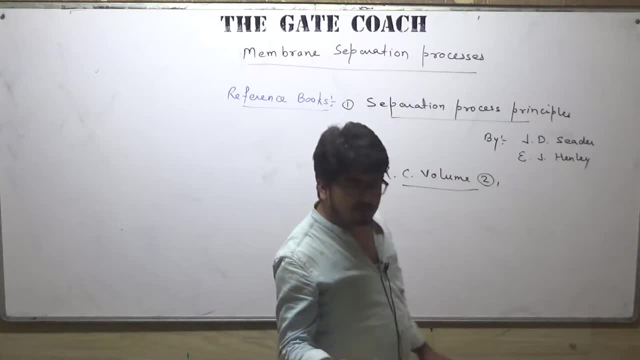 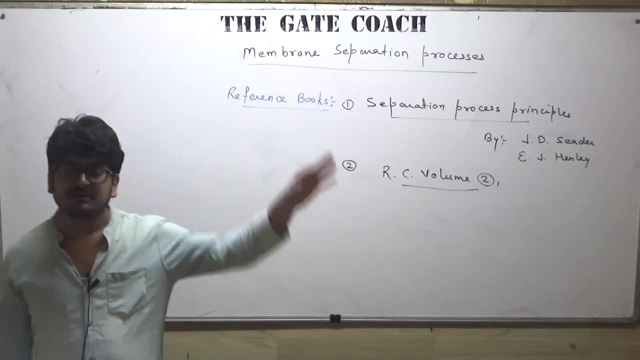 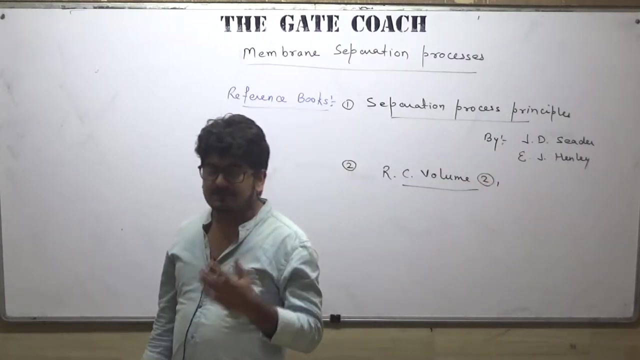 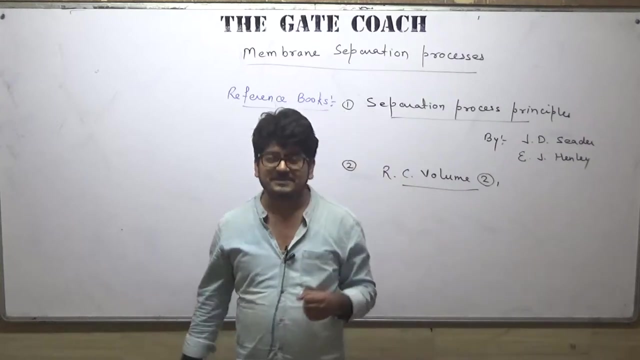 college. then obviously, the exam papers you have, they refer to the tray ball as well. Okay, So it's obvious. So when I was doing my MTech in IIT Delhi, at that time I opt for this subject- membrane separation- for getting some good marks, And I hope you also did the same. 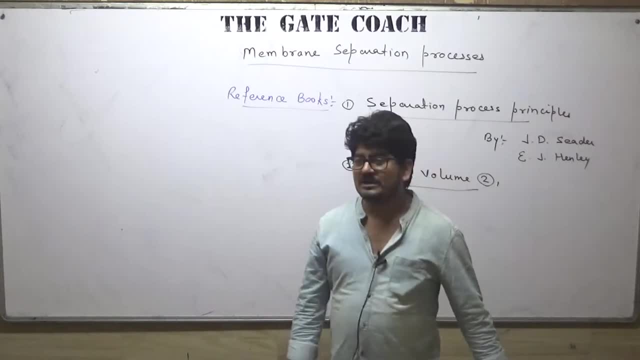 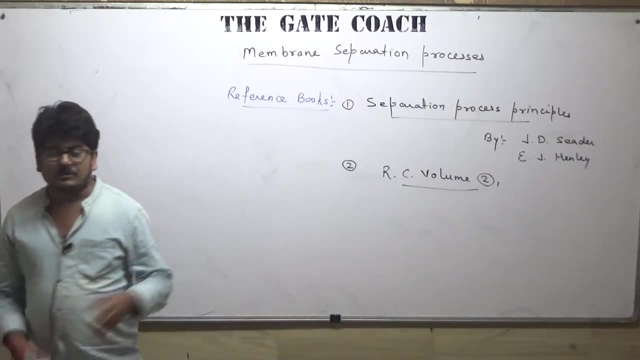 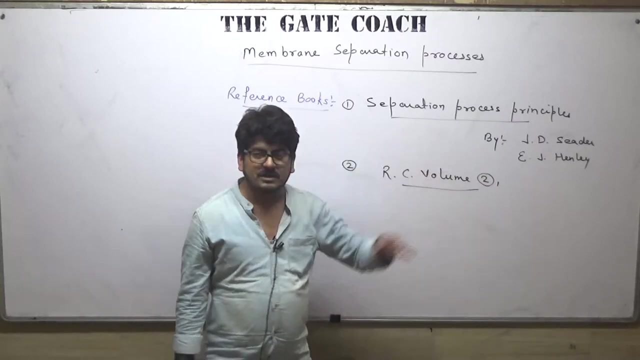 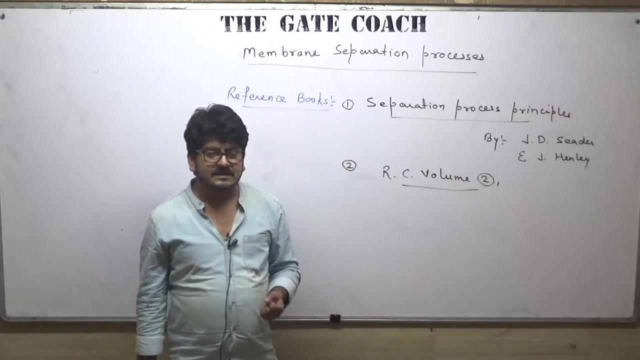 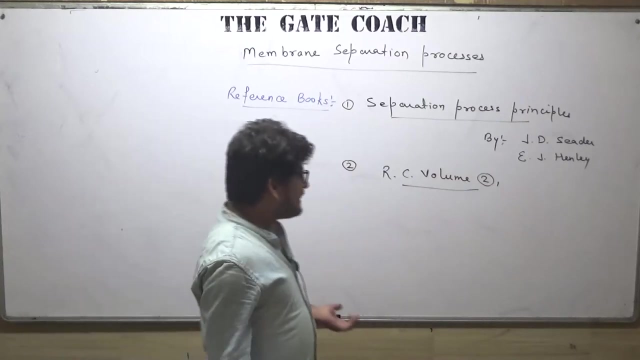 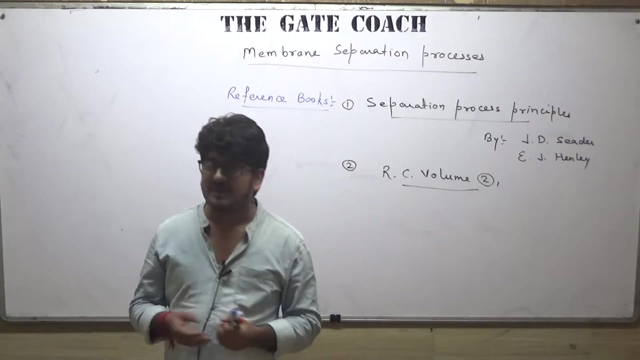 in your BTech as well. 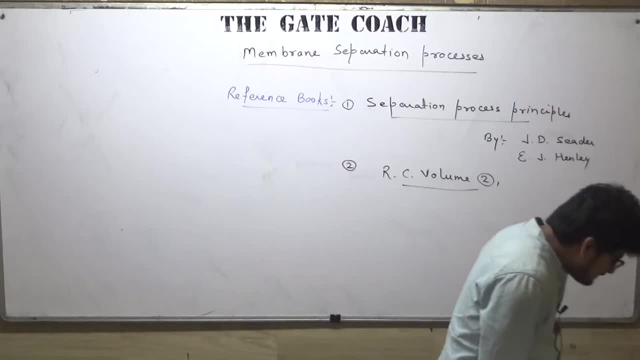 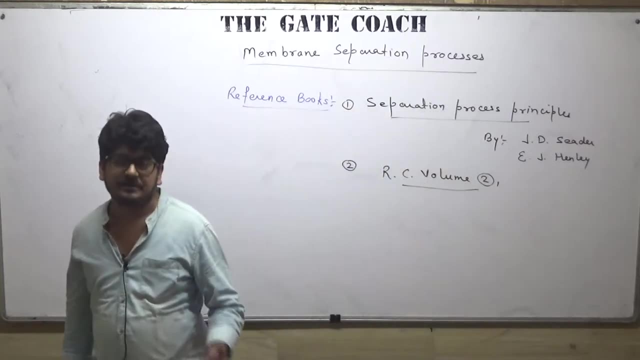 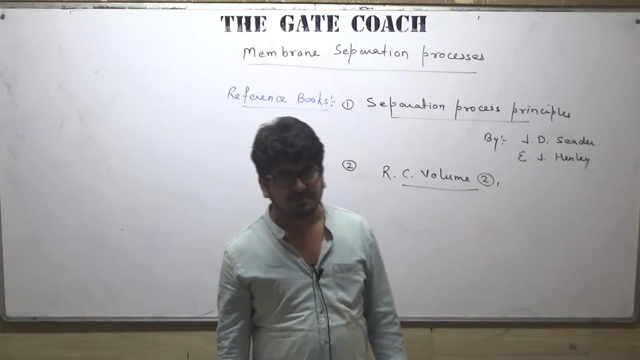 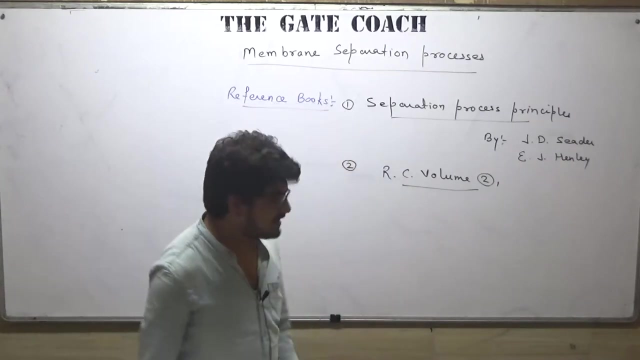 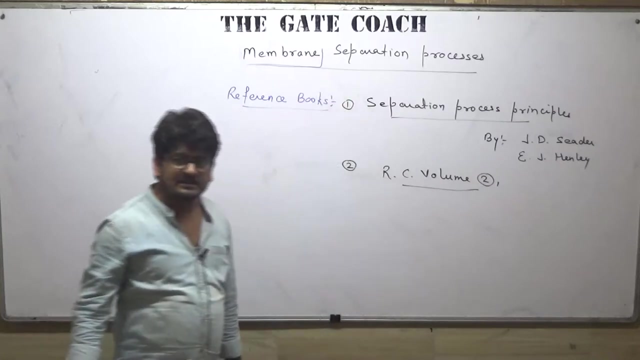 My part was membrane separation and CRE- okay, so let's go with this. So, guys, first thing first let's start. Okay, We have to study the membrane separation, So Let's go with the flow. The first thing is membrane. What is membrane? that we will discuss. 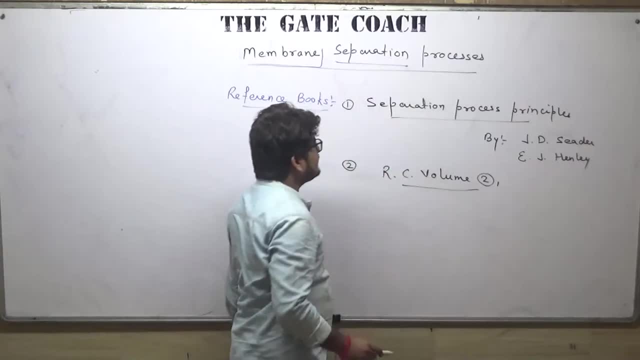 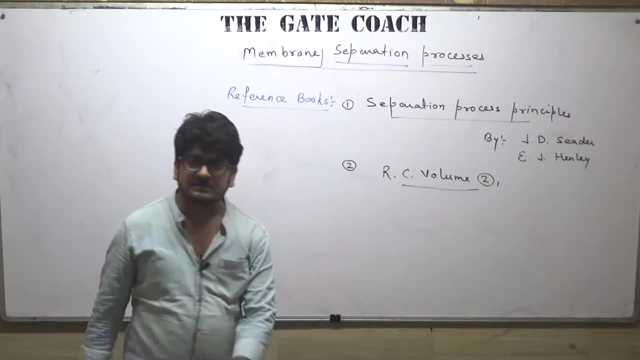 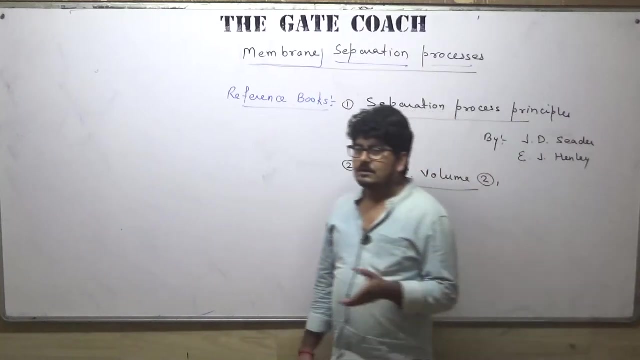 Wait for that. Second thing is separation and third is process- this term, Okay, so let's go by Each of this term, because what is my method? I believe that when you are preparing for any competitive exam, So you should be better than everyone else, So we should prepare like this: that 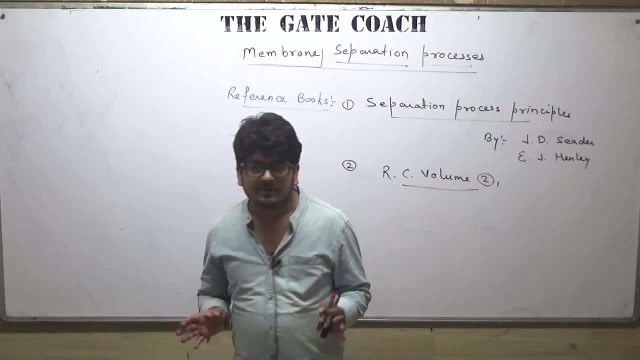 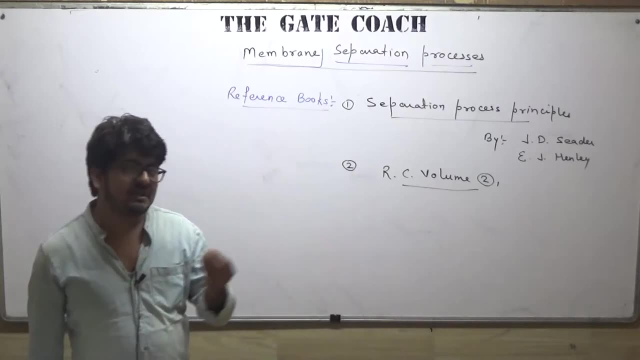 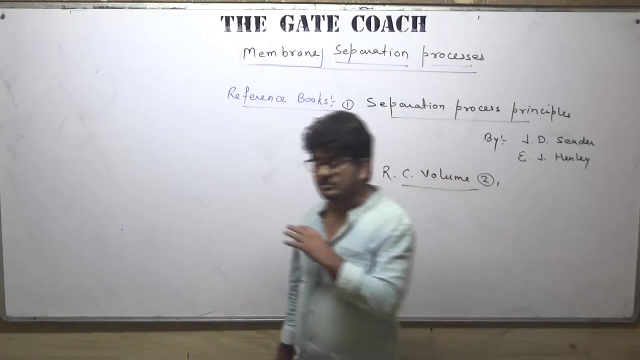 We can do all the questions, we can solve all the problems. Okay, So for me, I think if we study the meaning of each and every term, We understand the meaning of each and every term, Then we can do any kind of numerical, we can solve any kind of question. 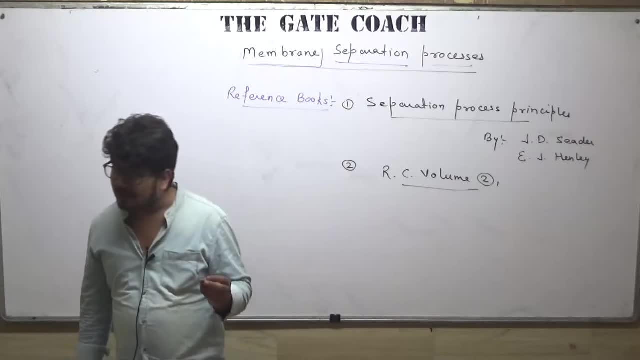 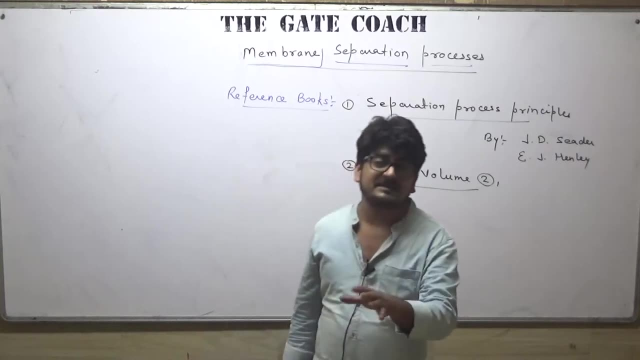 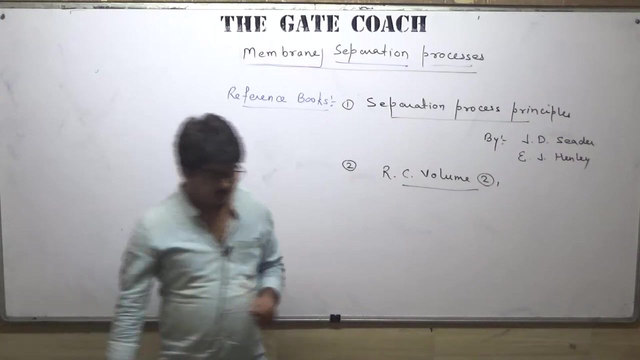 Okay, And when you know the meaning of each and every term in chemical engineering, Then obviously it will be helpful for you as well to while solving the questions of a multiple selective, Multiple select questions which have been introduced in gate 2021, first time, for the first time, Okay. 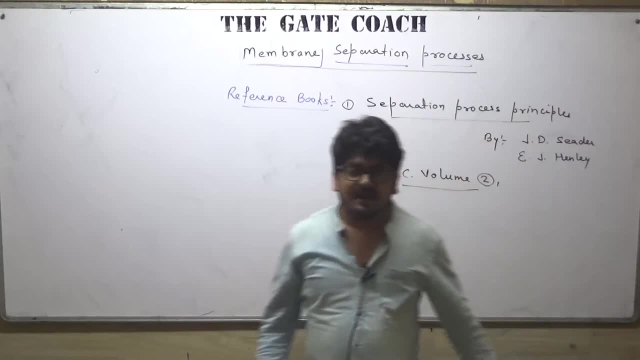 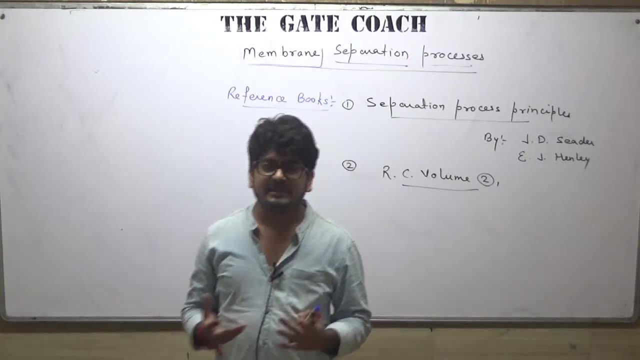 So let's talk about the process. Okay, and as all of you are there, Almost 70 plus students are right now we have, so let's make it our Interactive class interactive session. Okay, because I Don't believe in to complete the syllabus forcefully, So let's make it an interactive session. So 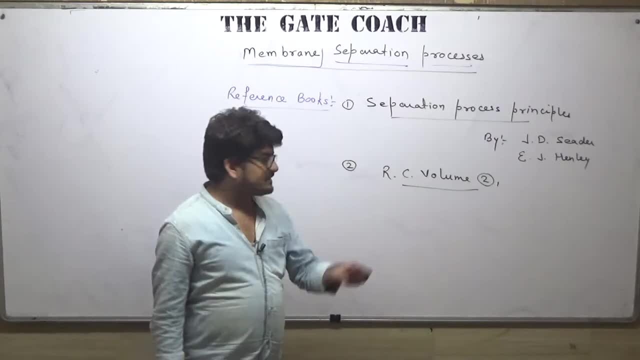 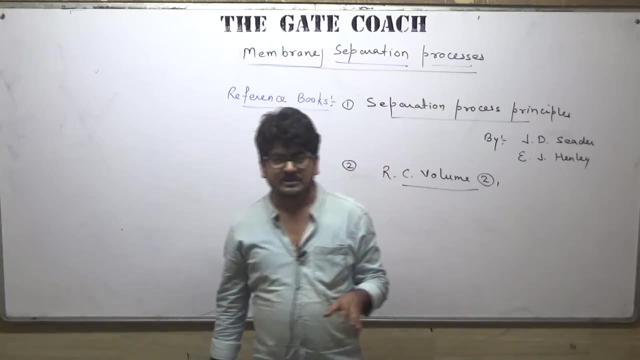 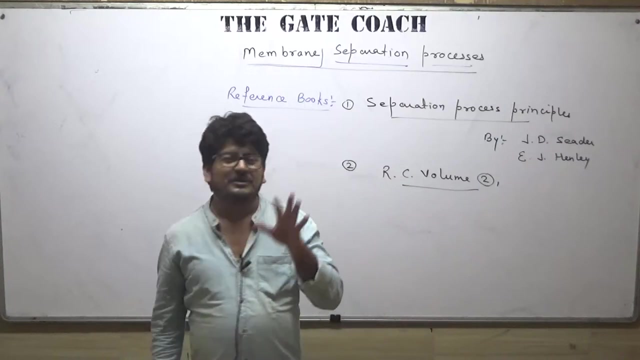 Can someone of you. I will discuss some points and I will ask some of the points from you guys so you can use this live chat option to answer Those points. okay, And I know you will not face any problem by in using this live chat, because most of you have have been become. 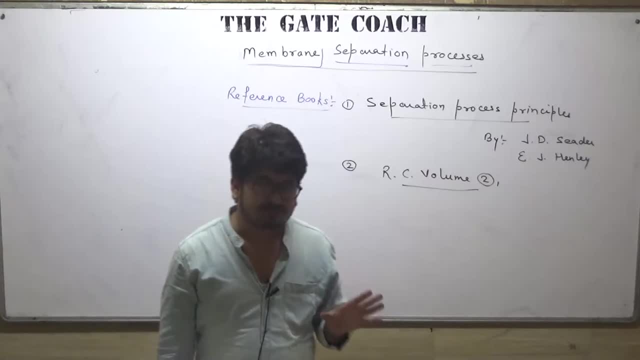 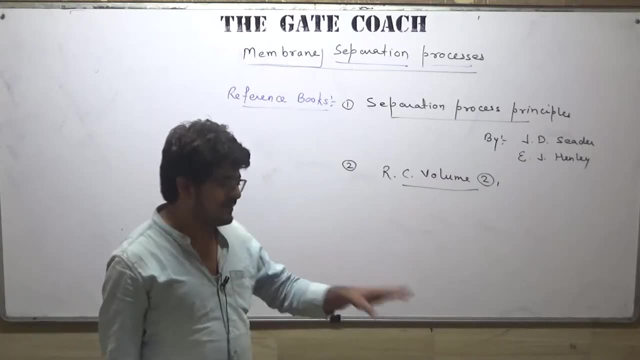 Expert in chatting, at least in this lockdown, Which will also palliative each adding my expert, the Facebook. what's up by Instagram? fit this? no, multiple logos have to check out the day, But you have to be able to make this a checker me, Okay. so I know I have a problem. They need to hear so, guys. 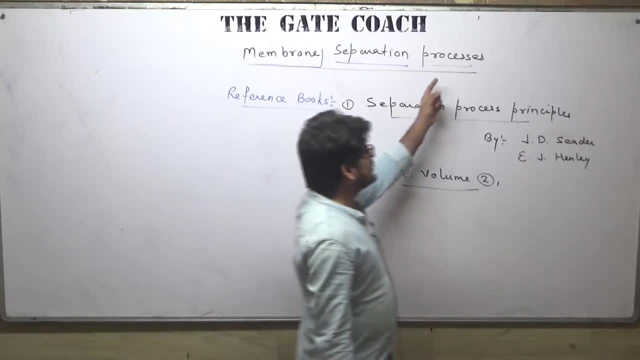 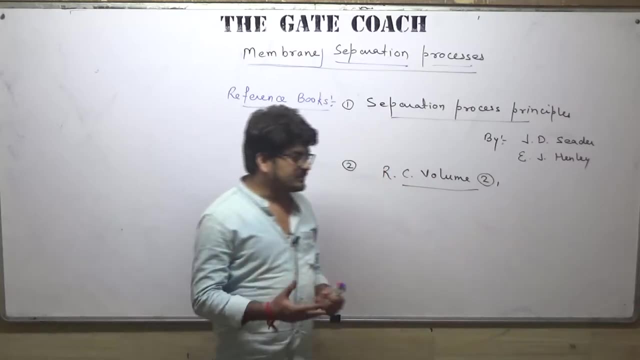 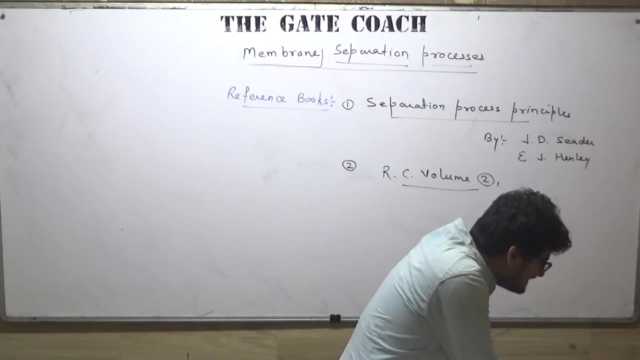 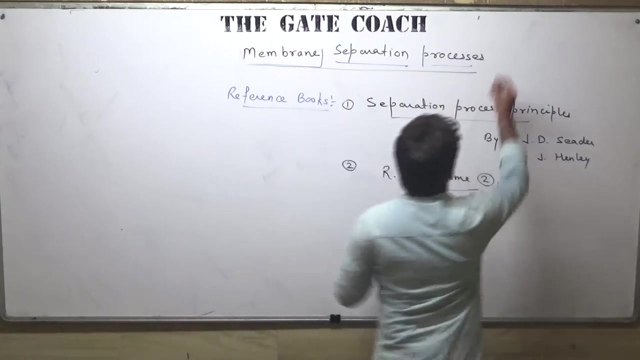 Tell me. what do you understand by this term process? Okay, So try, come up for a job. the answer, Karo, so that we can use this time. Kunal Sona. yes, this is chemical engineering part, Kunal, And if you are appearing for the gate exam in food technology or in any other, 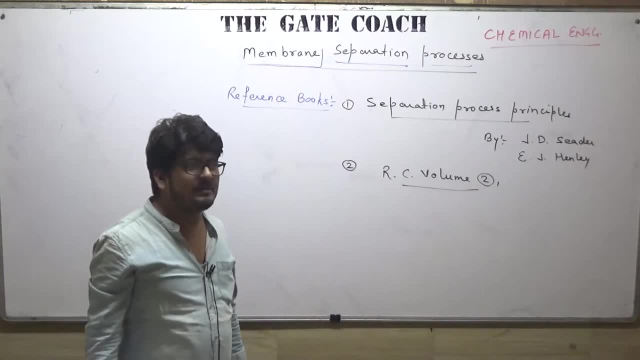 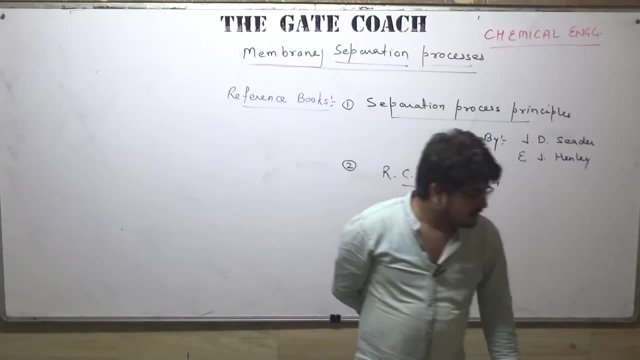 Subject: I don't know about all the papers, but in food technology as well. I don't know about all the papers, but in food technology as well, This part is there in gate exam. Okay, So, guys, tell me, what do you understand by the storm process? 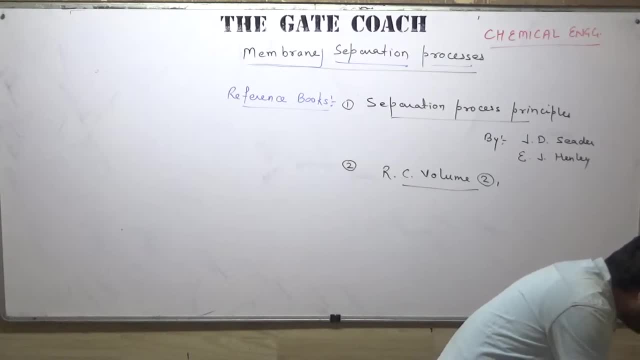 Process equal to no change in chemistry. not lazy, nice name, bro. We should not be lazy in our life. Good point armpit. anything which is used to convert one thing into another is called process. series of action of to achieve a desired state, some reaction happening, that is. 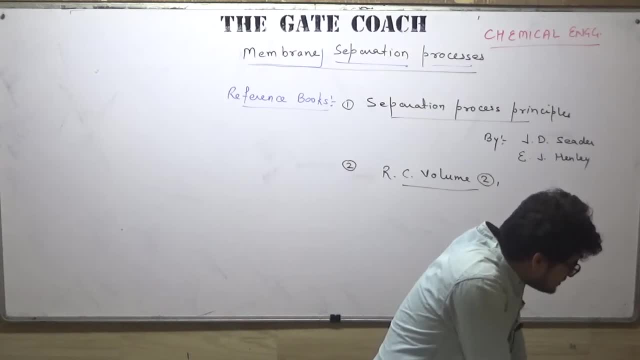 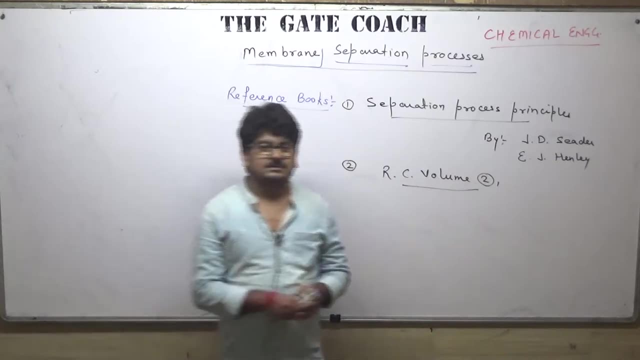 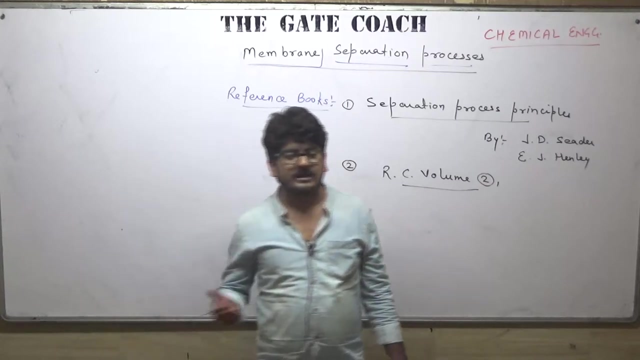 Method processes to get products from the feed reactions. see, as You are saying, it is correct. but Now we are not in college and I don't know about you guys. you have completed your beta for you are appearing for that, appearing in your final year, i don't know. but now, after the gate exam, when we will have a good score, 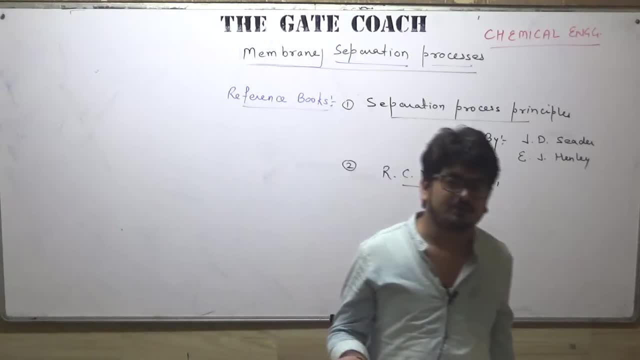 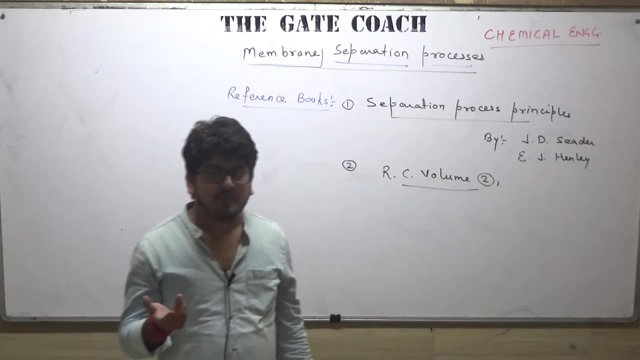 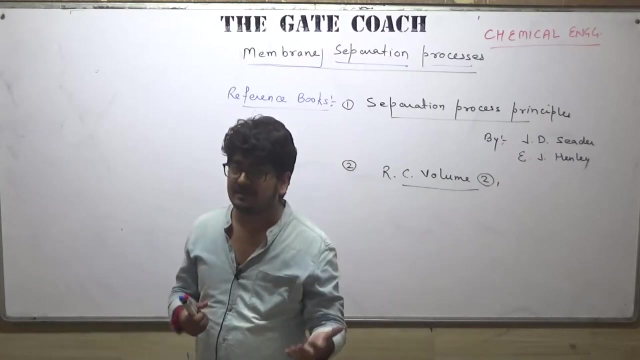 or even without the gate exam, you will go in for the job interviews or for the master or any interview. you have to represent your answer in a decorative manner, okay, in such a way that it should like that- yes, this is the one i was finding interviewer, think should think like that. this is. 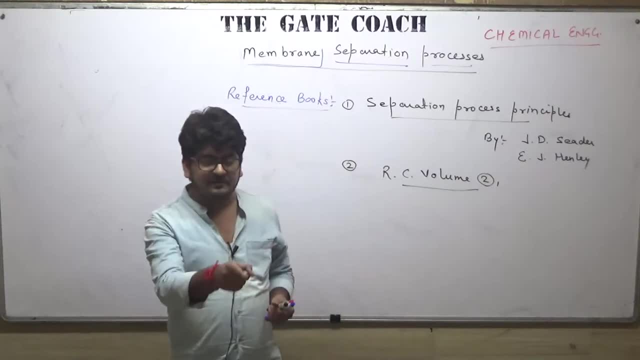 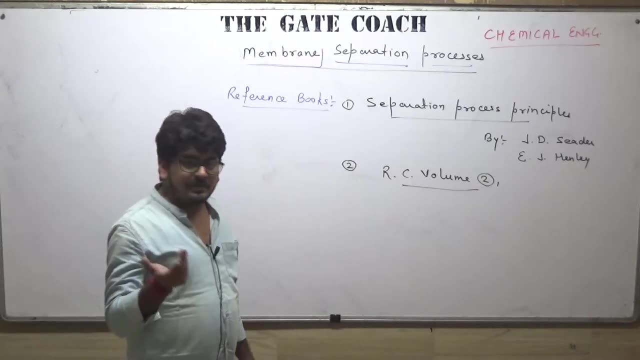 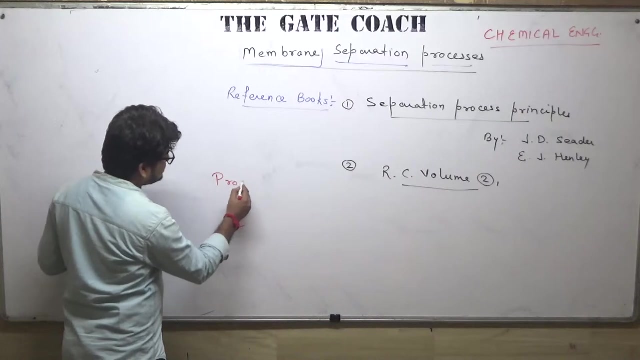 the guy we need in a for our company, or this is the guy we need for our research in an iit. okay, so always represent your answer in a proper manner. so you have mentioned your answer. that is absolutely correct. so let's see what we can say about the process. process is: 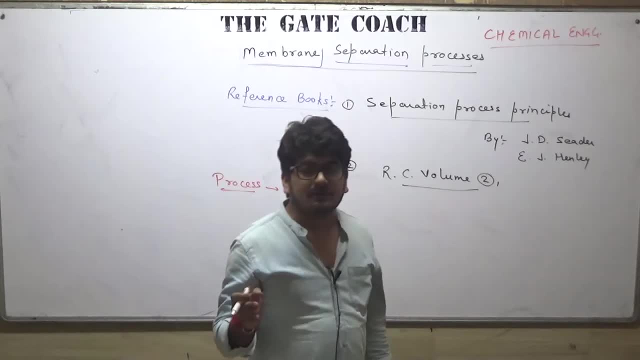 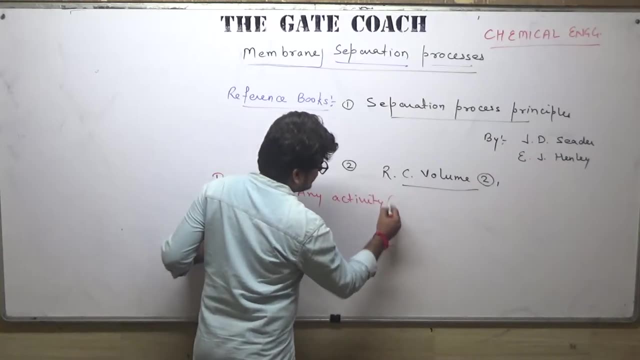 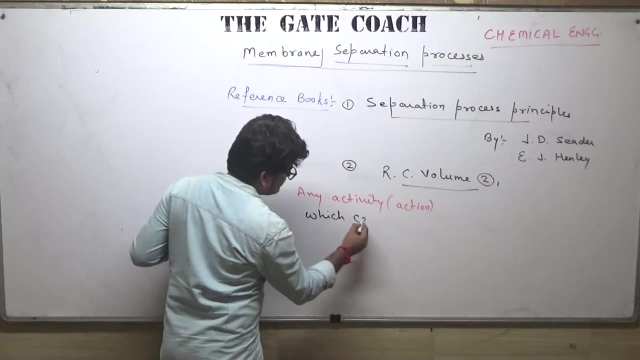 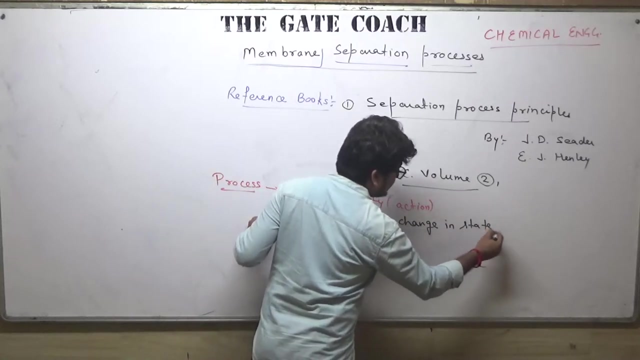 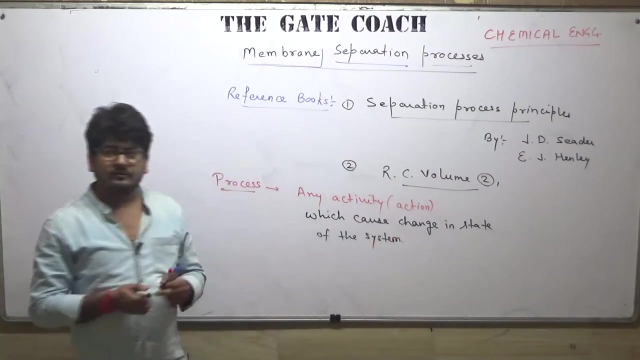 any activity, any action which causes any activity. or you can say action, any activity. or you can say action, any activity. or you can say action which causes change in state. change in state of what? change in state of the system. okay, i hope all of you know that every system has a state. thermodynamic state means the 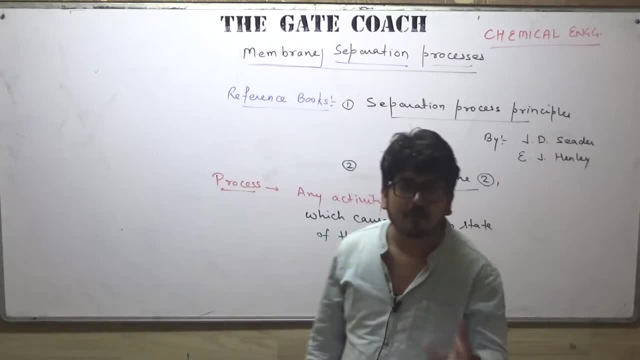 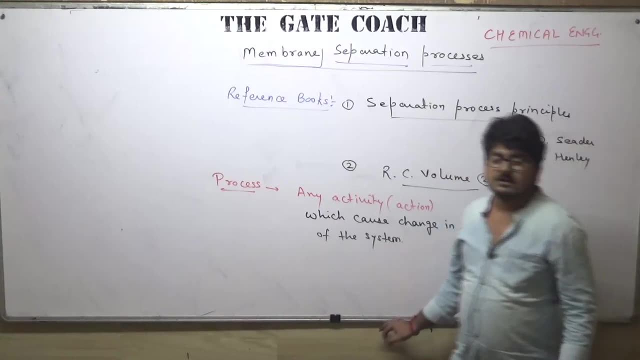 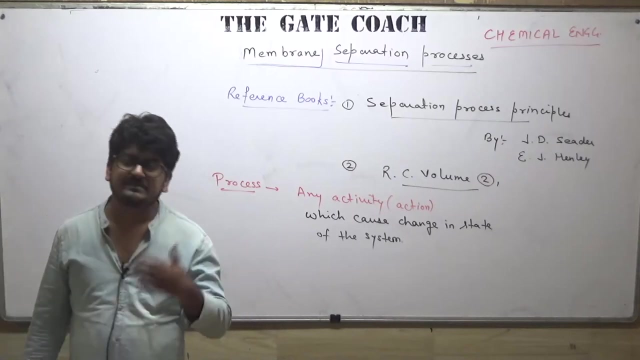 characteristics of the system at any given time. okay means the properties of the system, basically. so any action by which the properties, the characteristics, the state of the system is changing, that is called process and depending on the change in characteristics, we can classify the process like chemical processes, mechanical processes, physical processes and all those things. 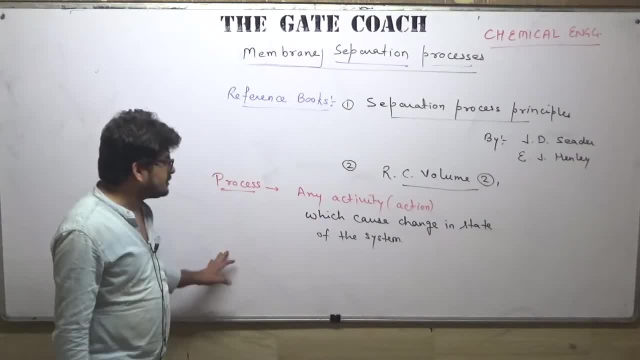 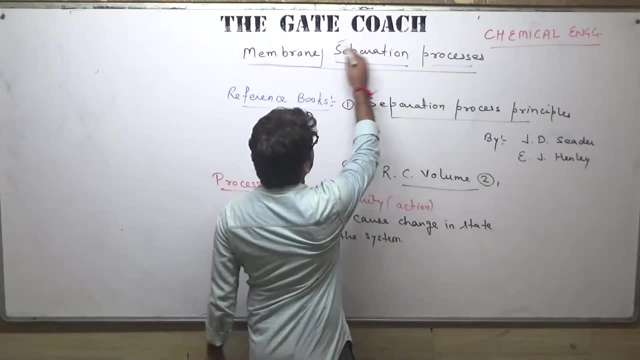 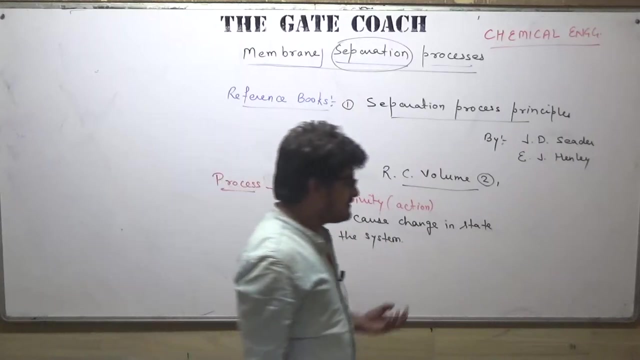 okay, we will not go in all that much detail because i assume you know all of those things. in case you don't know, then you can discuss that after the class. next part is guys- separation. next part is guys separation. next part is guys separation. okay, so what do you understand by this term separation? 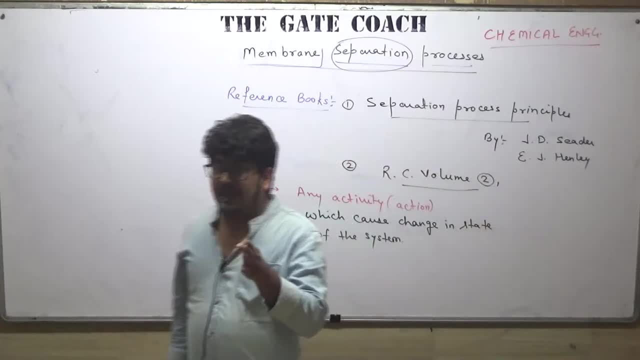 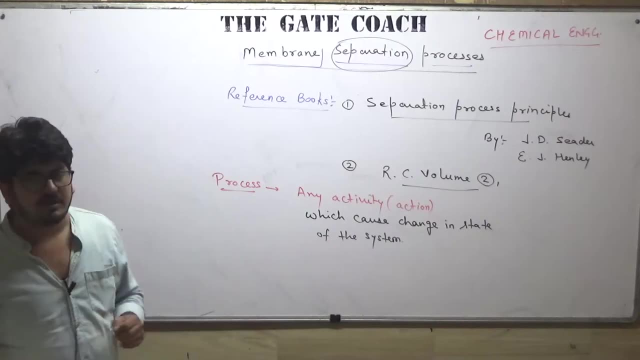 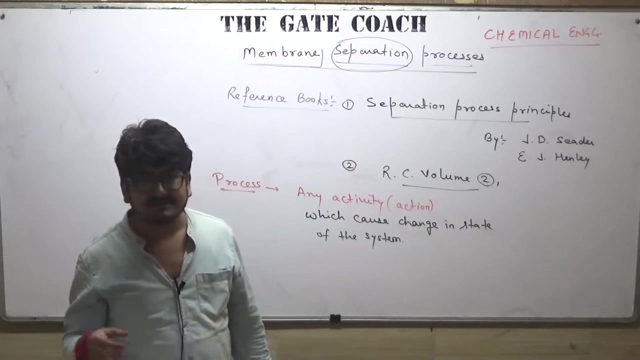 cause chemical change. if the action is causing chemical change, that will be a chemical process. if the action is causing chemical change, that will be a chemical process, basically chemical reaction. okay, if the action causes changing mechanical sector characteristics like shape, size etc, properties, all those things, then that doesn't mean that makes any difference. 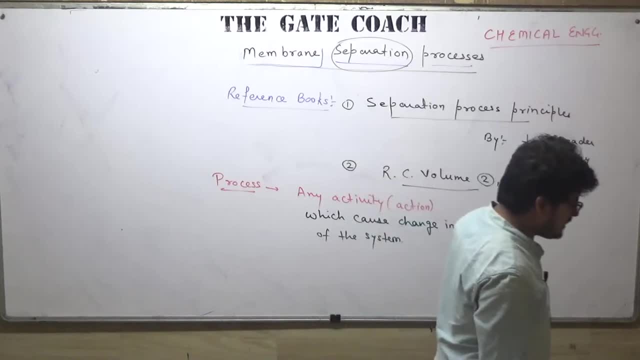 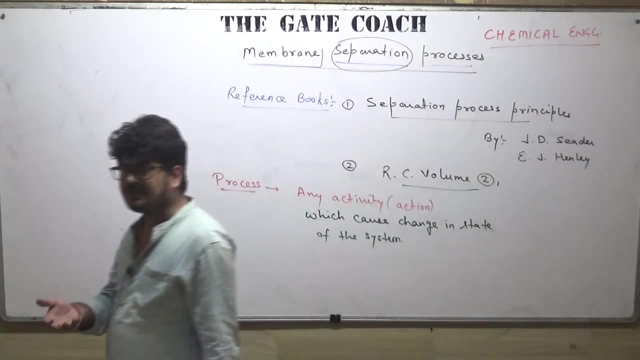 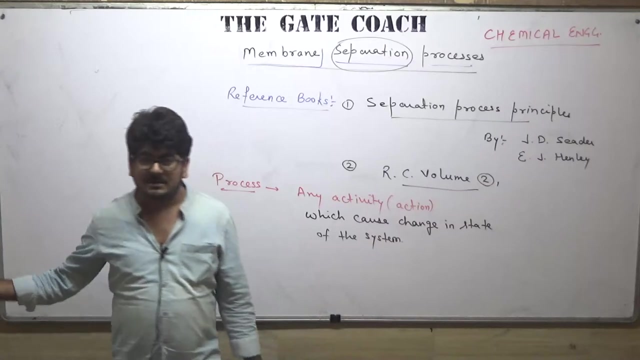 then that is mechanical action, mechanical process. And if only the physical characteristics are changing, like composition, temperature, pressure, all those things, then we will say it could be a physical process. Based on that, our chemical engineering have been divided into several parts like mass. 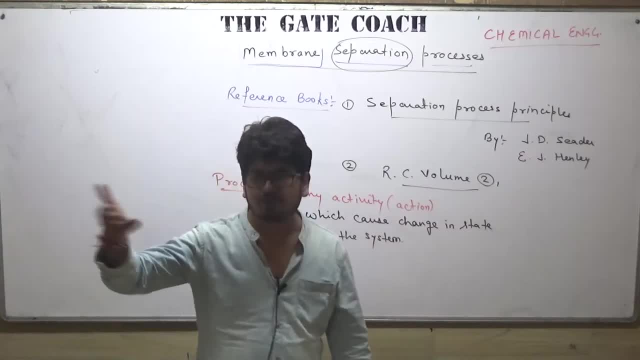 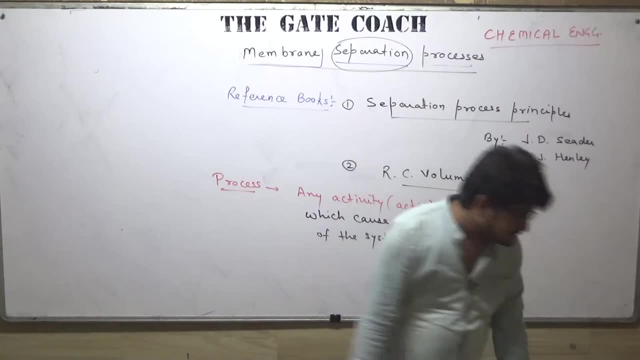 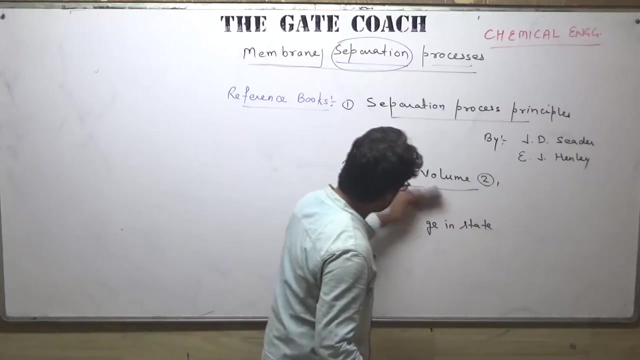 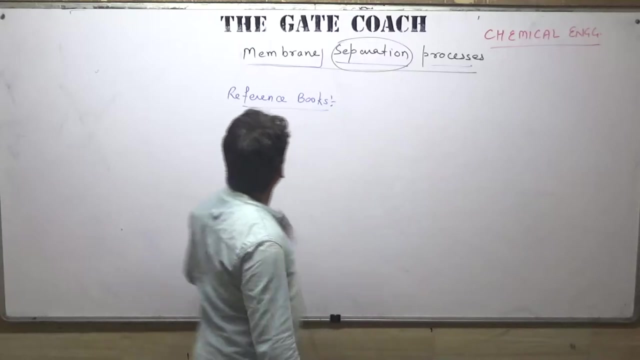 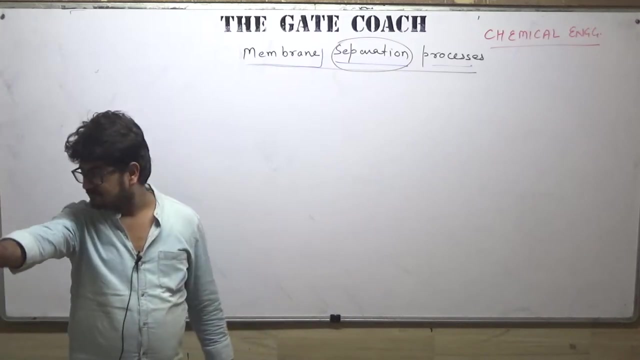 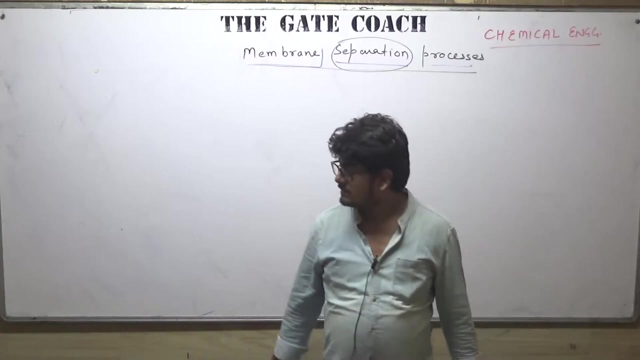 transfer, heat transfer, unit operations, unit processes, all those things. you know all that stuff. So, guys, what is separation for you? What is separation? Tell me, What do you understand by this term? separation, Light on. I think now it's fine. 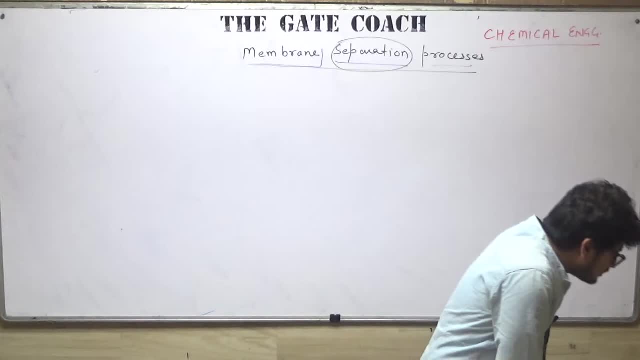 It's better. Thank you, So, guys. separation is: can we see video tomorrow? Cause: chemical grouping on the basis of particular properties. Removal of one thing from group of things- Okay. Aggregating based on some unique qualities. Differentiating substance on different properties. 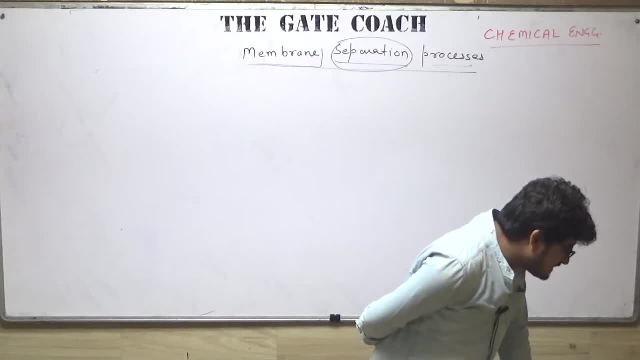 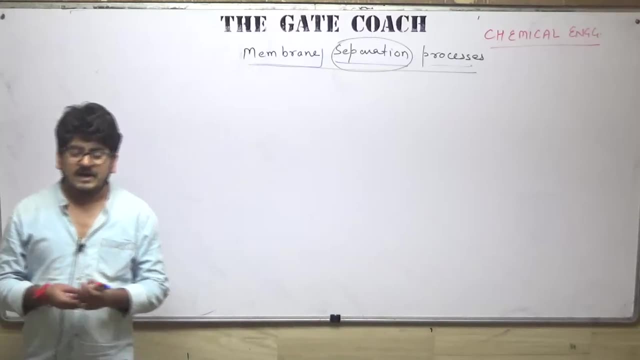 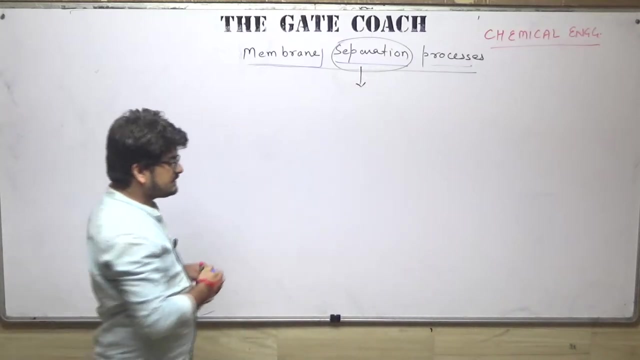 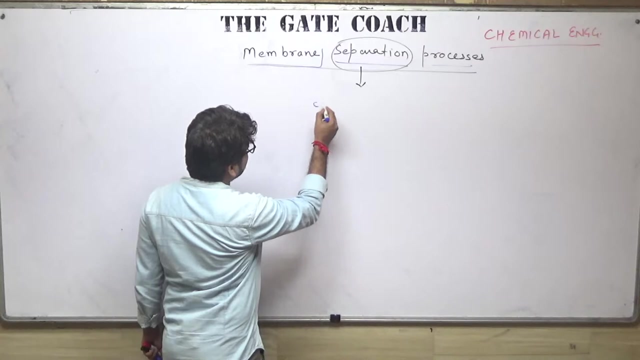 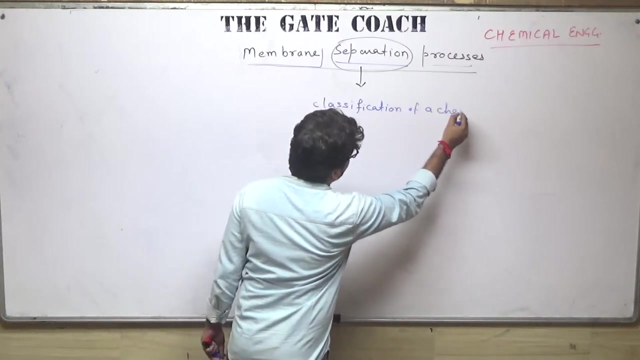 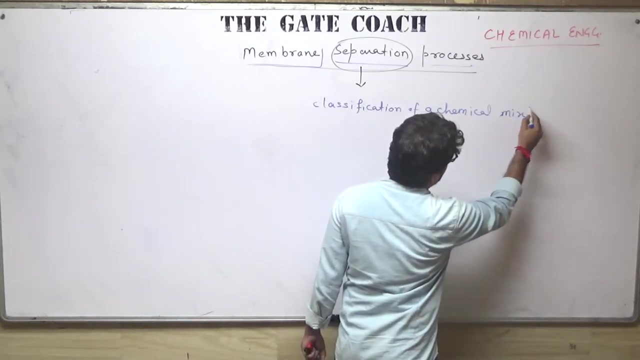 Okay, Different basis: Remove desirable substance from undesirable. Yes, Basically, to remove, to divide something and what we are dividing, Okay. So separation we can say as you can say: break or dividing, or you can say the classification of a chemical mixture or a composite system or a composite mixture or compound into its. 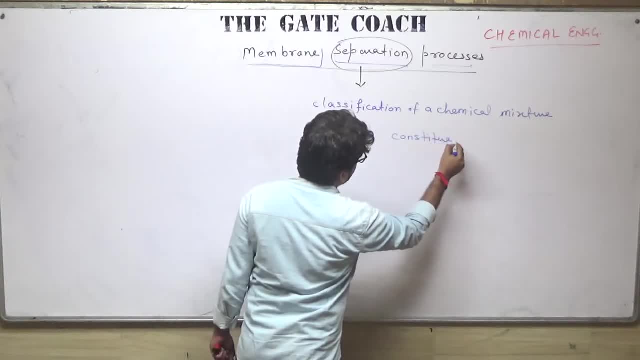 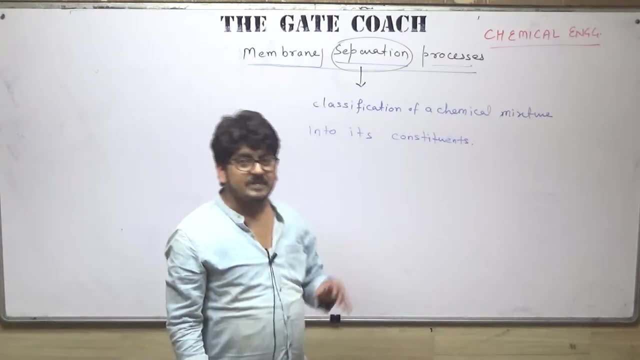 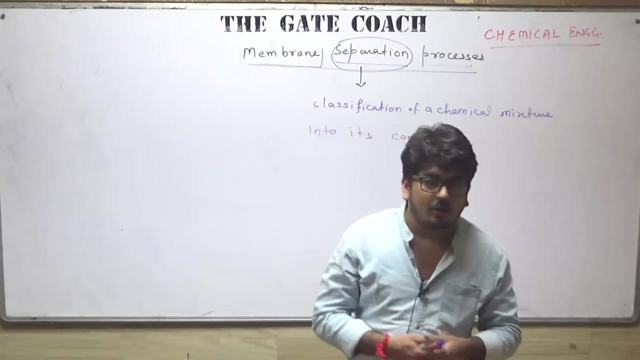 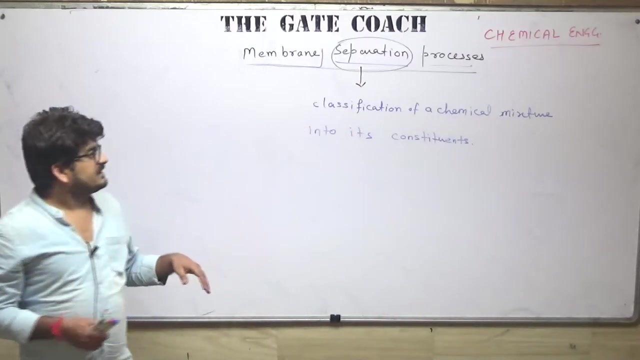 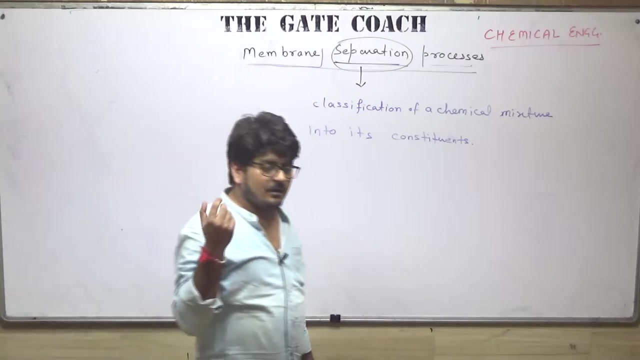 constituents, Okay, Classification of a chemical mixture into its constituents Means. That is what we call separation. Okay, guys, And for that separation, if I talk so, separation is a very old process and that is one of the most important process in our industry. 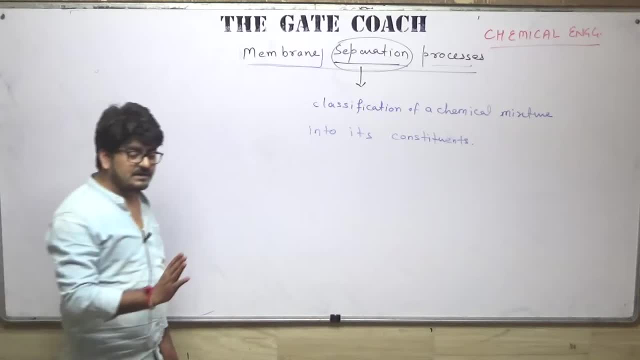 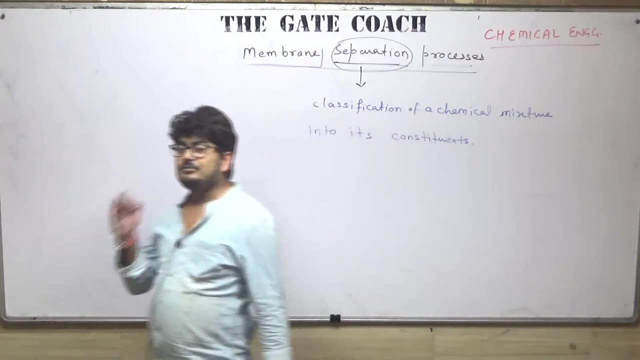 Okay, As a chemical engineer, if you remain in the core technical line, then ultimately we you have to go in the industries. obviously Okay, And in any industry, the main process is always the separation which always decide the cost of the process, cost of the product you have. 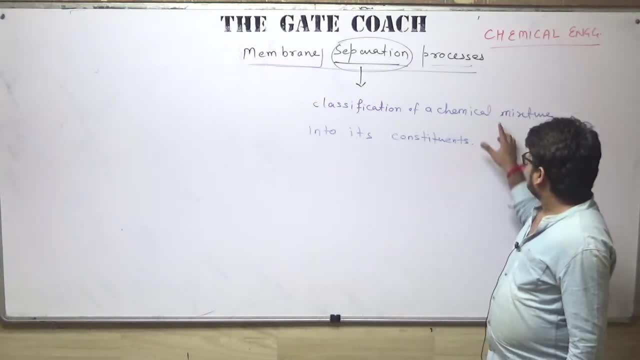 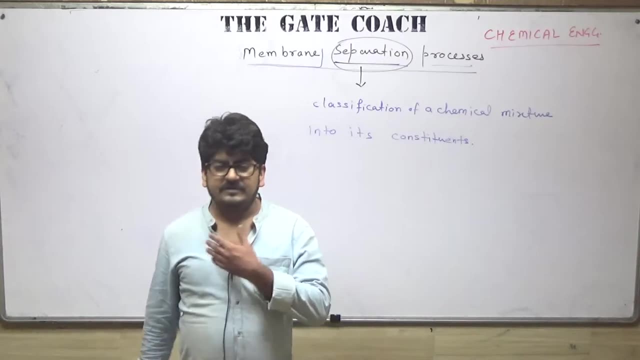 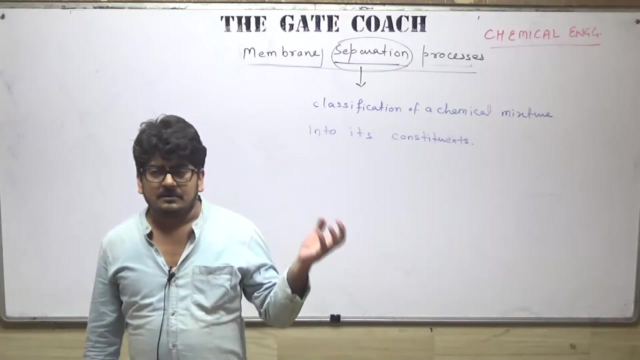 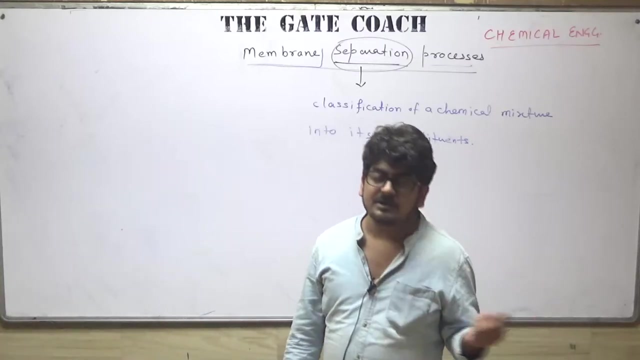 Okay. So here, if I talk about the separation processes, Okay, So we have so many examples which we are using from our ancient times. Okay, Like the manufacturing of perfumes from flowers. Okay, Salt from sea water. There are so many examples. 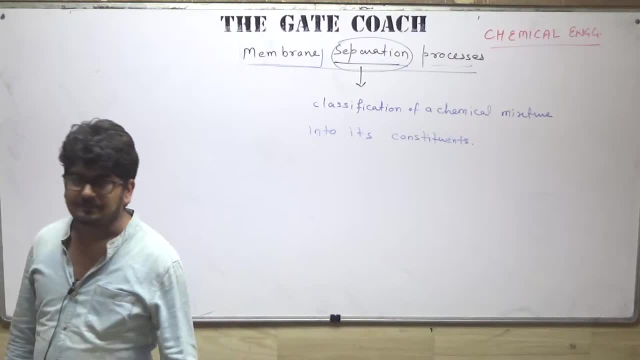 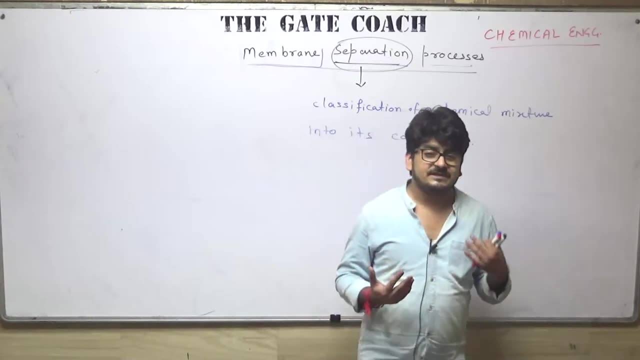 Metals from their ores. There are so many examples, are there? So? and if I talk about our human body, then in our human body as well, there are so many processes going on inside the body. Okay, And if I take one example of the kidney, 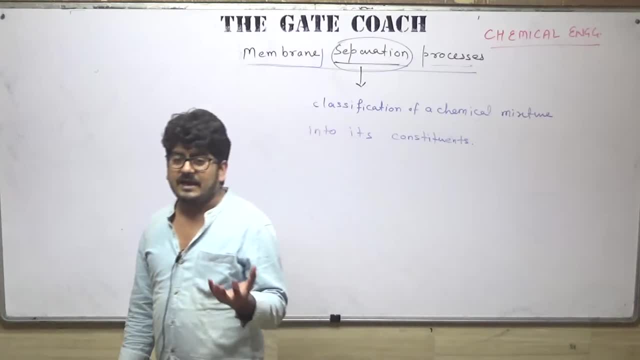 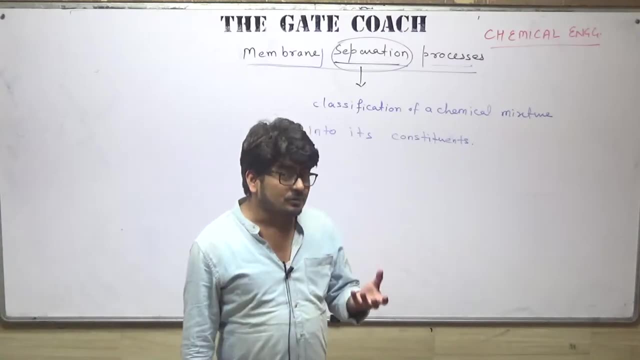 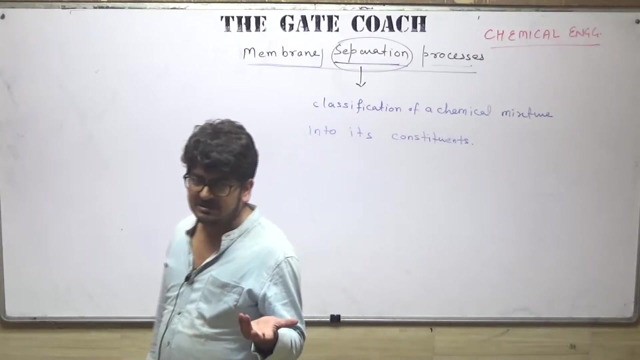 Okay, So kidney is also acting like a separation process. where what is happening? I hope all of you know that kidney is used. Kidney separates the water and the waste product which are produced because of metabolism from the blood, And so many things are there. 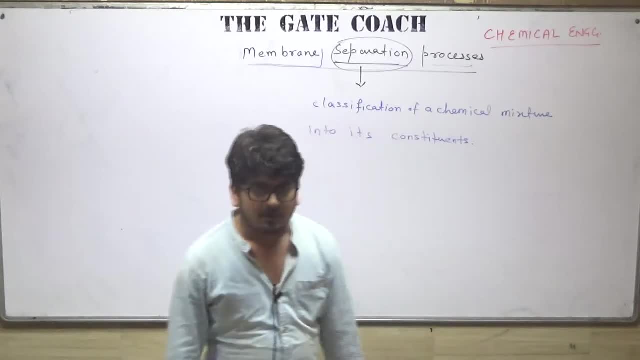 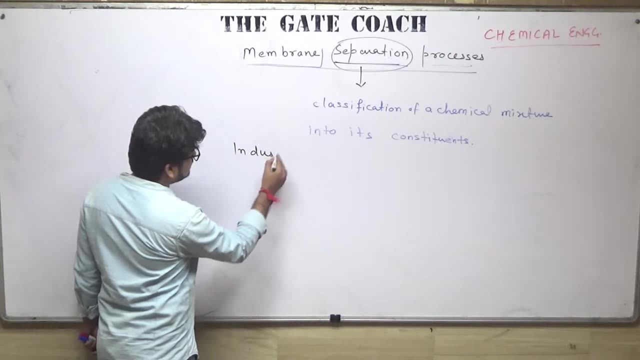 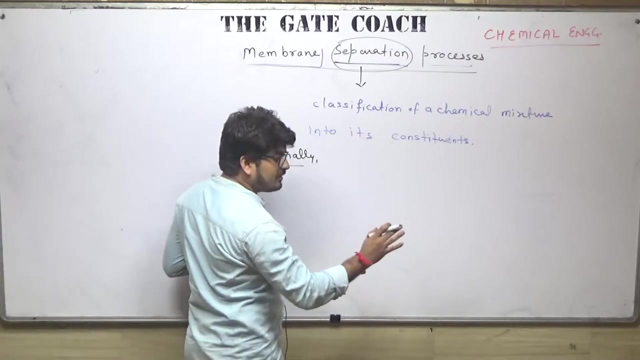 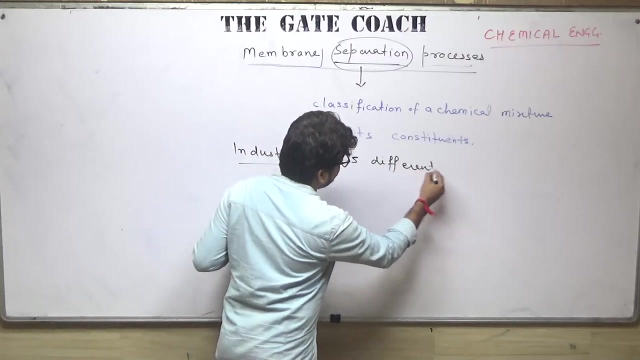 Okay, So these all things are separations. Okay, And on industrial basis, If I talk about the separation industrially, if I talk about the separation, then separation we can perform by five different methods. Okay, Five different methods we use to do the separation. 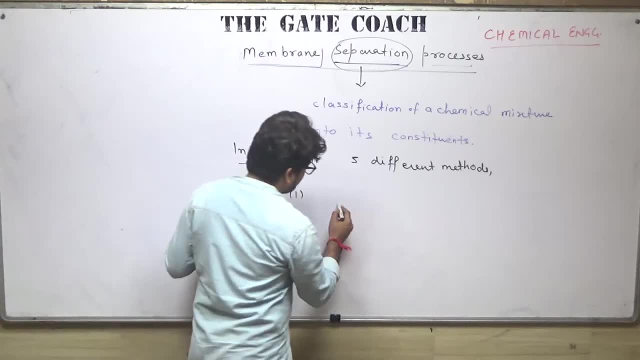 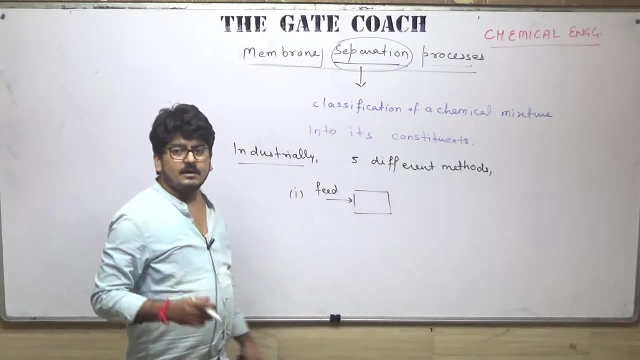 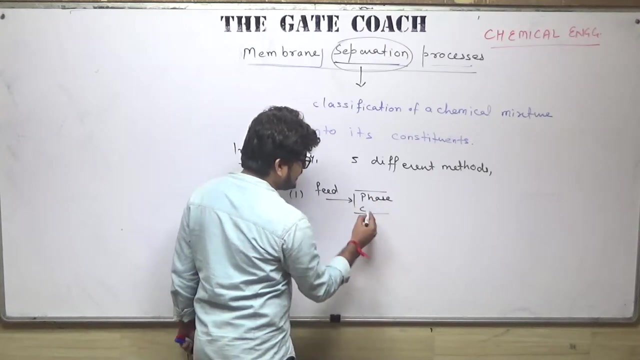 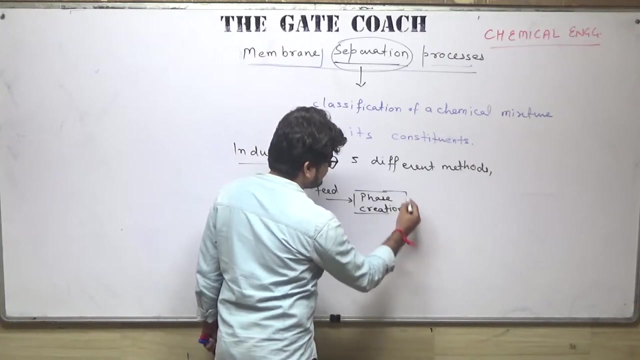 The first method is suppose this is the feed We are sending to a system. The first method is phase creation. Okay Means from the feed we are creating a new phase for the separation, where the feed further separates into two parts or more than two parts. 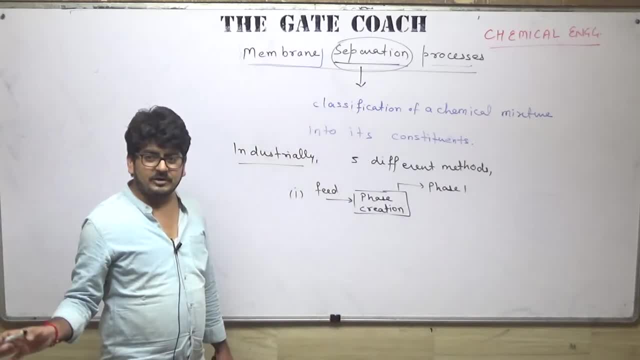 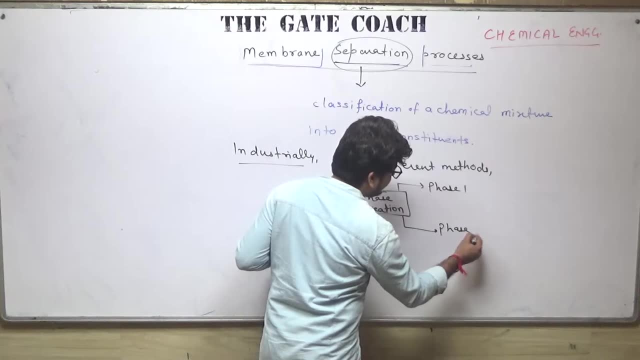 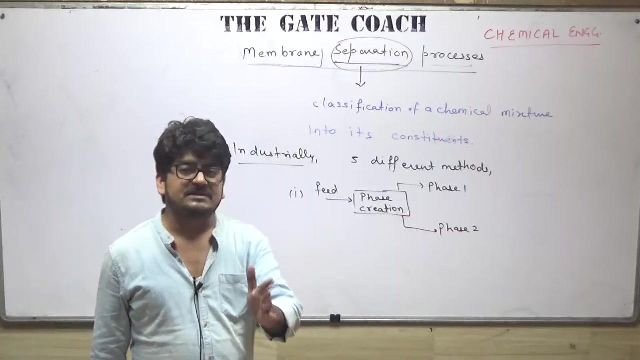 Obviously if separation is there, so at least product in the outlet we will get at least minimum of two streams. Okay, Let's say that is phase one and phase two, or stream one and stream two, Phase creation: Okay, Phase creation means we send the feed to the system and by the use of some heat or you. 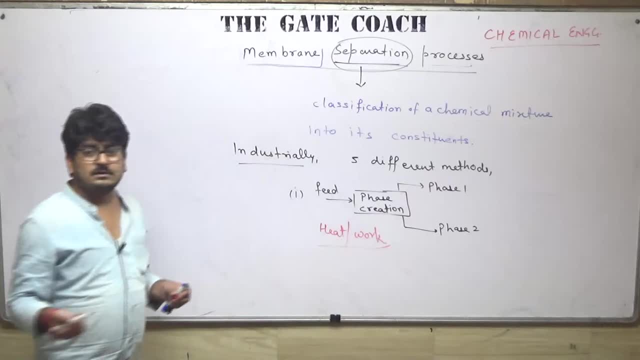 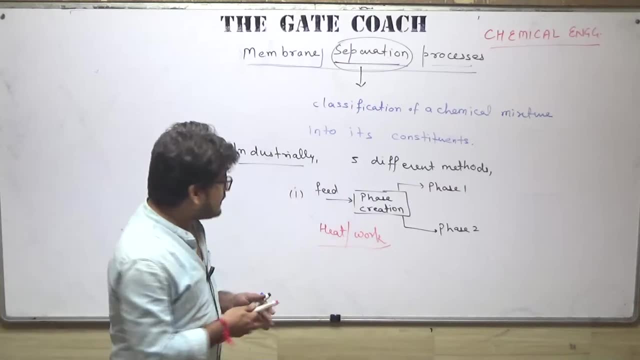 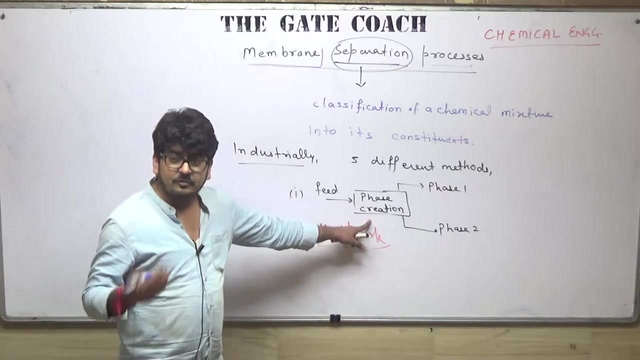 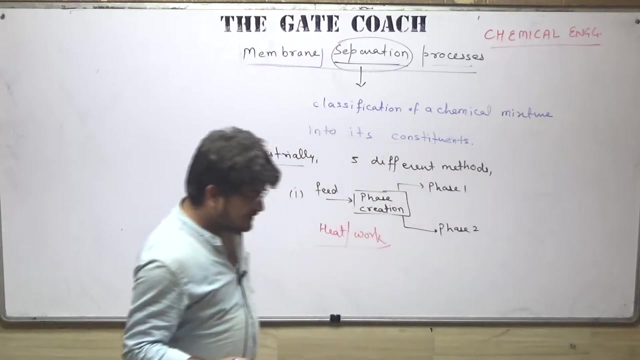 can say work or both. we create some phase. Okay, We create a new phase for the separation purpose. The example: can you tell me any example of this? It's very easy to understand Where we are creating the phase, a new phase, with the help of heat and work. 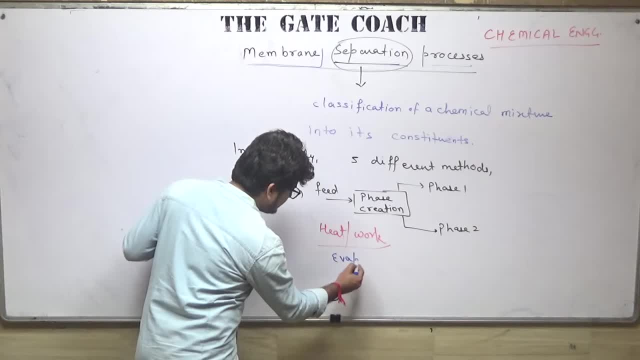 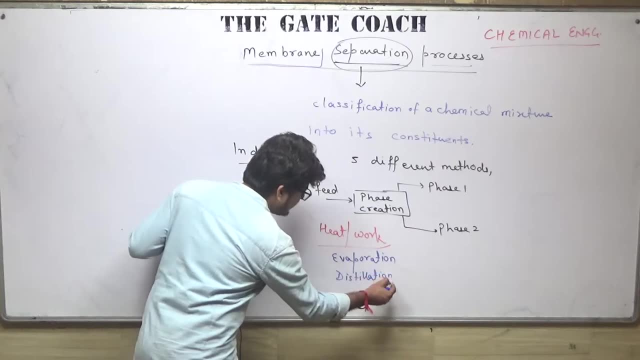 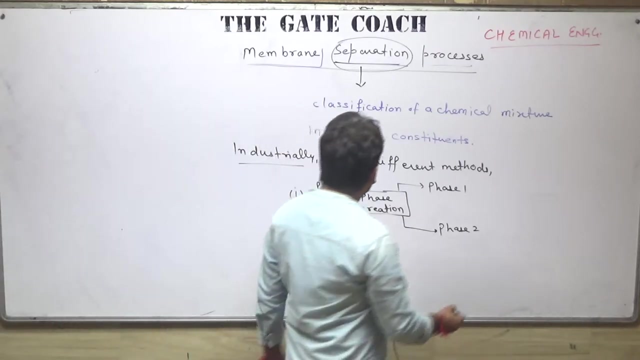 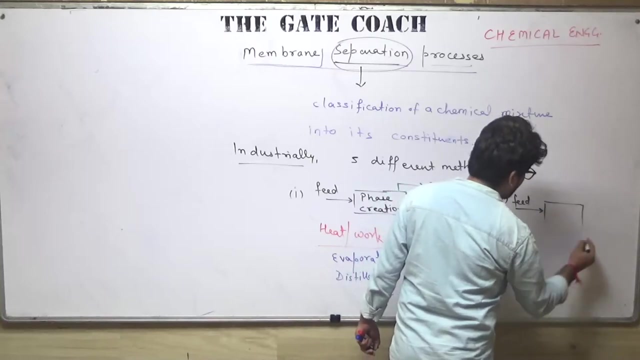 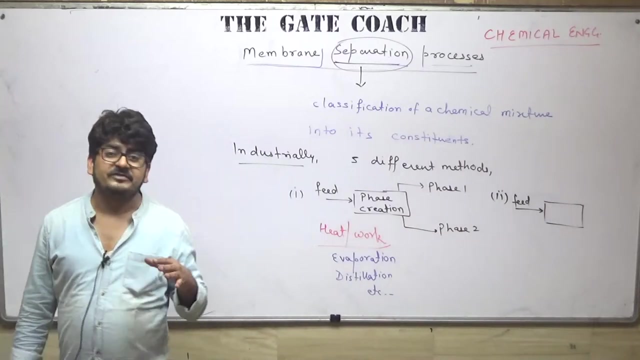 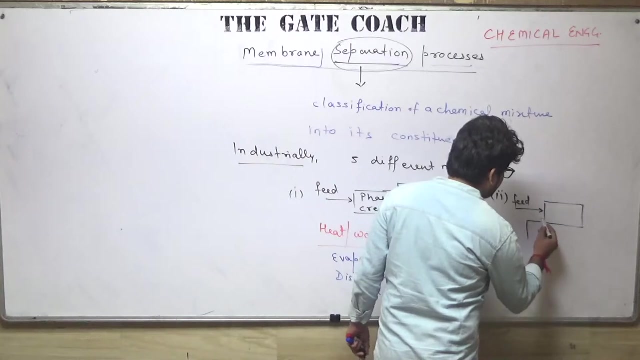 Distillation, Yes, Distillation, Evaporation. These are the examples where we create the new phase for the separation purpose. The second method is: suppose this is the feed we are sending Now. we don't want to create any phase. Instead of that, we are sending. a new phase means the phase addition. 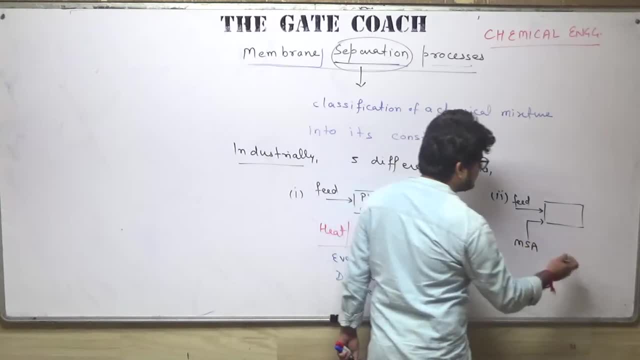 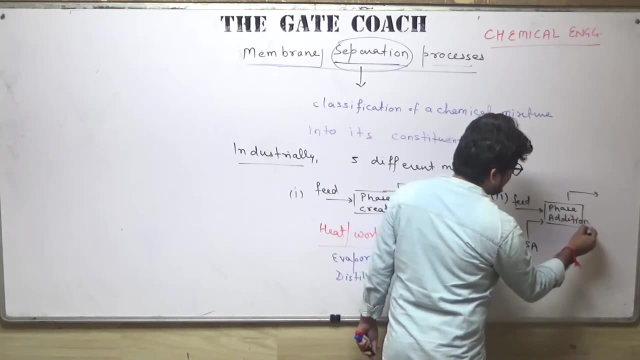 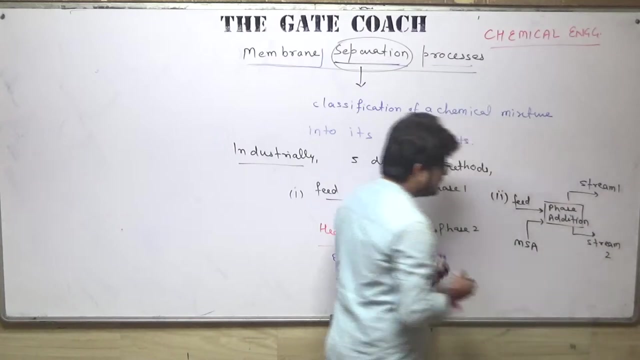 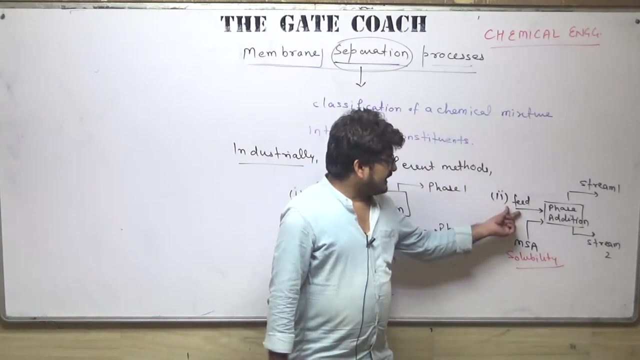 Okay, It means a new phase is introduced in the system And, based on that, separation takes place, Where we get stream one or you can say phase one or phase two. This method is like based on solubility. Okay, In the feed we have obviously many components. 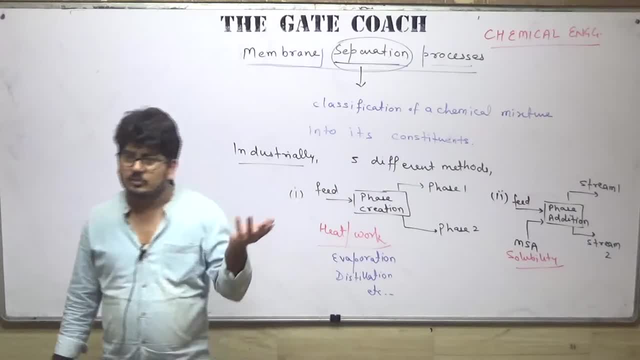 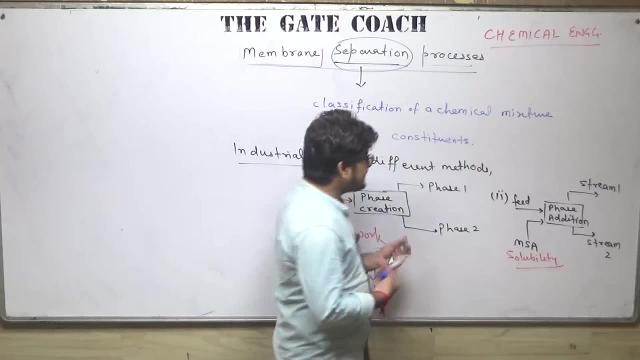 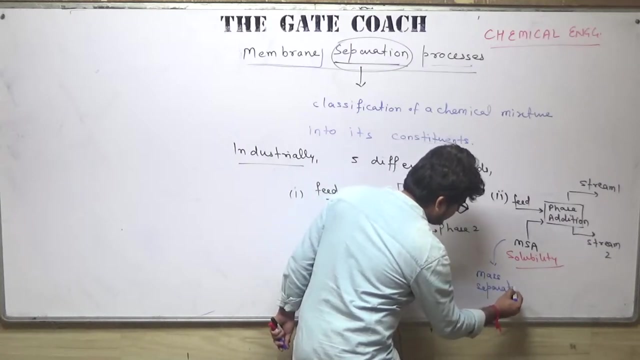 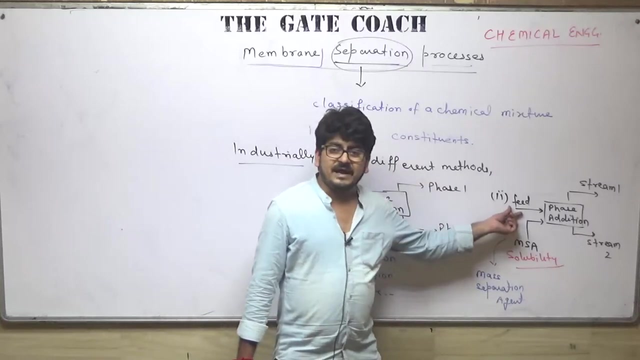 That's how we want to separate it. Many means two or more components, So we will use a substance, We will use a new phase, MSA. MSA basically stands for mass separation agent. Okay, Where the solubility of any of the component which exists in the feed. 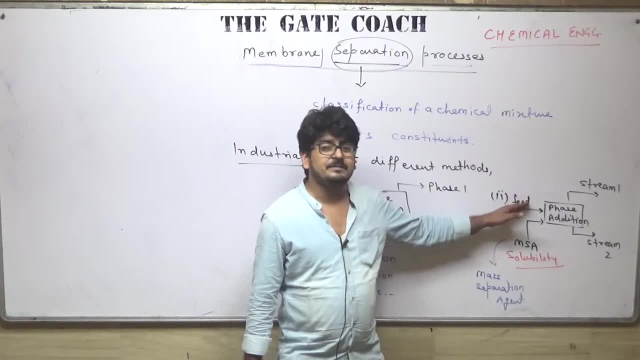 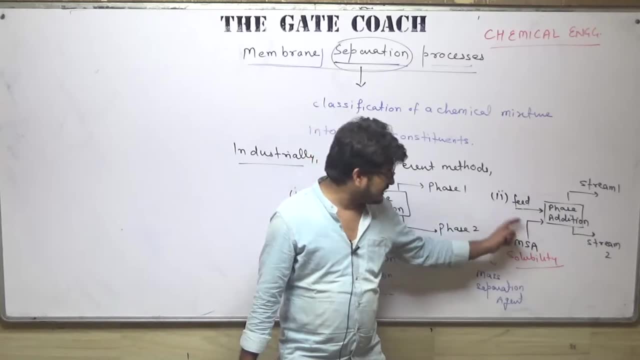 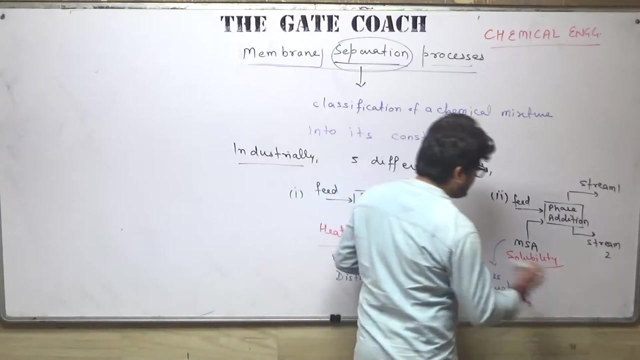 So solubility of any of the component will be high in this new phase. So the component will leave the feed and move into this mixture, Into the new solvent, And we will get the separation. Okay, That example I hope you can write. 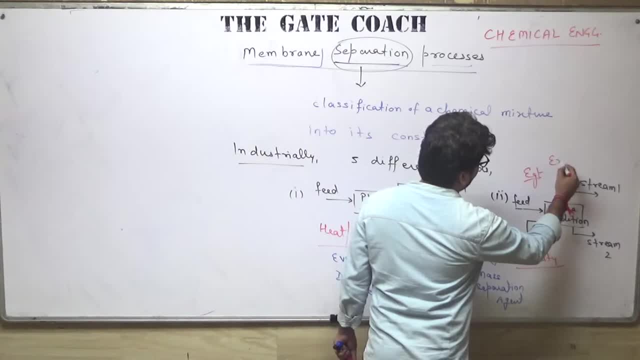 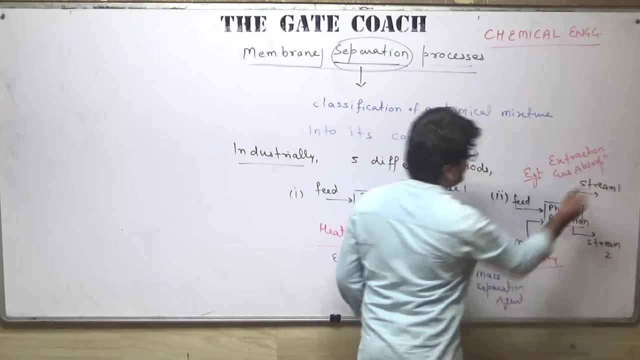 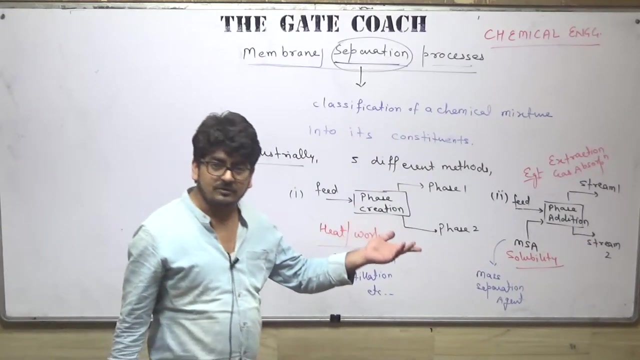 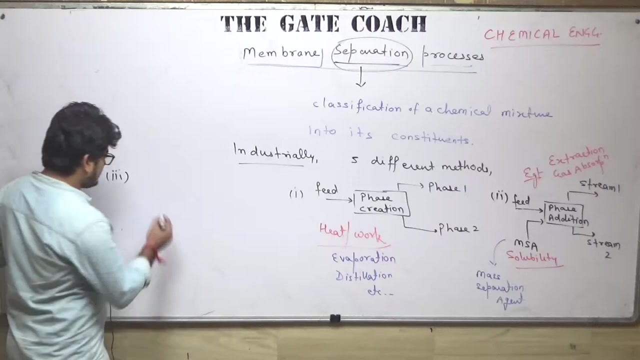 Example is extraction, Gas absorption, Etc. Okay, Like in extraction, in gas absorption we send the new phase. That is the solvent for the separation. The third part is: guys, When we use some barrier, Okay, This is the feed. 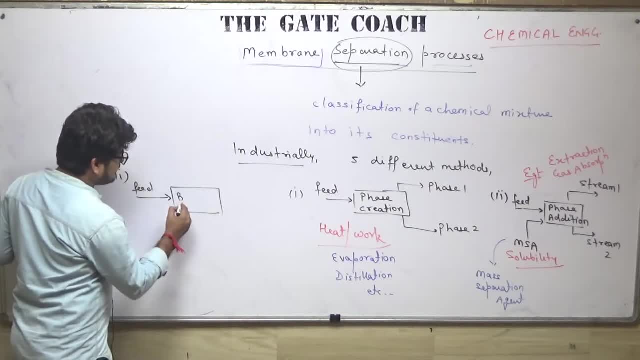 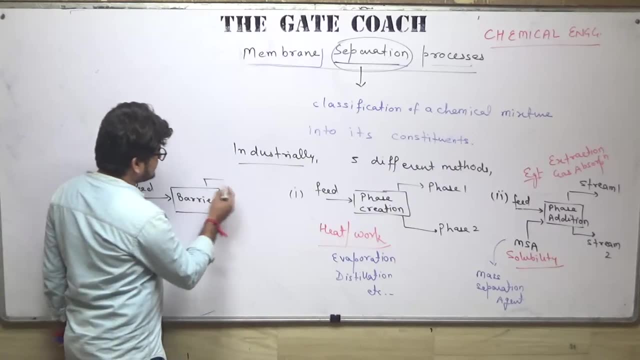 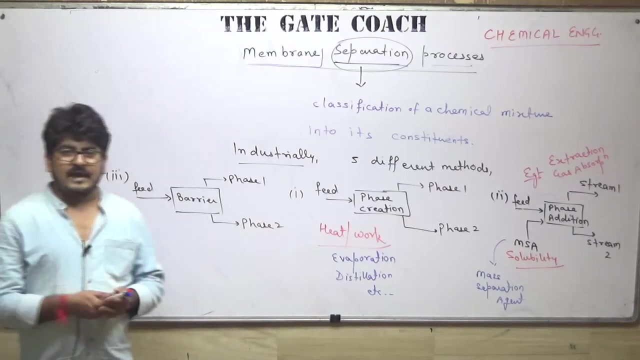 We send this feed in a system where some barrier is present And because of that barrier the feed separates into multiple parts. Okay, Like here we can say phase one and phase two. Examples are like barrier means when feed go through with the barrier. 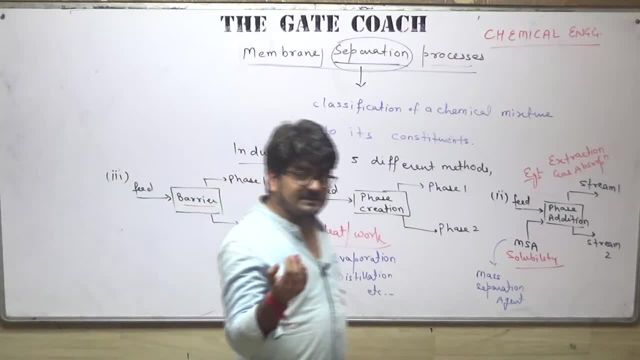 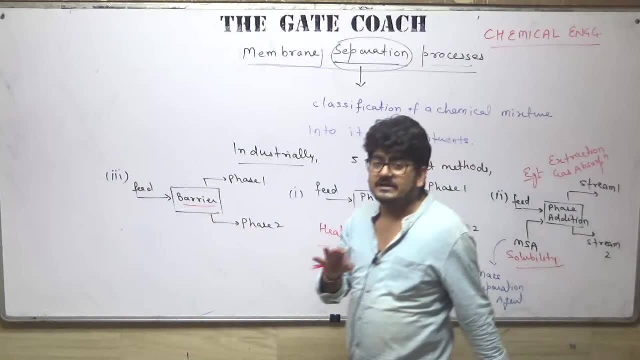 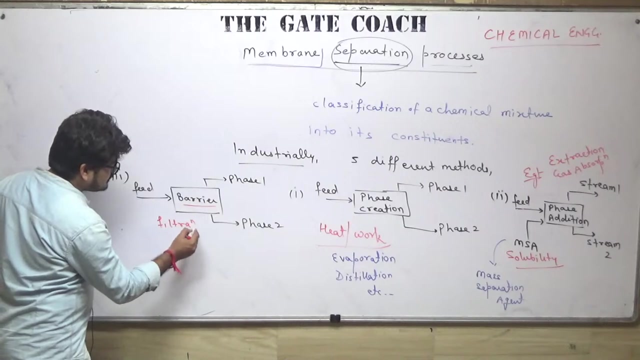 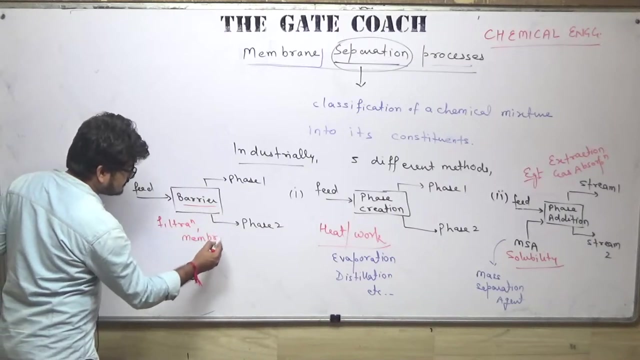 So the selective components from that feed will be allowed to pass through that barrier And the remaining components will retain over the barrier. Okay, The examples you want. you can write it as filtration. Okay, You can say membrane, separations, Etc. 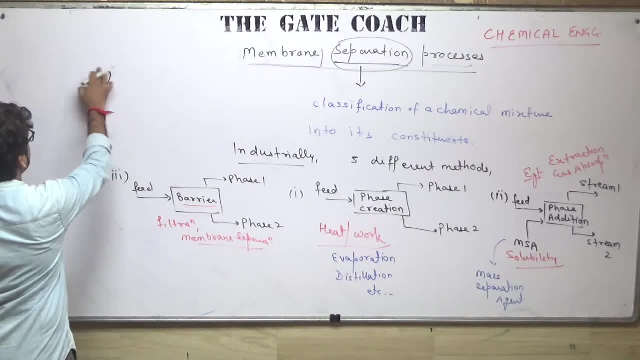 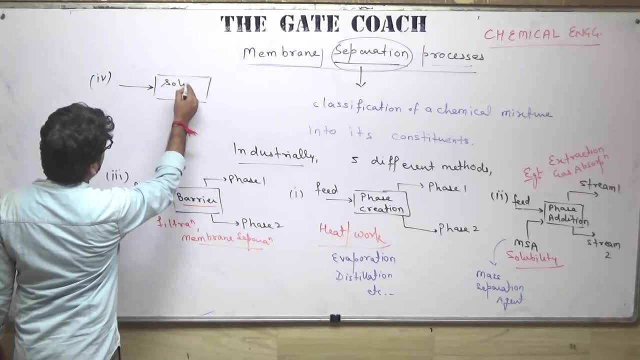 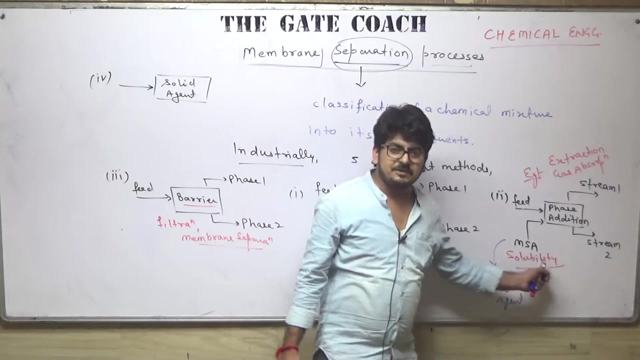 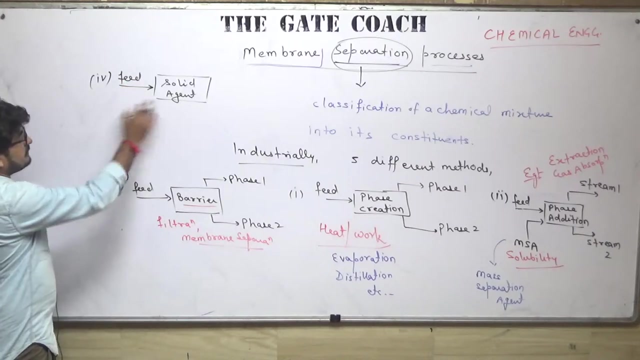 The fourth method is introduction of a new solid agent. Okay, Okay, Okay, Okay. Like here we were using some liquid solvent for the separation purpose, Here we are using solids for the separation purpose. We introduce the feed with solid agent and we get the separation into different parts. 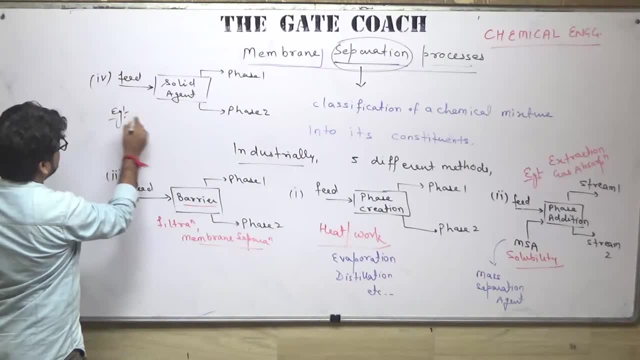 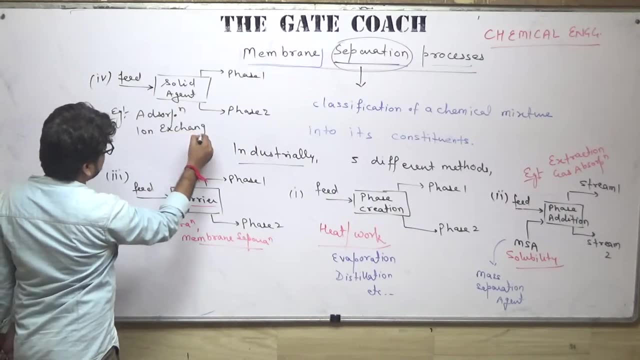 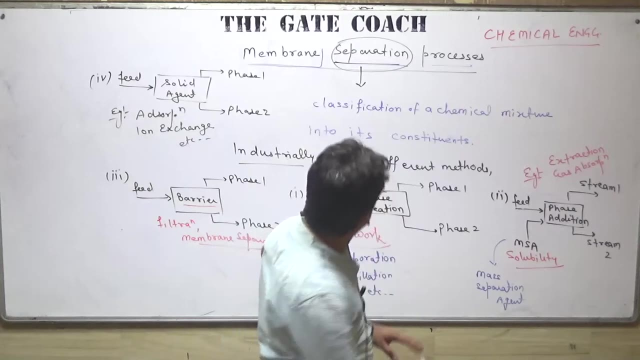 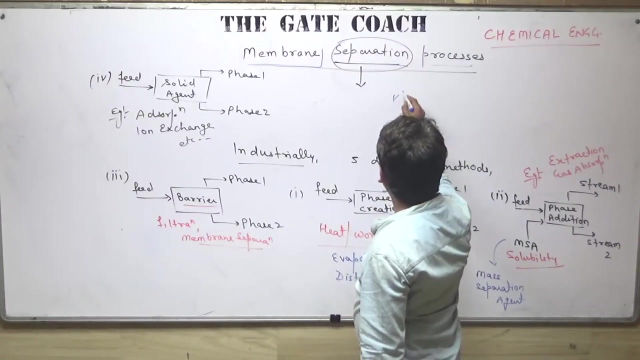 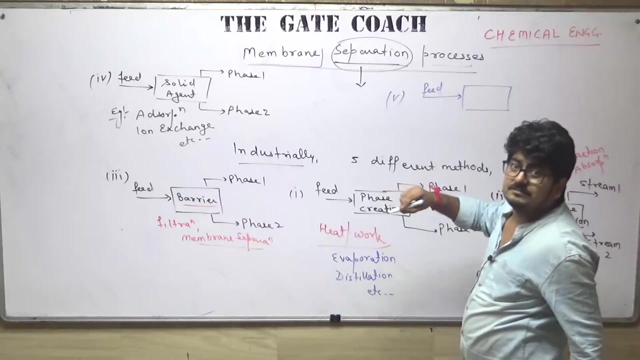 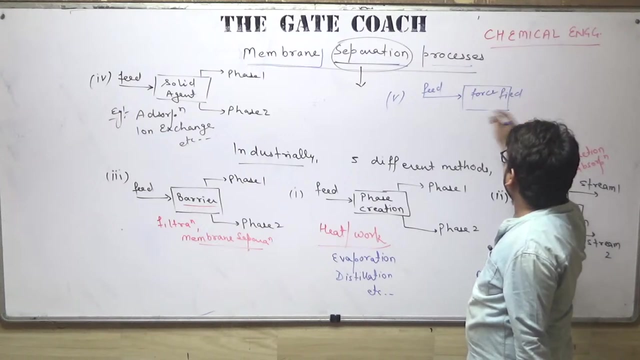 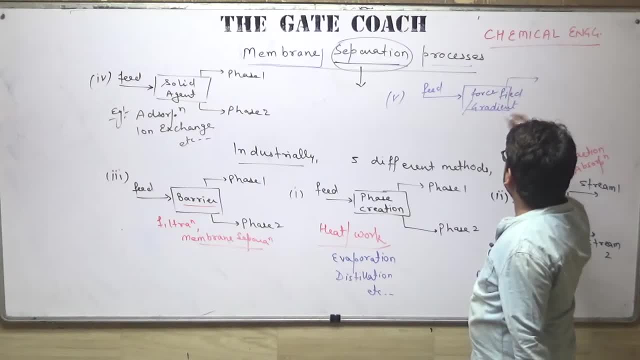 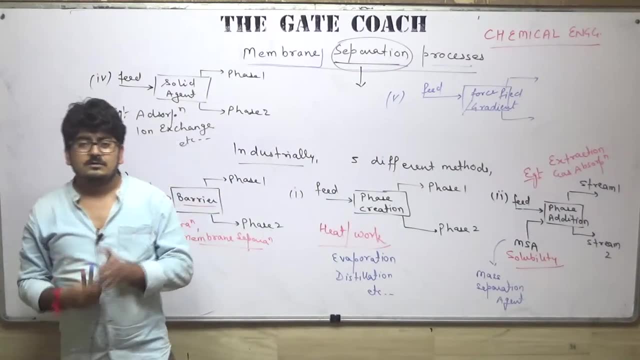 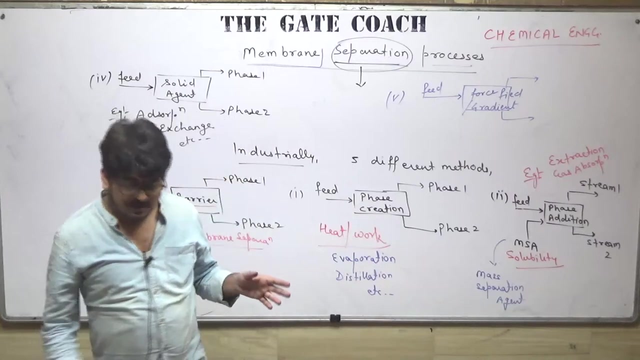 What you want to write is like: this Field is already present, or you can say: the gradient is there. Okay, For the separation part, We've sent the feed to a new force field. Some external force medium is there, or some gradients are there. 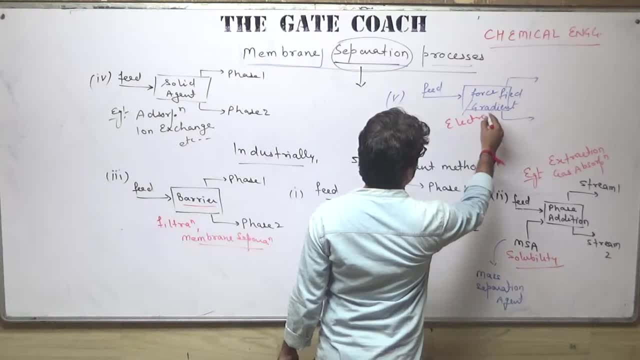 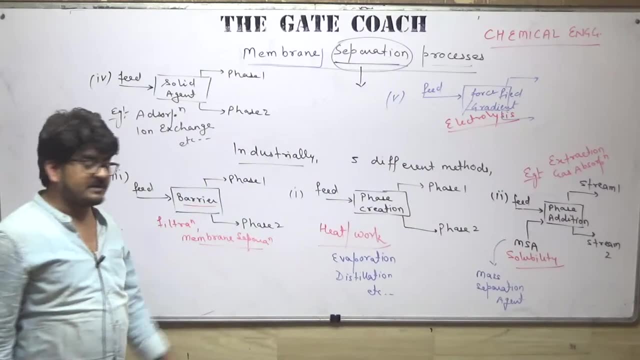 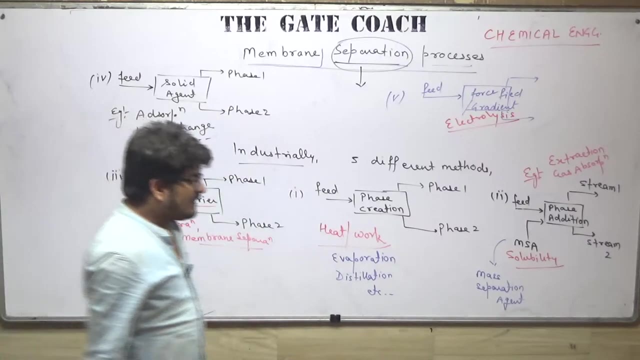 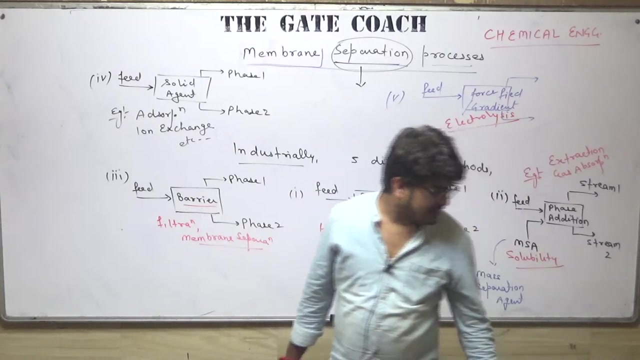 For example, electrolysis, Electrostatic separation- Right Here electrostatic separation, electrostatic precipitators, that is, magnetic drum separators which we use for the separation of solid solids normally. So, guys, these are speak Hindi, sir. okay, I will speak in Hindi and English both. 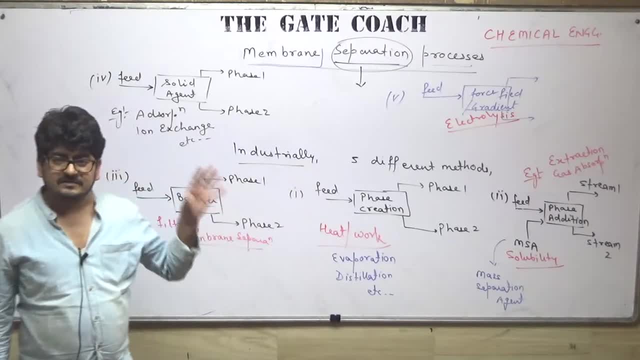 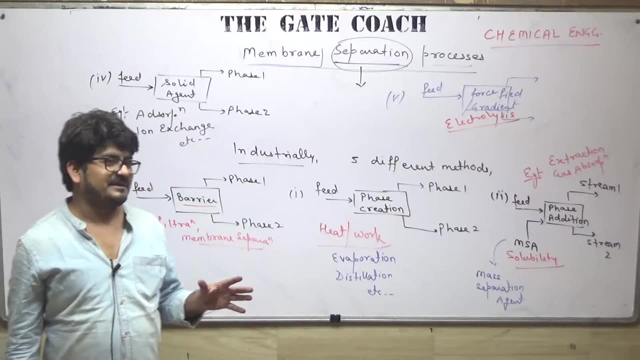 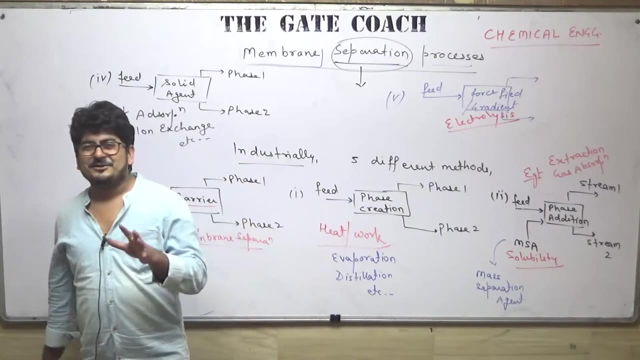 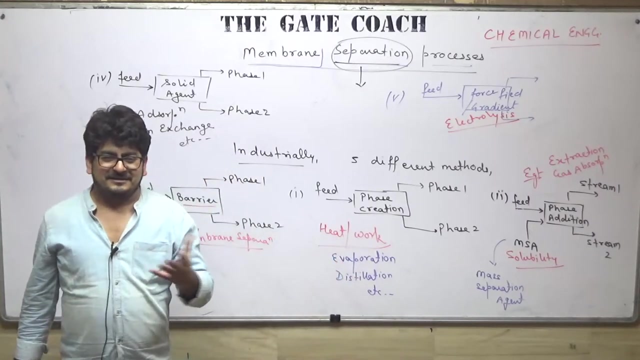 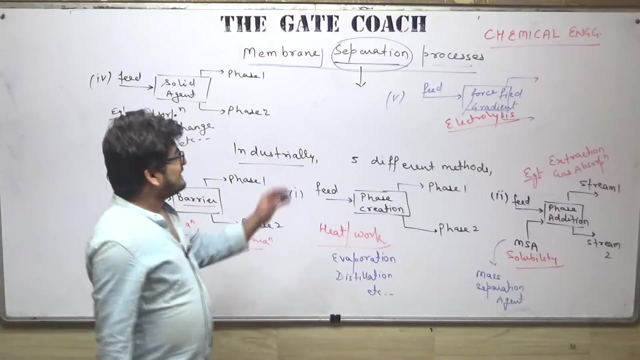 So these are the methods, main five methods which we use in industries for the separation purpose. So these are our five methods. I don't know what is the Hindi word for method or process. These are our five processes which we use in industries, I think, for separation purpose. 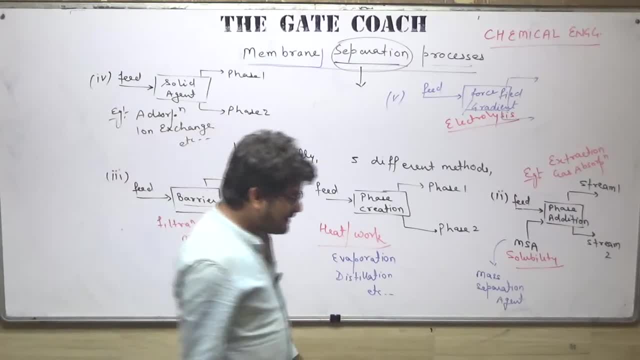 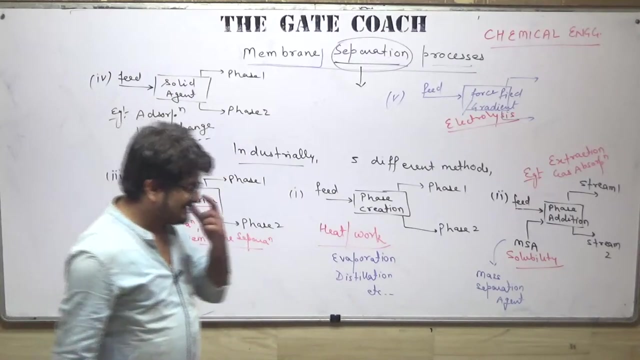 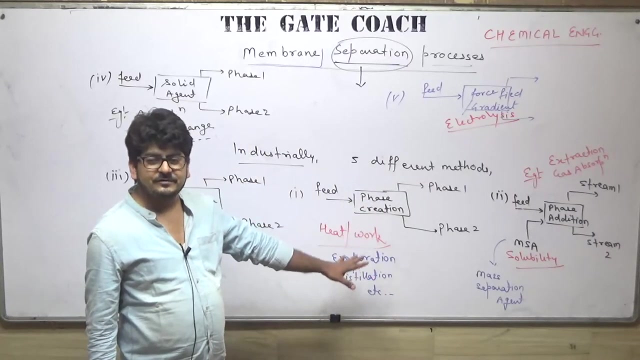 Okay, Rajneesh, will it be okay if I use some of the English words, because, although I am from Hindi medium, but it's been so long that I am using so much of Hindi words. Okay, so these are the five processes, five methods which we use for the separation. 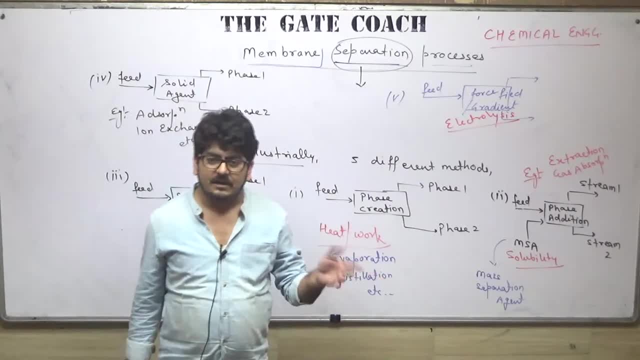 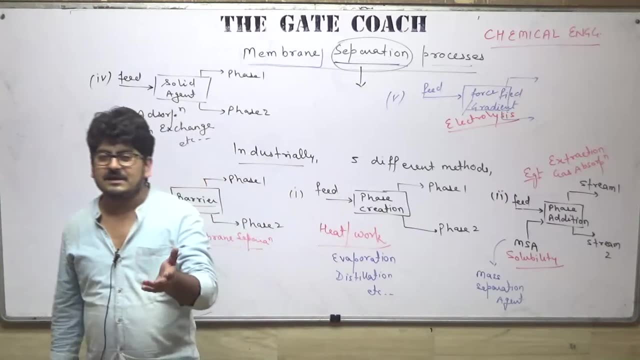 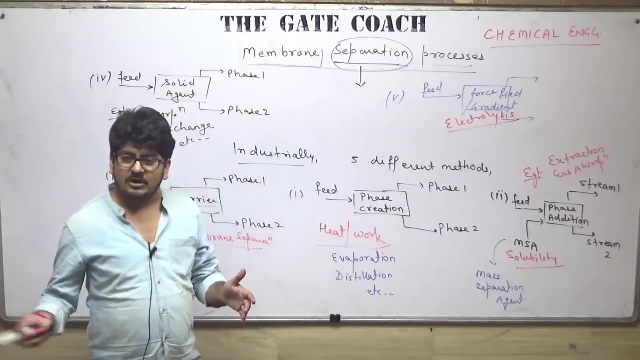 First method is phase creation. We are creating a new phase. We have applied energy and heat. we created a new phase for the separation, For example, your salt formation of salt from sea water, or evaporation distillation, where there is a reboiler and steam is used. a new phase is created. 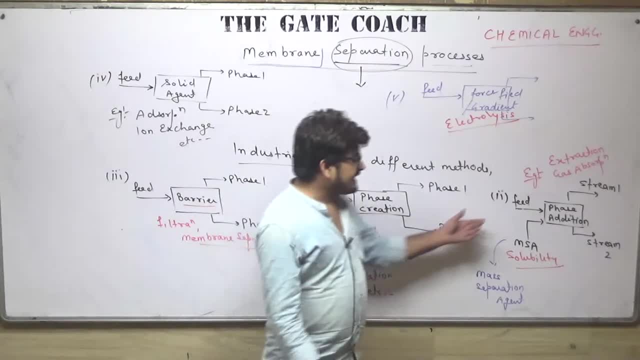 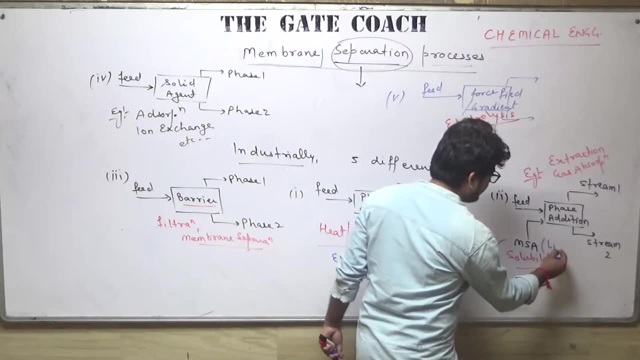 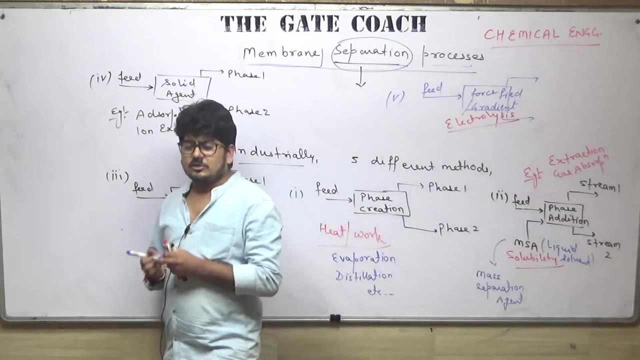 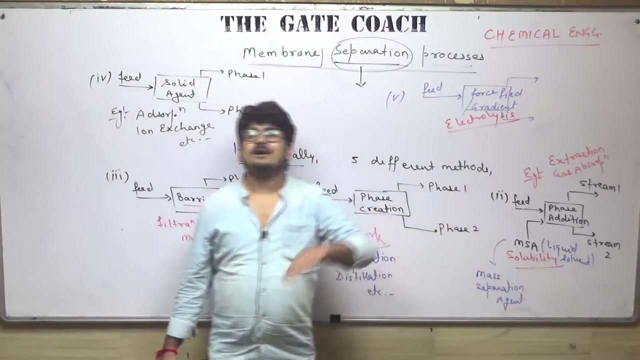 Okay. The second method is we are not creating a new phase, we are adding a new phase. Most of the time here, our liquid, is there A liquid solvent, Okay. So what happens here? So what happens here? So whatever feed there is, whatever component there is for that particular component, our solubility affinity will be more in that solvent. 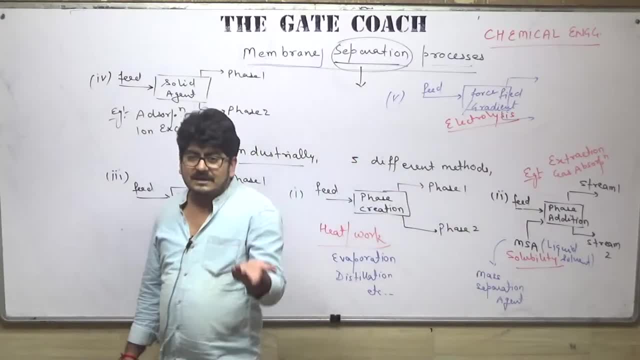 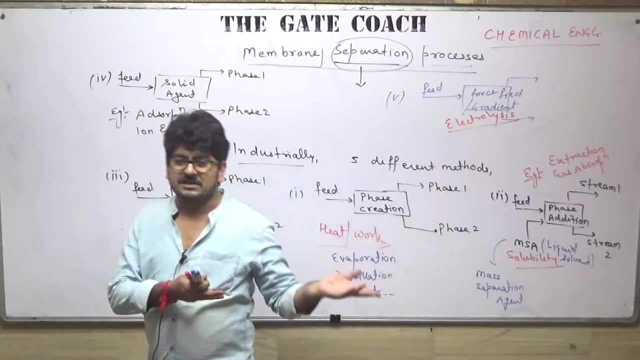 So our component will leave that feed and go there Means, like normally people do in job, that they have more package offer than other company. so they will leave from here and go there Because they were looking more attractive there. So similarly, here we have separation. 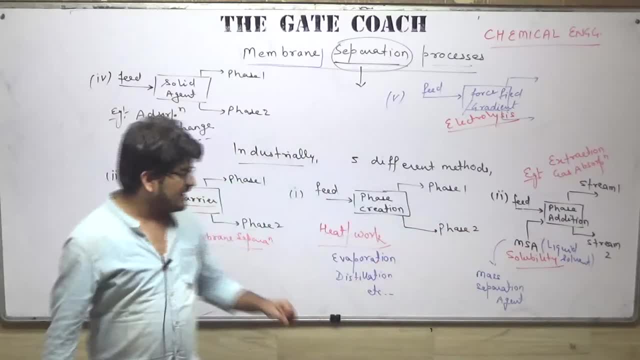 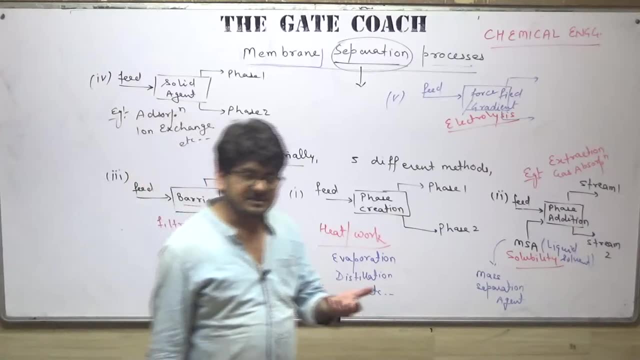 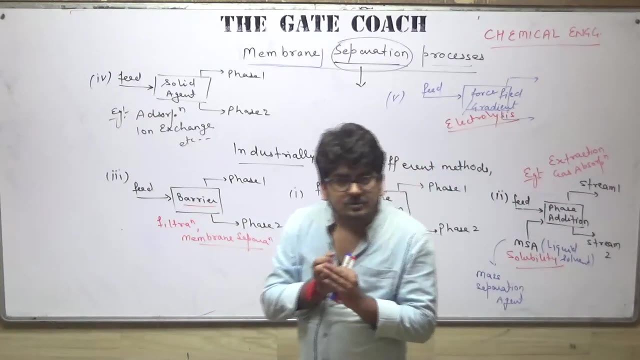 Just like extraction, gas absorption and all Okay. Third method is when we use some barrier, some porous medium or some membrane, some films etc, Interface etc. Where we pass the feed through that barrier, There are pores in that barrier. 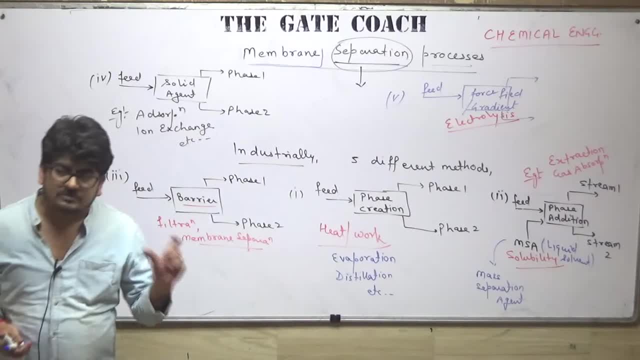 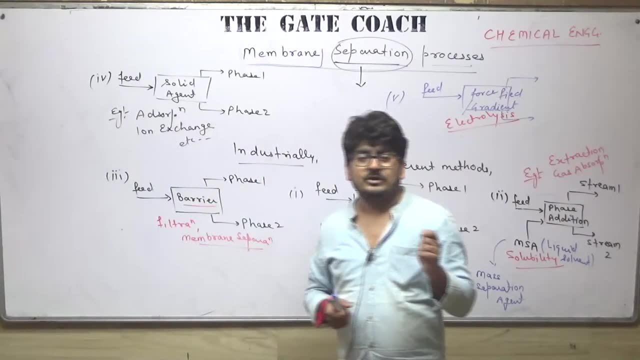 So we set the size of those pores. in this way We create that barrier, in this way We manufacture it That whatever feed we have the selective components from that, they pass through that barrier or get retained And the rest of the feed 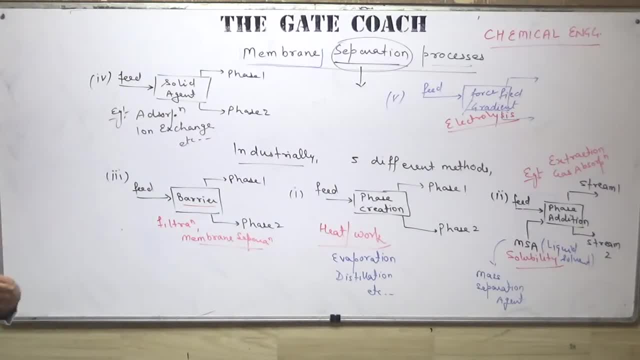 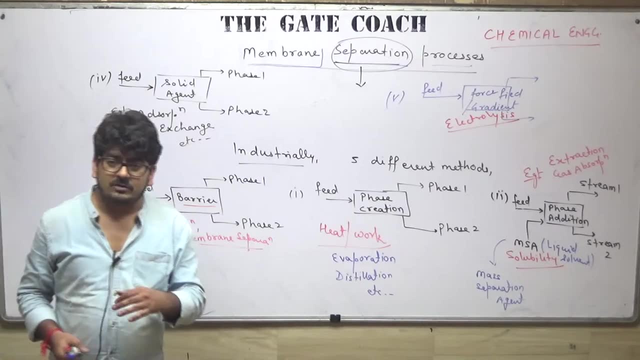 The rest of the components are opposite Means. if some components are passing, then the rest of the components will be retained, Just like membrane separation, filtration, etc. Filtration- I hope you all will be clear. We send the solid-liquid mixture in a porous medium. 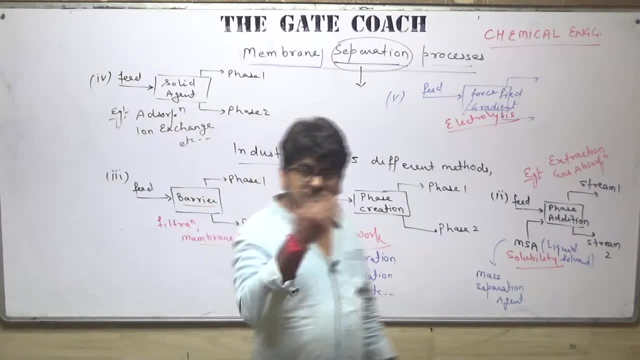 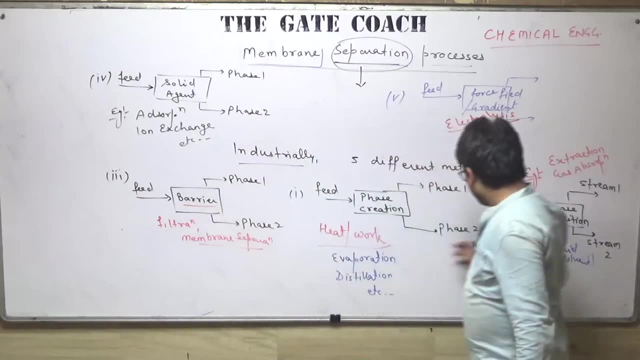 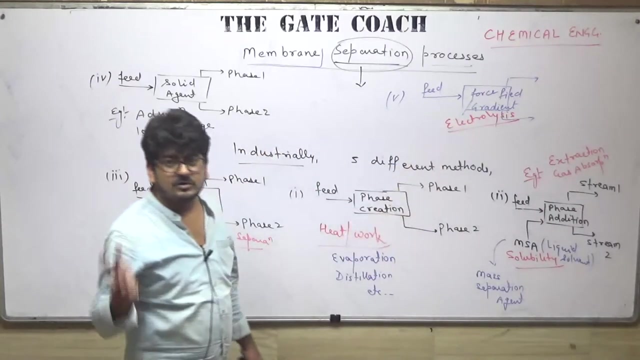 That is called filter media or septum Solids retain liquid pass. Separation takes place. Fourth method is absorption: ion exchange, When we, instead of liquid solvents, we send the solid agents. Okay, The last one is when we send the feed to a porous field. 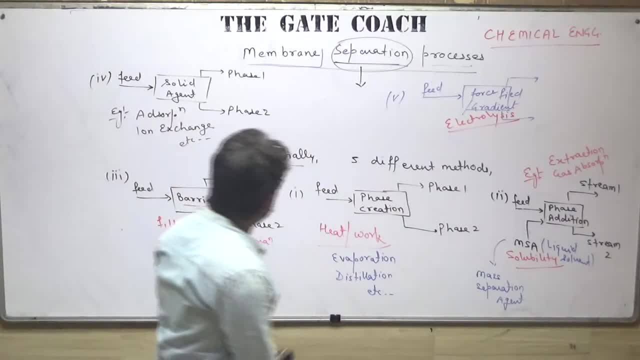 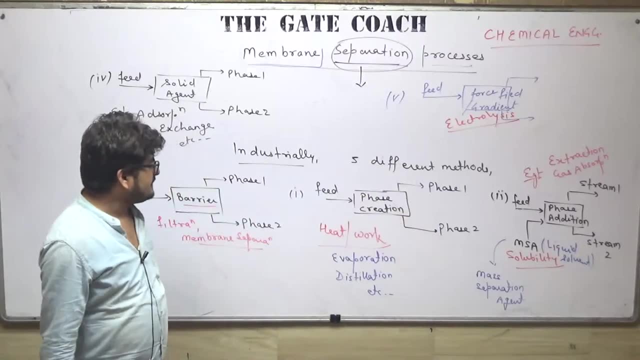 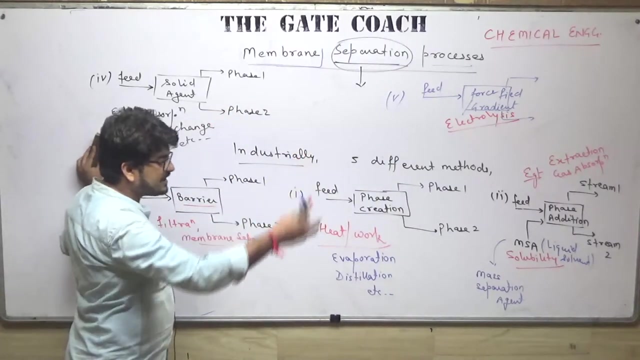 Like electrolysis. Okay, So these are some methods which we use in industry for the separation purpose. Now I will not go in much detail of all of these things Because I hope all of you know this part. Okay, This distillation, all these things you will study in your respective subjects. 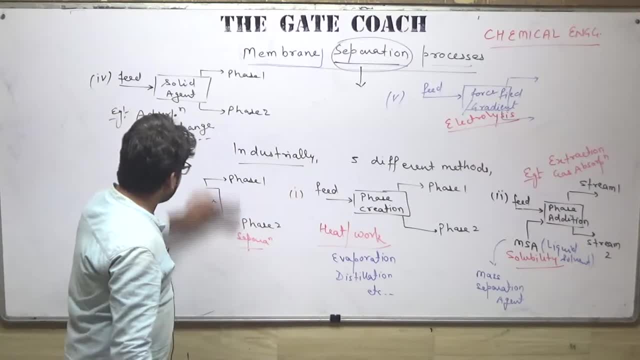 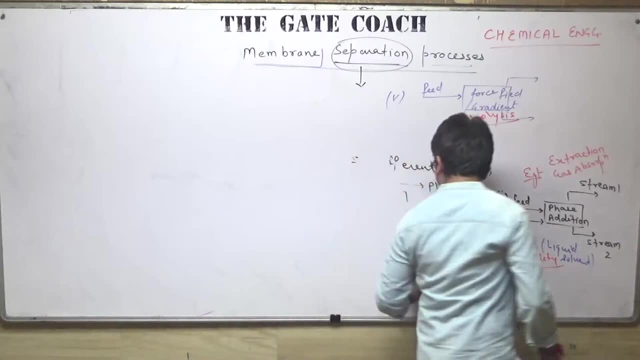 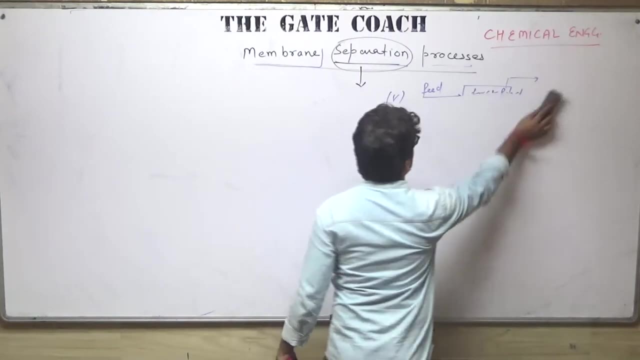 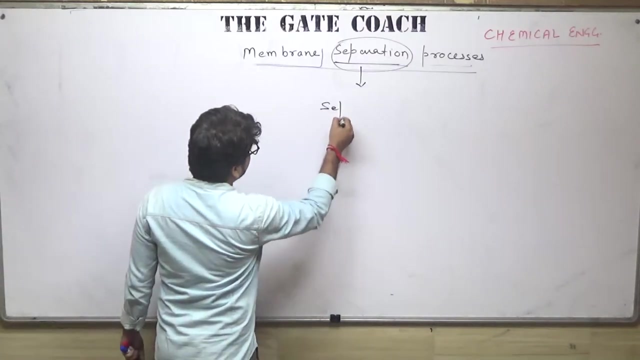 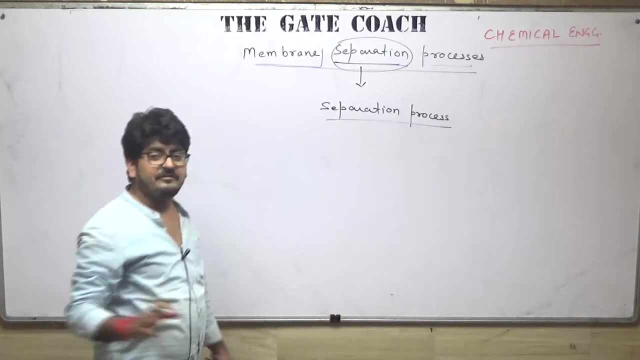 Evaporation, distillation, extraction and all Okay. Second basis is guys to separate, to classify the separation processes. If I talk about a separation process, So these were the five ways, five methods which we use for the separation purpose. 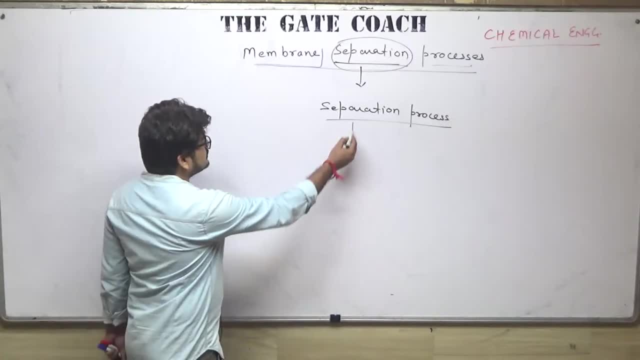 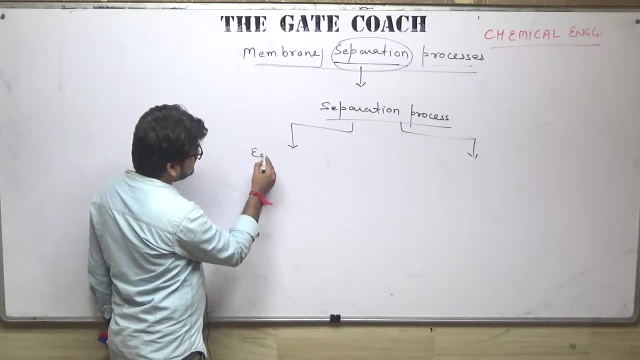 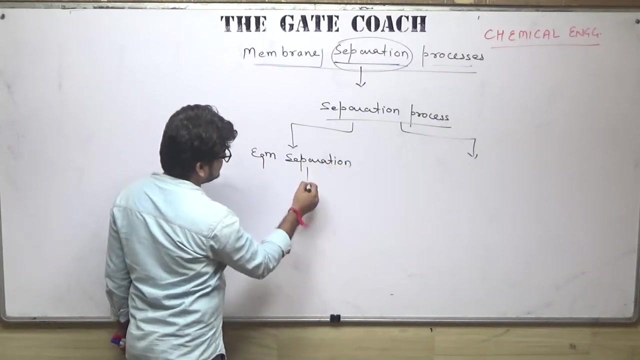 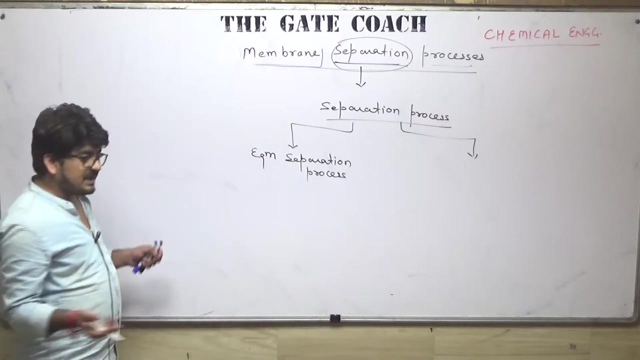 Now, if I talk about the separation process, So I can classify the separation process into two categories. First is equilibrium separation process, Where the process, the separation, takes place based on the equilibrium state of the system. Equilibrium of the system. Okay, 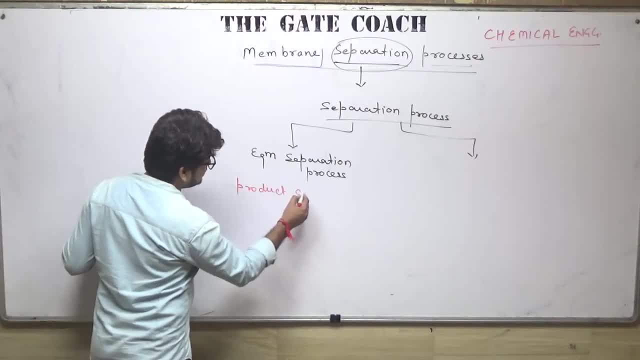 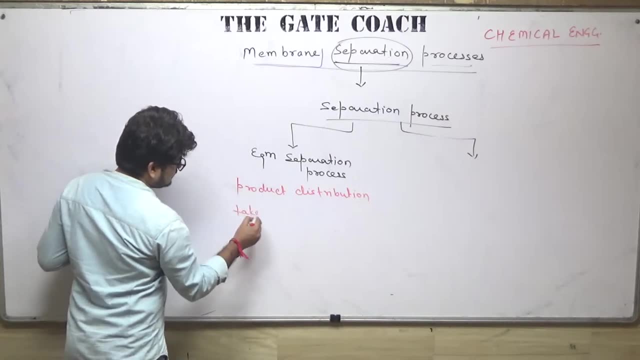 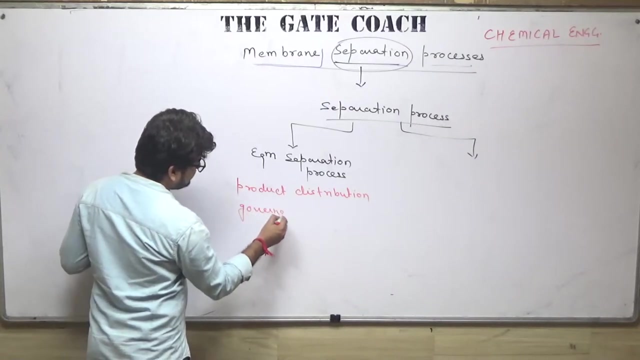 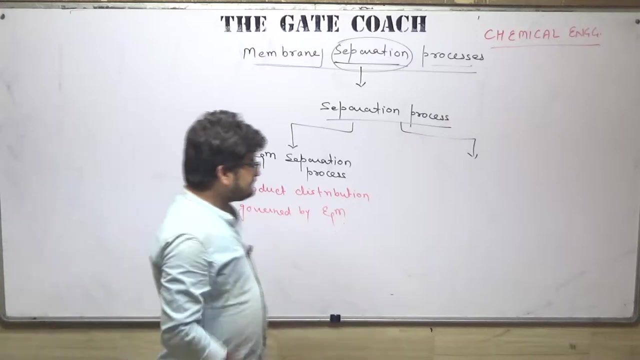 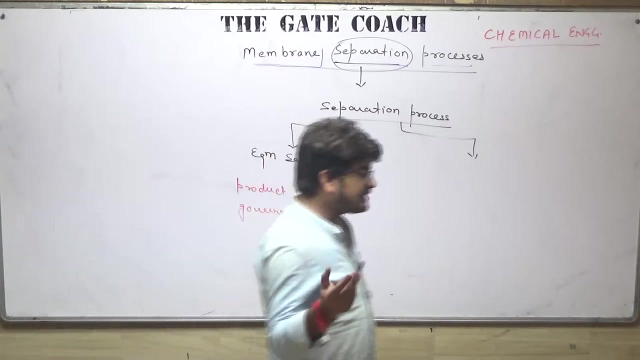 Like you can write it, as the product distribution, the separation of the particles or molecules, components, takes place, or I should say, governed by chemical equilibrium. Okay, And I hope all of you know that. Okay, In any separation process, for example, distillation, absorption- there are so many processes, are there? 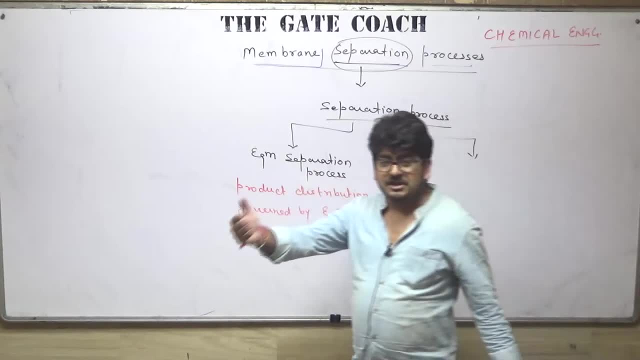 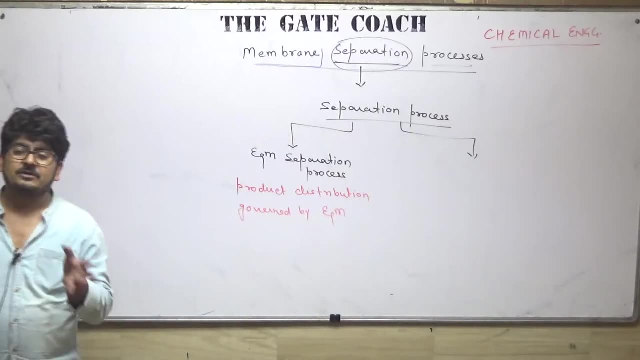 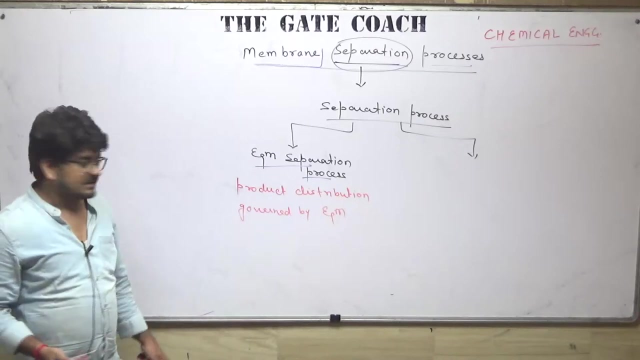 Where, when equilibrium is achieved, when the equilibrium state is achieved, then the separation stops, As the network obtained stops Okay. So in any process, when we separate on the basis of equilibrium, then it becomes our separation process Based on equilibrium. 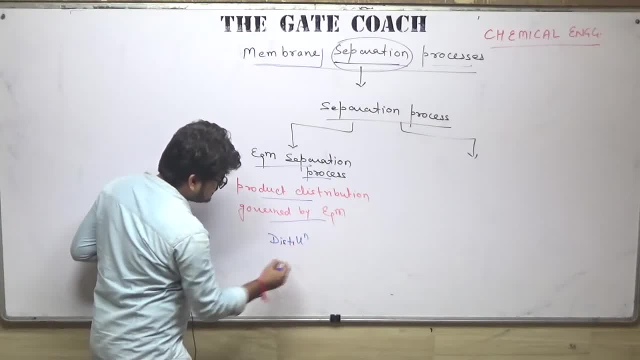 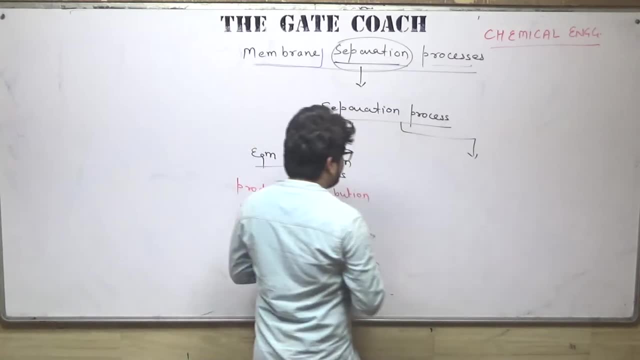 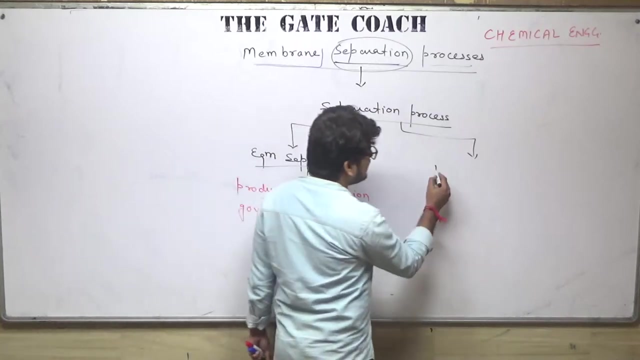 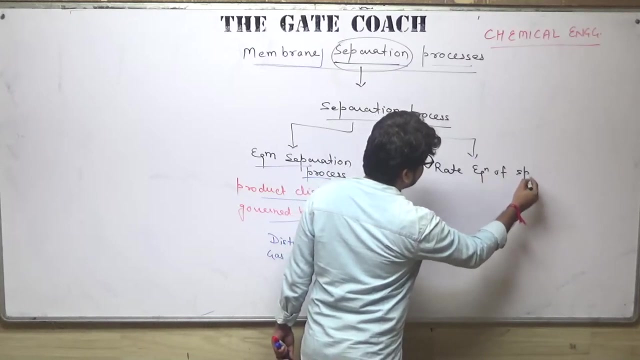 Here comes the example again: same: distillation, gas absorption, etc. Second method is where the separation process is based on, not on the equilibrium, but, other than this, based on the rate equation of species, of chemical species. Okay. 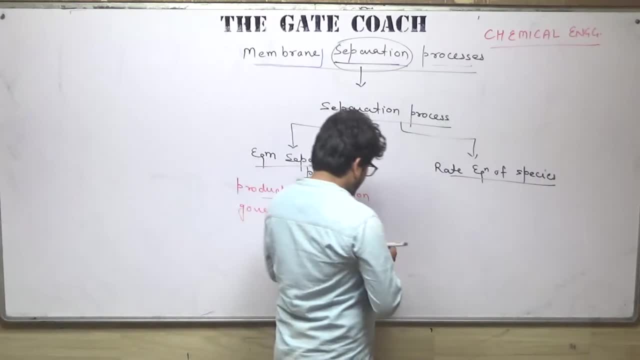 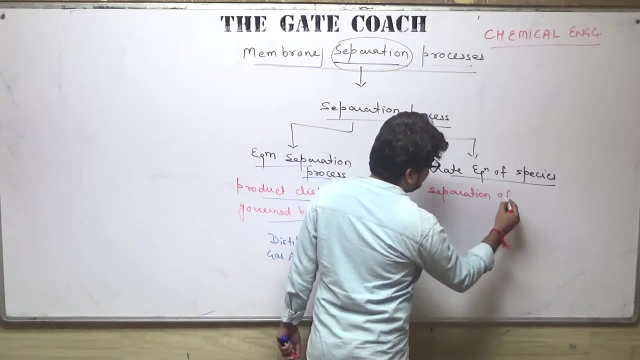 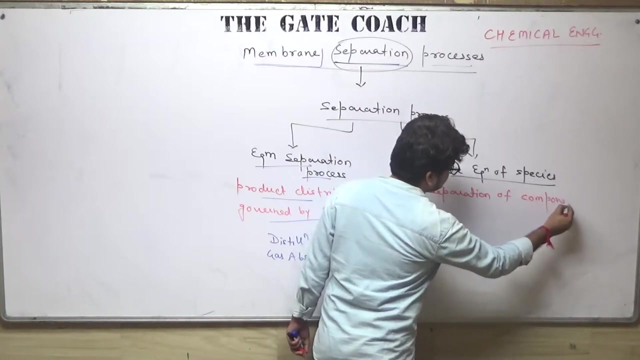 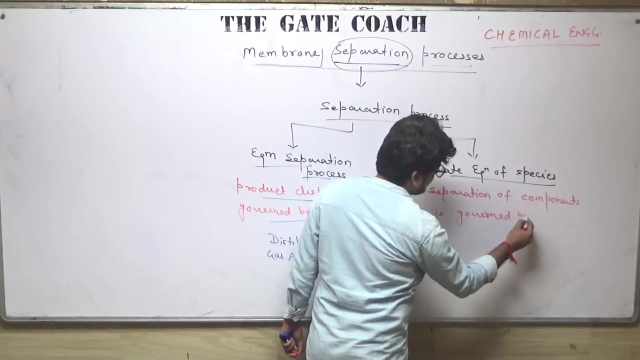 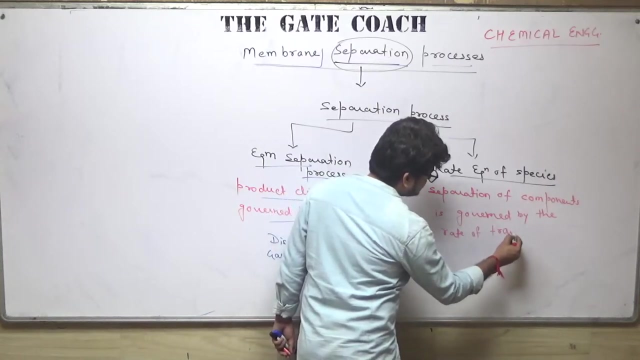 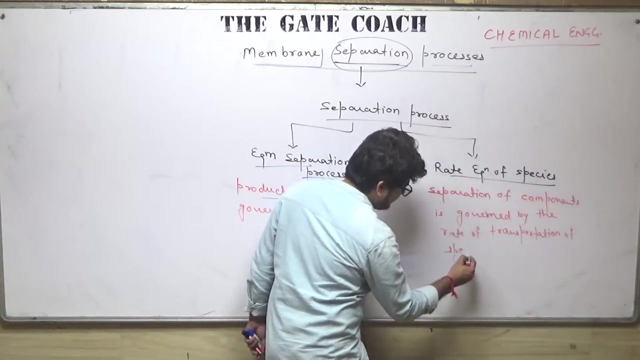 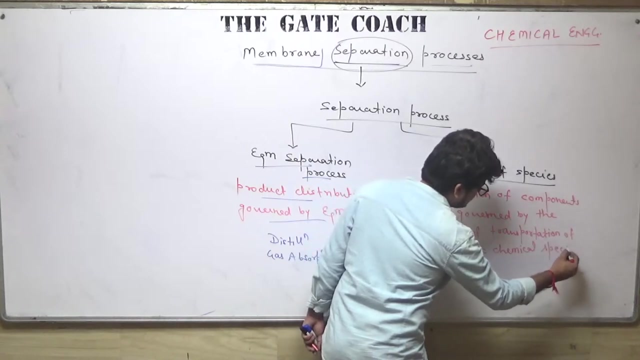 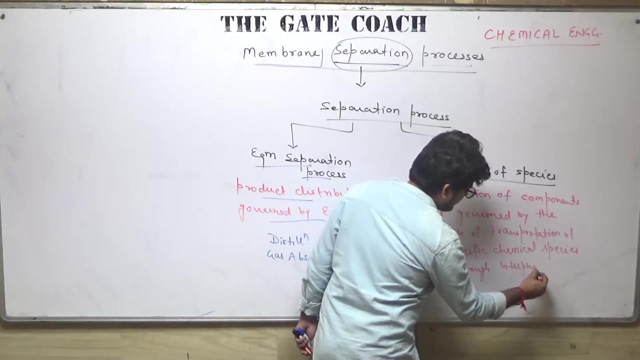 Okay. Rate equation is basically when the separation of particles of molecules, or I should say components or species is governed. rate of transport: rate of transportation of specific chemical species through interface. Ok Means in any of our mixture, in all the components. 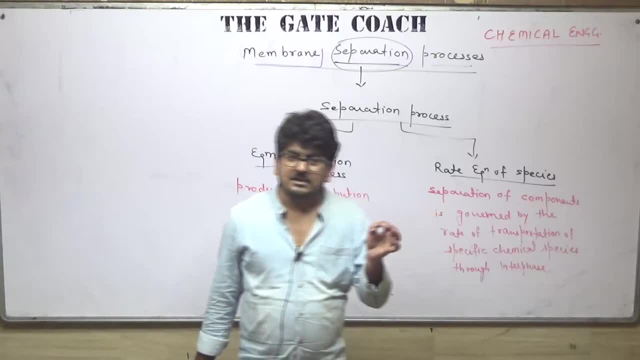 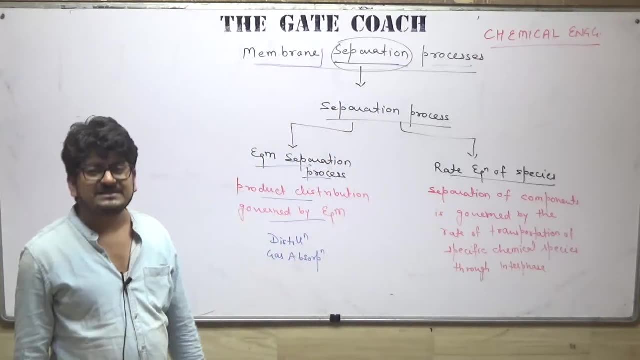 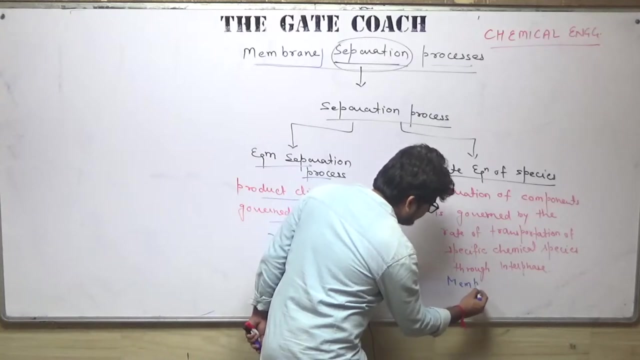 in any particular component which you want to separate, on the basis of the mass transfer rate of that component, we will decide what will be the separation process, And your example comes in this Membrane separation processes, Where we don't talk about the equilibrium. 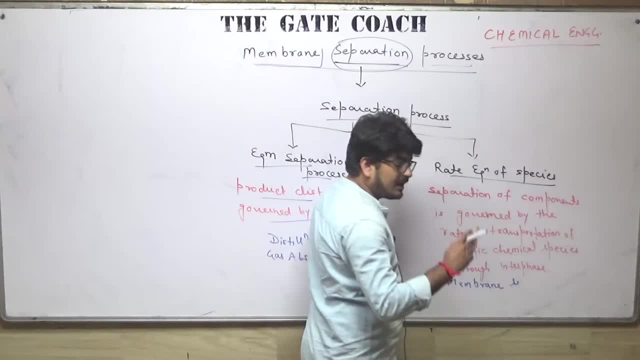 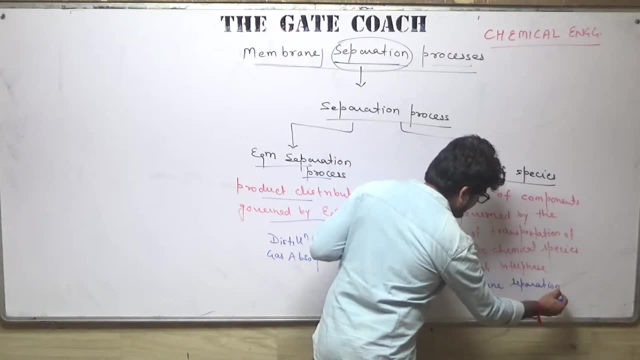 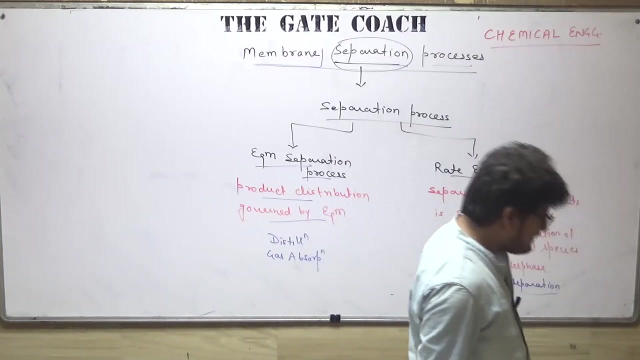 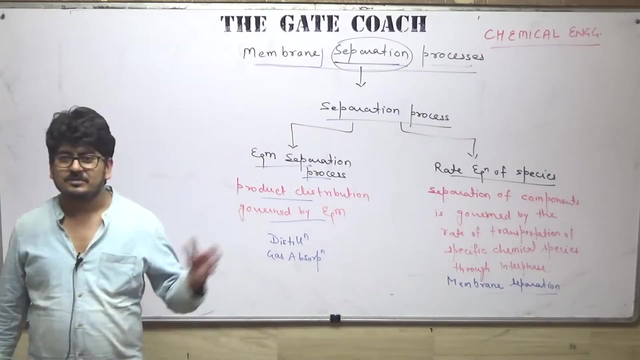 We talk about the rate of the transportation, Rate of the mass transfer of the species VLE, for example. Vapor-liquid equilibrium, Yes, in distillation. Ok, Explain in English. Oh my god, Hindi English. So many people are there. 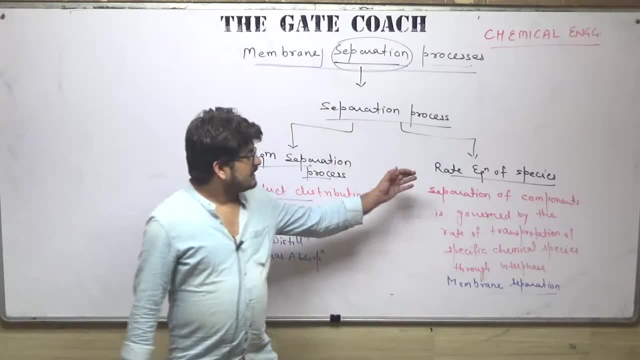 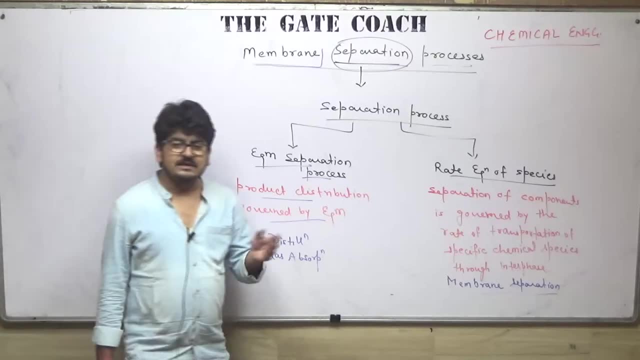 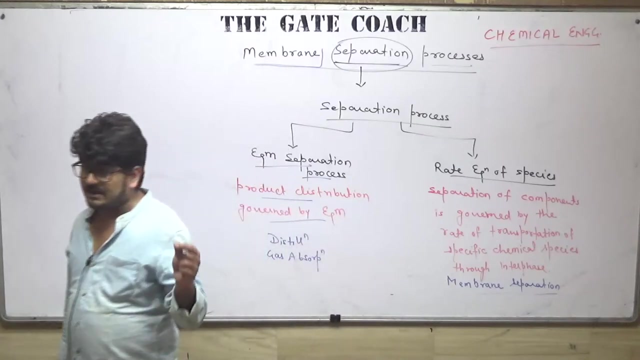 No problem, guys. So separation processes Rate equation can be classified in second category, Based on the rate equation of species Rate equation, basically the rate of mass transfer of the chemical species, Specific chemical species, through the interface. Ok Means obviously when there are. 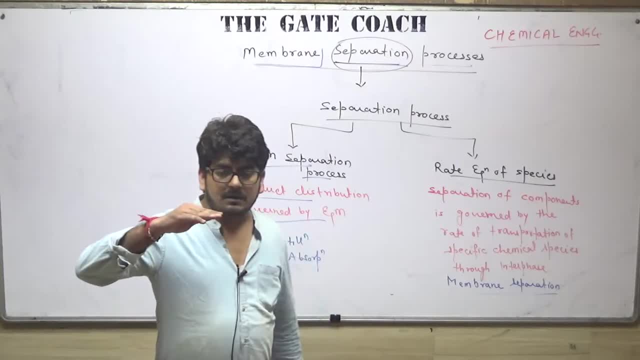 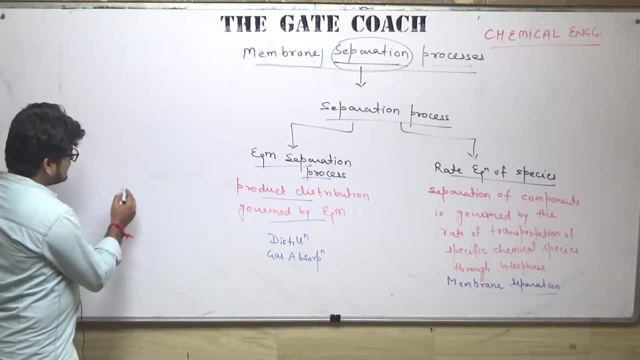 for example in membrane separation or in any other. don't talk about the membrane separation. Suppose if two phases are there, For example if two phases are there, Like alpha and beta, Or liquid and vapor, So obviously some molecules will move from one phase to other phase. 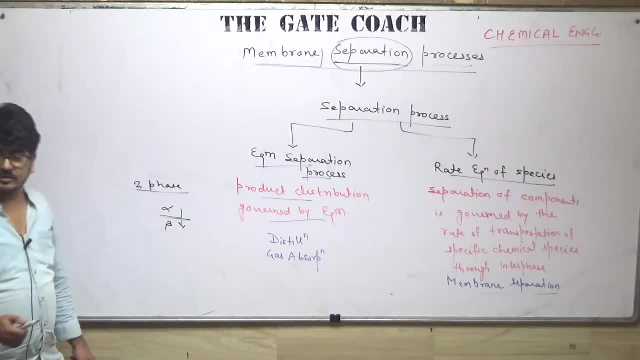 Obviously they will move through a interface, Through an interface. I hope you must have studied the two-film theory in mass transfer. Ok, So what is the rate of mass transfer of that species between the phases Through this interface? Or, for example, if 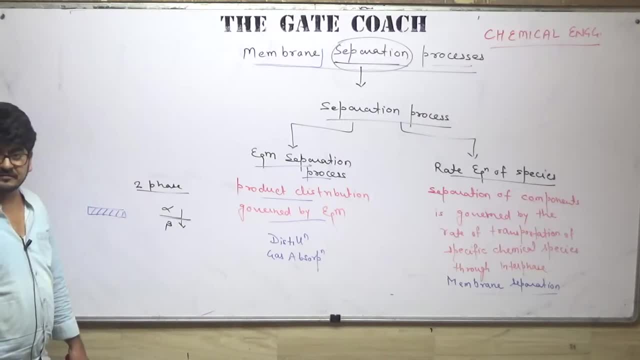 there is some porous medium or a barrier we are using for the separation Feed enters. Ok, Some of the species will pass through this medium, Some will retain And some will pass. So what is the rate of mass transfer of these species? 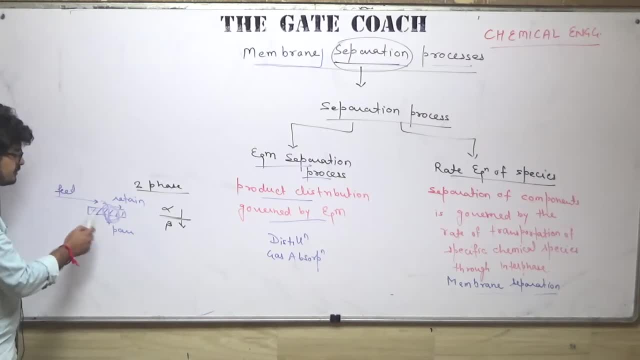 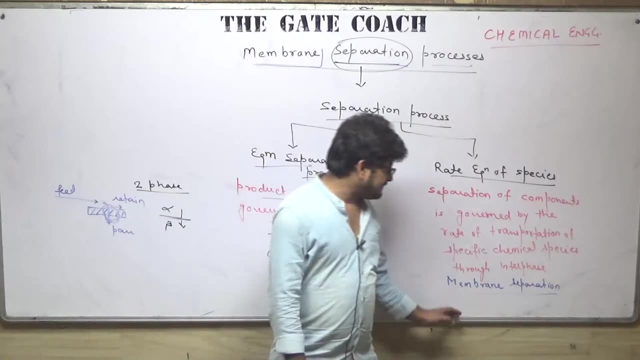 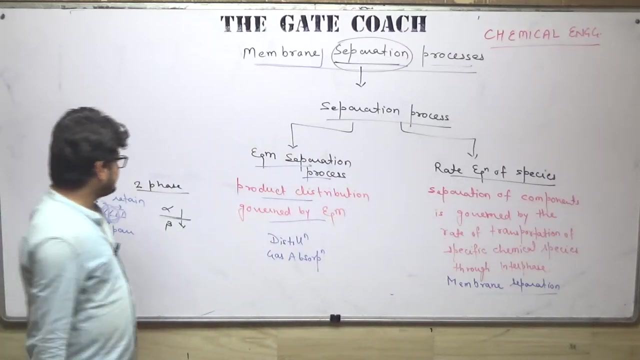 When they are moving through this barrier, When they are moving through this interface. So, based on that, we can classify the separation processes. Ok, So in this the example is membrane separation, Drying, And there are so many examples. are there? Ok, guys? 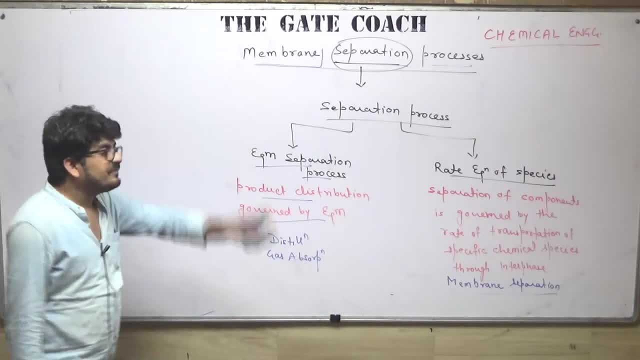 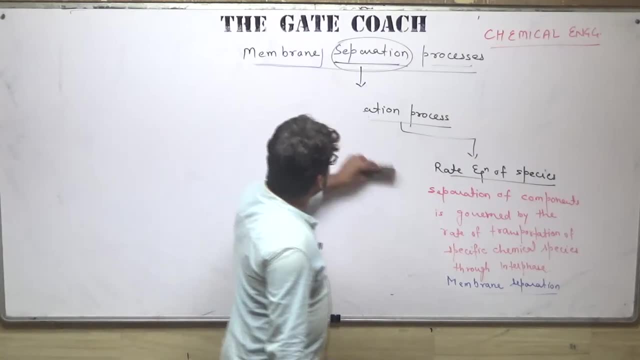 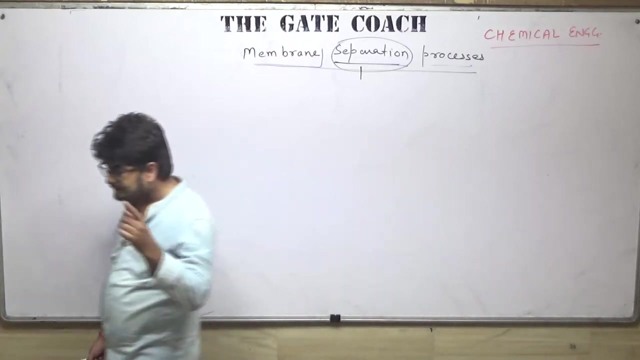 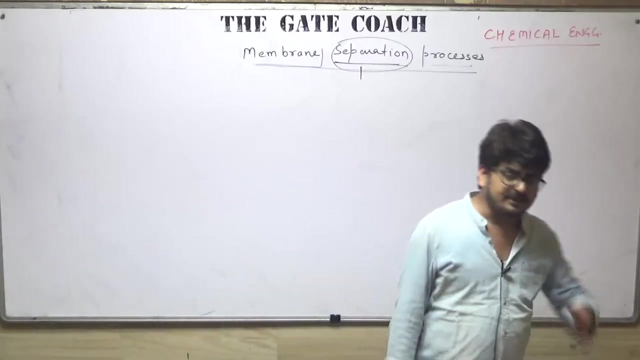 So this is something about the separation part Now. next we will talk about the membrane. But before we talk about the membrane, I want to ask to all of you- You must have heard a question At various places, May be in your college vivas. 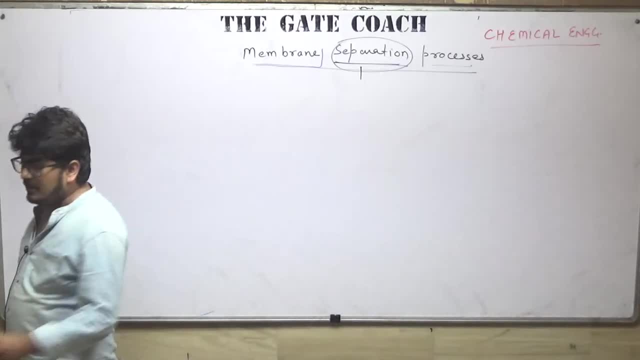 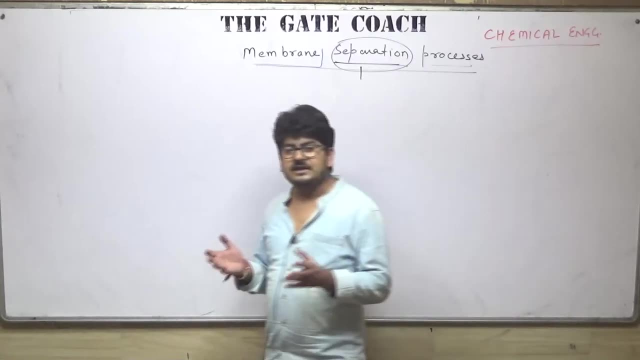 In your interviews So many places. What is the difference between heat transfer and thermodynamics? What is the difference between heat transfer and thermodynamics? So you must have heard this, Ok, And I hope all of you also know the answer of this. 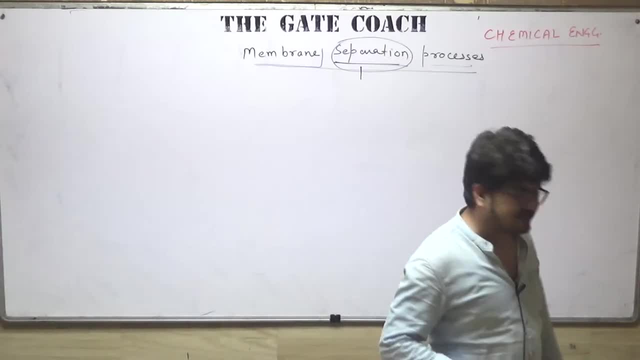 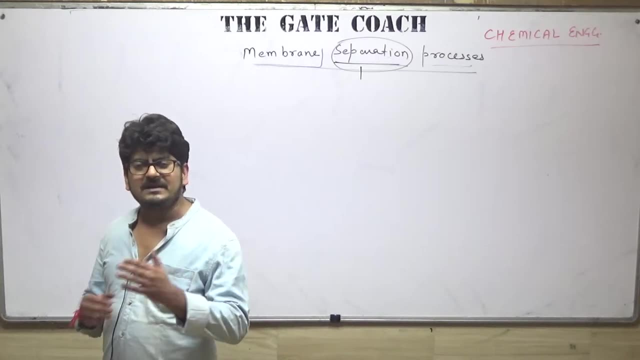 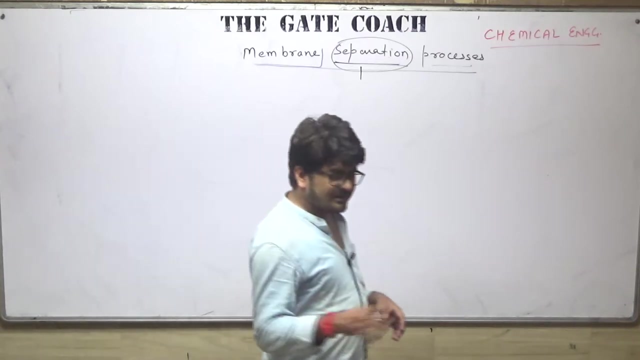 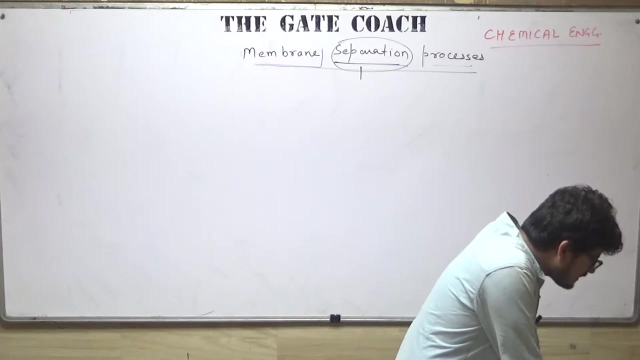 In case you don't know, then we will see about this in some other lecture Here. my question is: What is the difference in mass transfer and thermodynamics That we will discuss? Tell me guys, Sir. is absorption an equilibrium process? Absorption is not an equilibrium process. 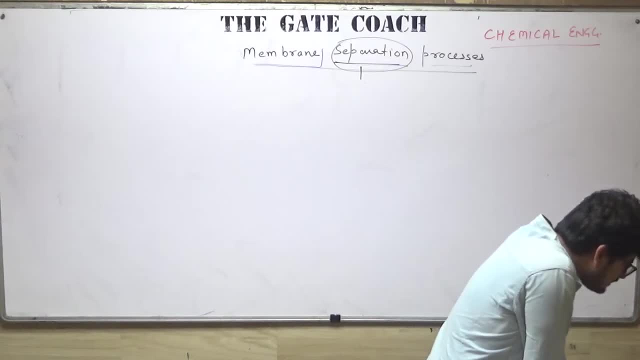 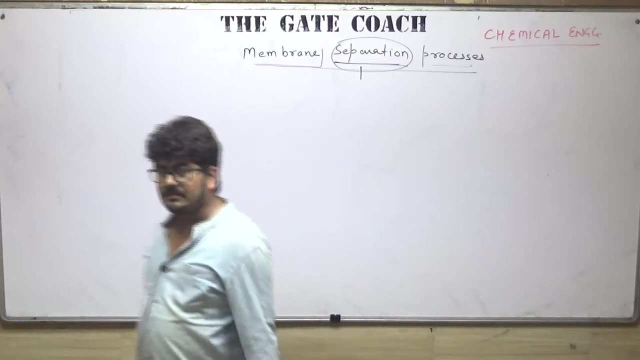 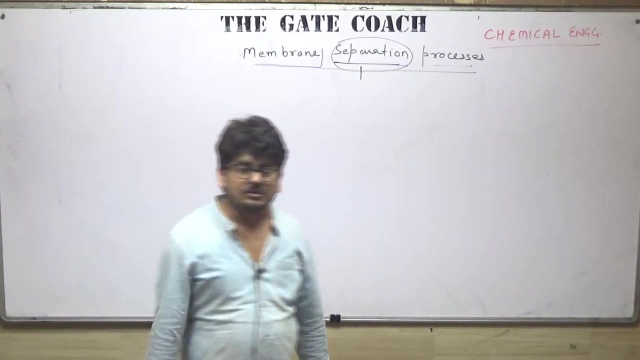 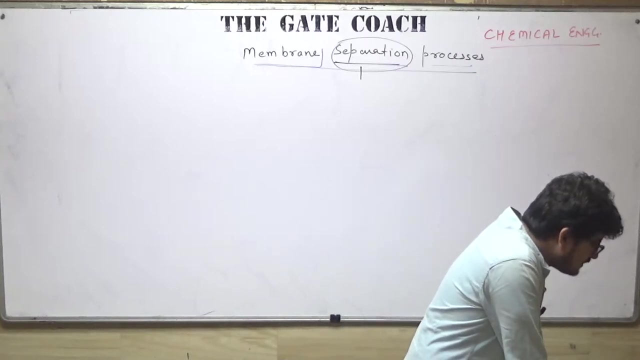 Ok, Ok, See, this video will be available on the YouTube channel, On our YouTube channel. Ok, This is the benefit of having live stream on the YouTube: That automatically the recorded version of that stream remains on the channel. Ok, So you can access this session afterwards as well. 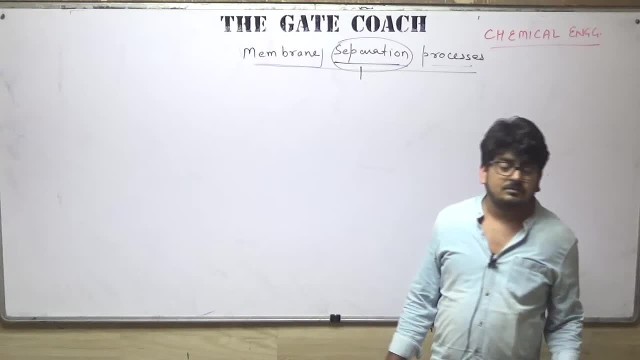 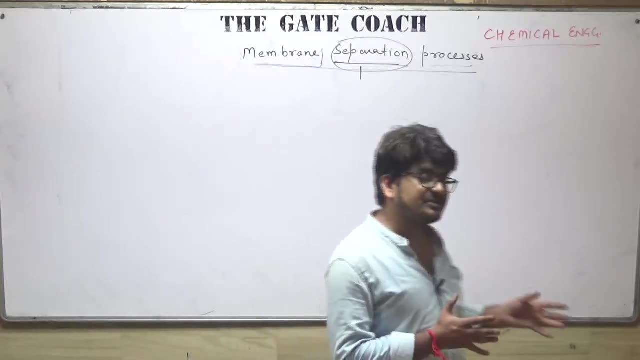 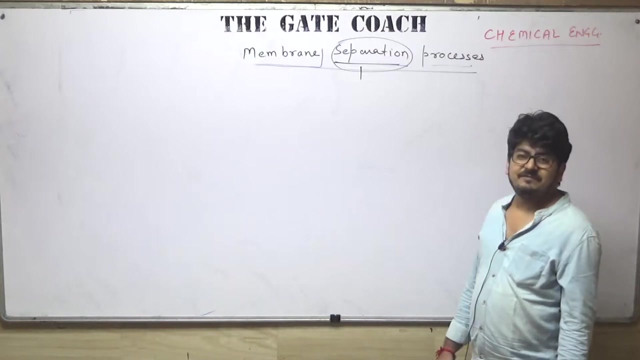 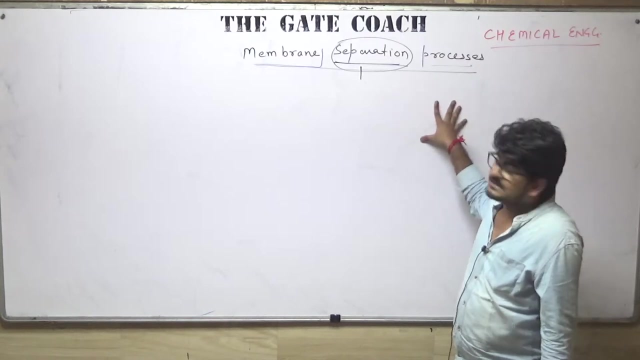 Now, I was talking about the Mass transfer and thermodynamics. So, guys, tell me What is the difference Between mass transfer and thermodynamics? Ok, Or let me simplify one this question for you: In separation processes, In separation processes, What is the role of mass transfer and what is the role of thermodynamics? 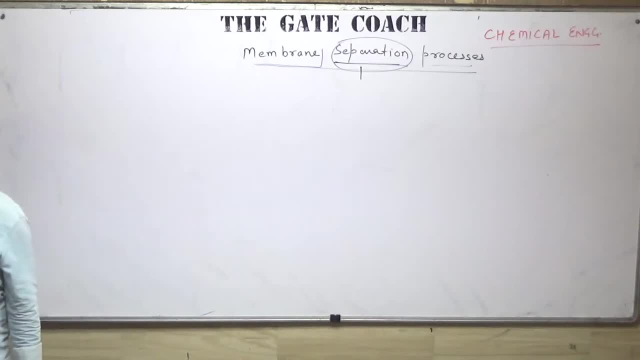 Yes, First, the mass transfer, The mass transfer and thermodynamics. The mass transfer and thermodynamics: It's because the mass transfer and thermodynamics are the two states that are the ones that are the most important things. Yes, Of course, the mass transfer and thermodynamics. 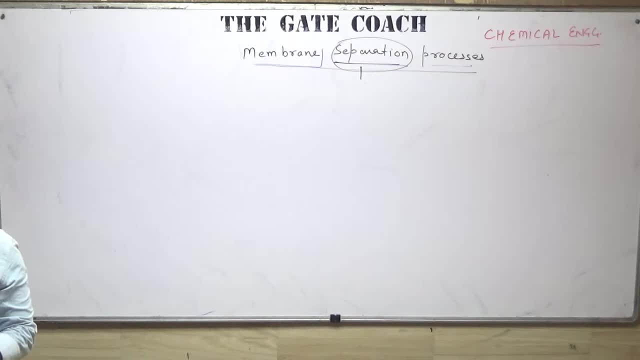 The mass transfer and thermodynamics is a gas. Bruce, you could call it a gas. I just called it gas. I don't know, But if you look at it You will hear: The gas is the gas. That is a gas. 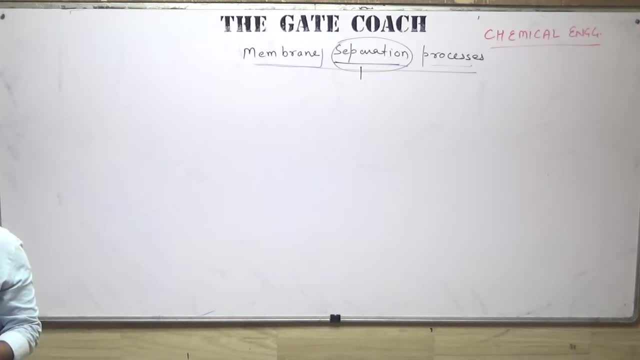 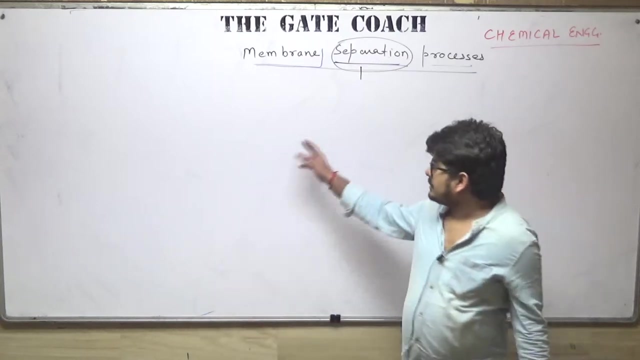 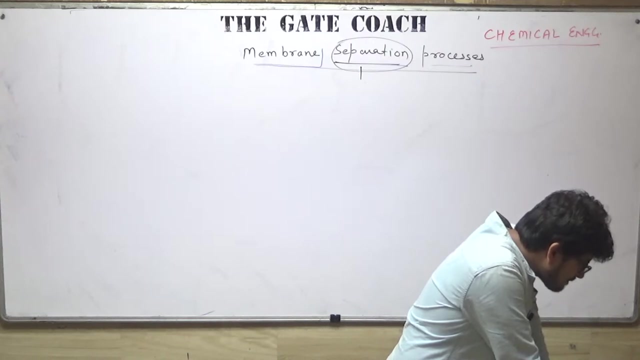 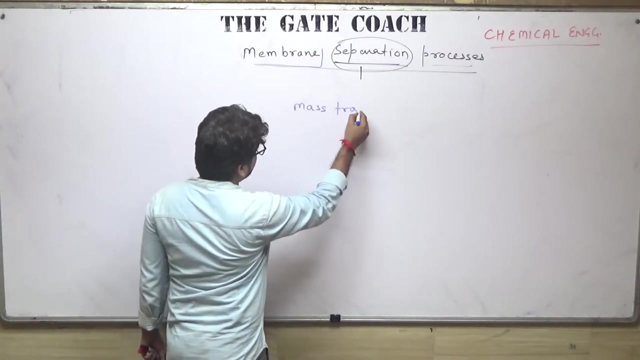 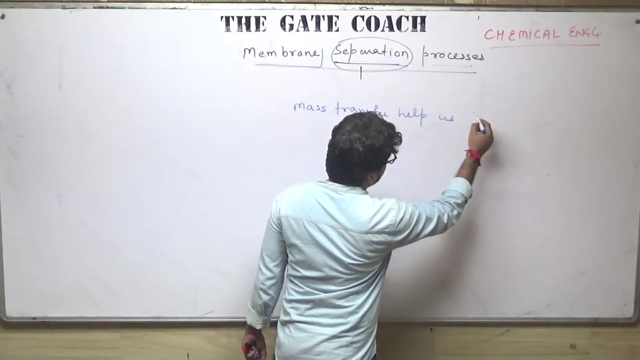 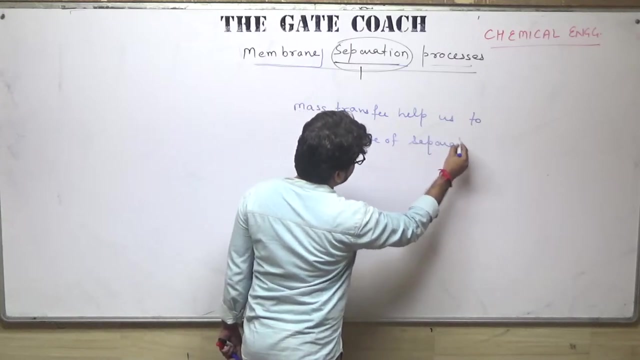 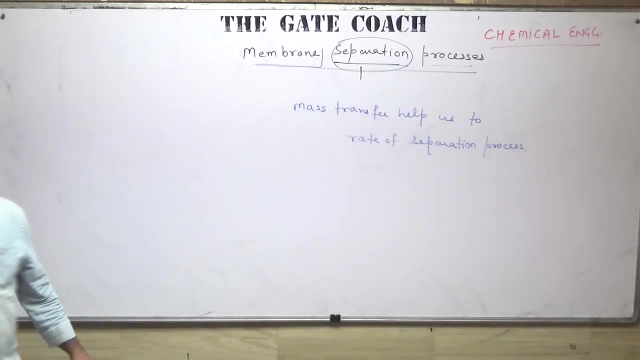 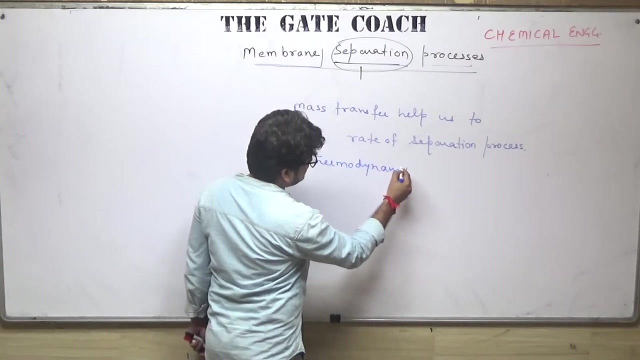 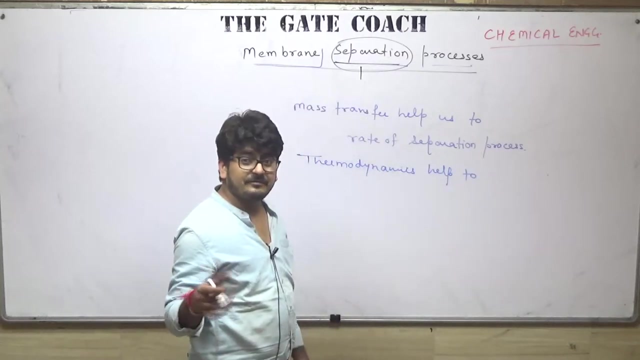 It is a gas, absorption comes under the equilibrium separation process. okay, thermo gives the van equilibrium achieved, mass transfer gives the rate. wonderful guys, absolutely okay. mass transfer will help us to figure out a the rate of separation process, while thermodynamics help to figure out, as you said, van equilibrium is achieved means the extent. 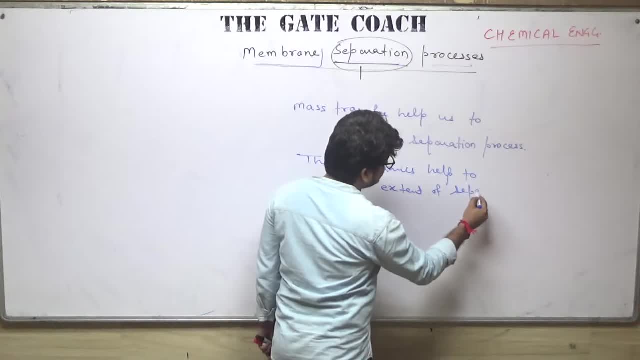 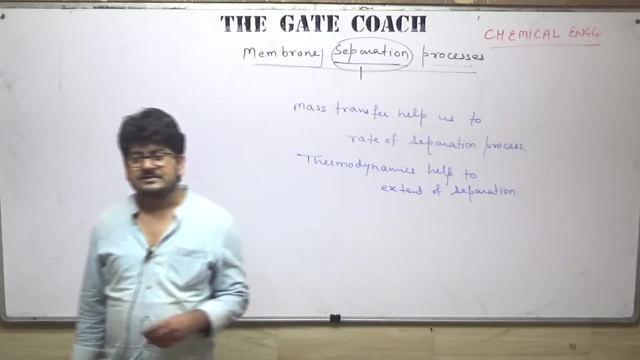 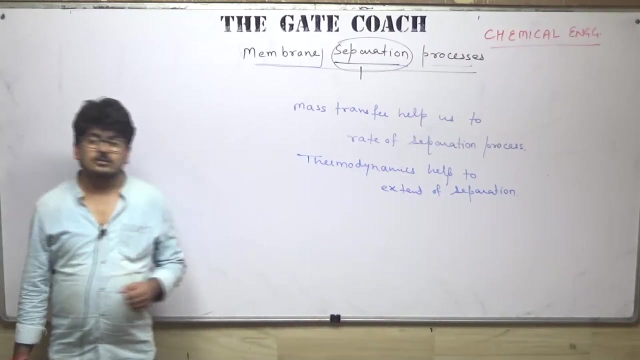 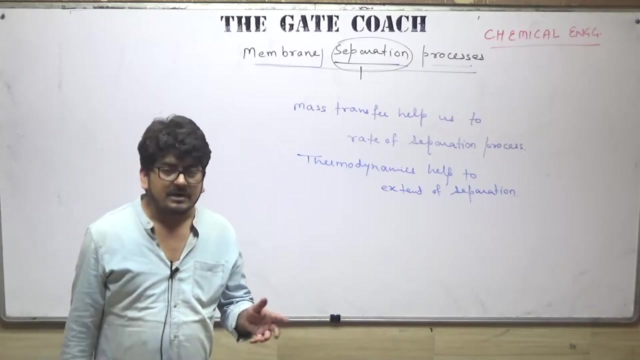 of separation process, but the time of separation, mass transfer help us to identify the rate of separation process, with the help of which we can find out the time required for the separation, and, in thermodynamics, thermodynamics help us to find out the equilibrium state. when the equilibrium state will be achieved? okay. 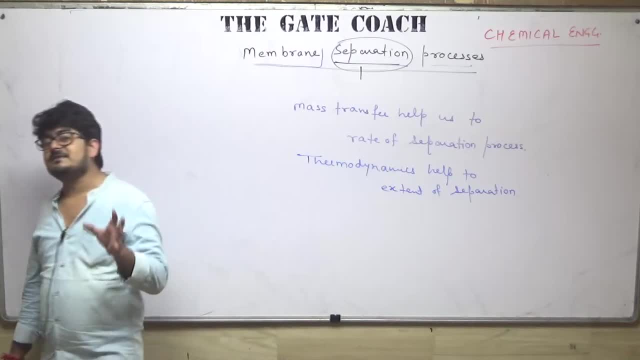 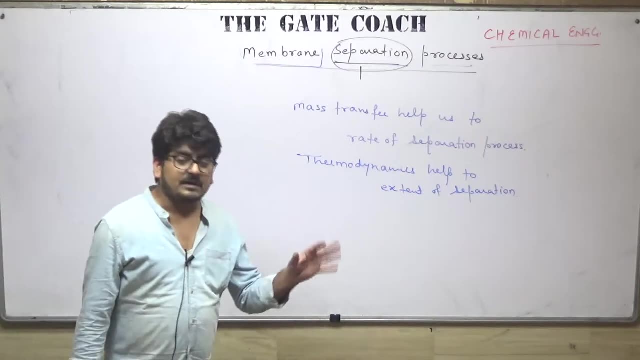 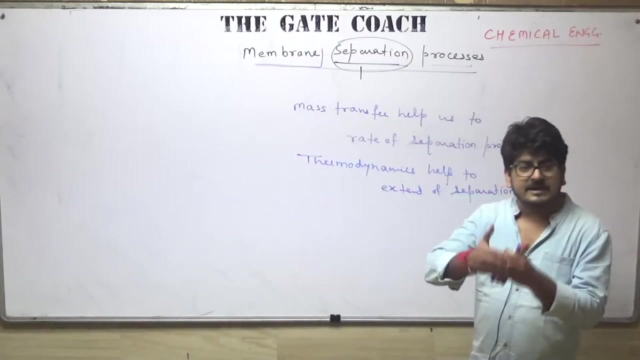 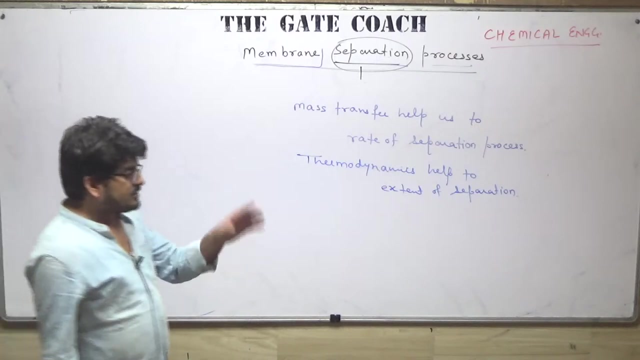 ultimately, we know that in any separation process, fall equilibrium isē, then the separation stops. so we can say the extent of separation. the thermodynamics help us to identify the extent of separation, when the separation, separation will take place, up to which extent? okay, so, guys, it's good that you. 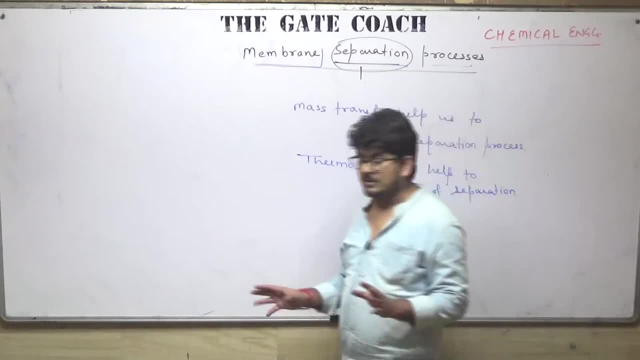 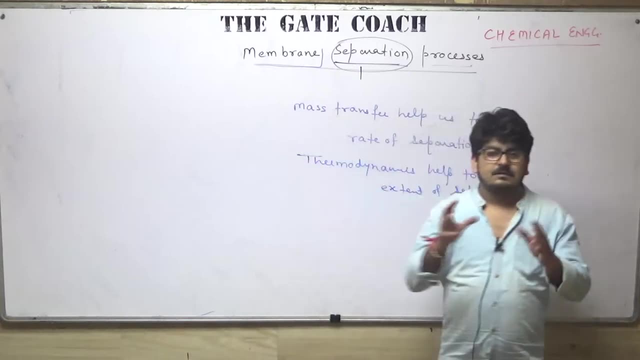 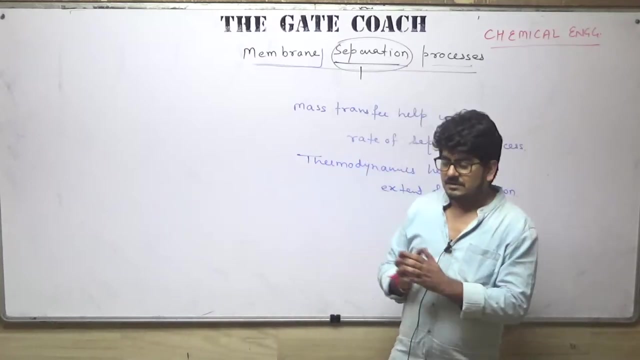 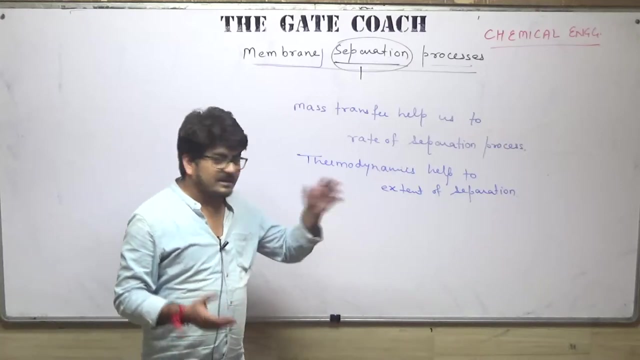 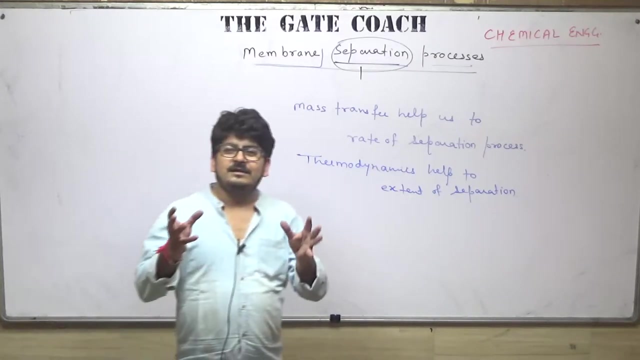 have some basic knowledge and a sufficient knowledge about this topic. okay, so tell me one more thing about this part. sorry if I am going out of the direction, but I just this question comes in my mind, so that's why I'm asking. okay, if I am going out of the league, sorry for that in advance, but what is the you must? 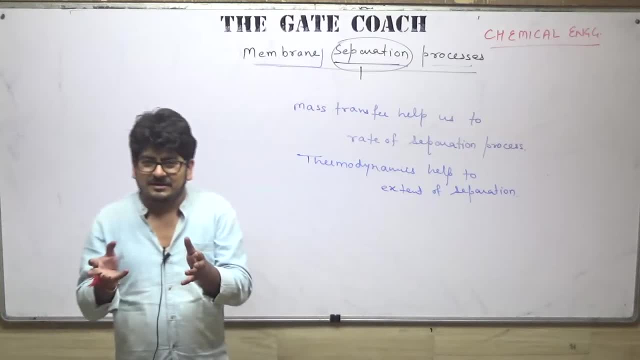 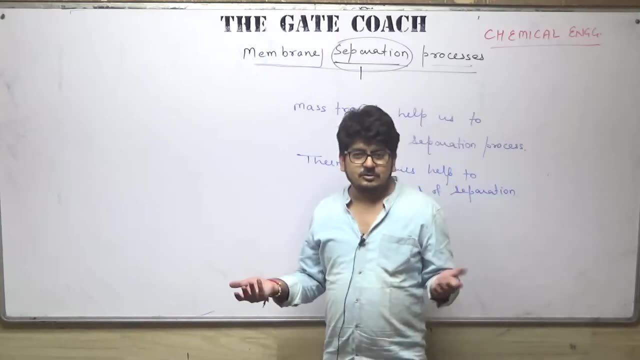 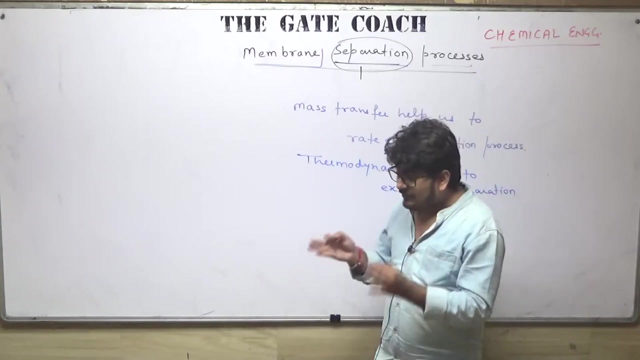 have heard a question: what is the role of a chemical engineer? okay, and or what is the difference between chemist and chemical engineer? as you know that we are a chemical engineer, we do not study chemistry in the four years of BTEC, even in the masters in the PSG, anywhere. we don't study that subject. okay, we have. 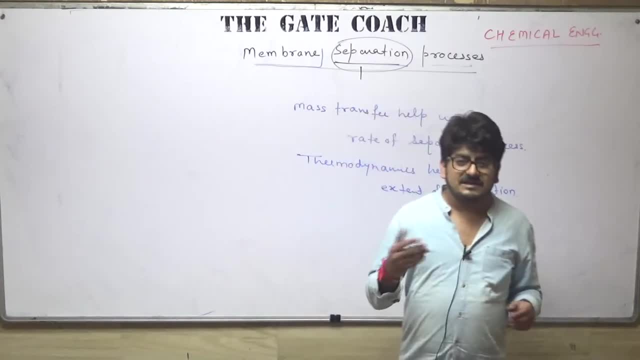 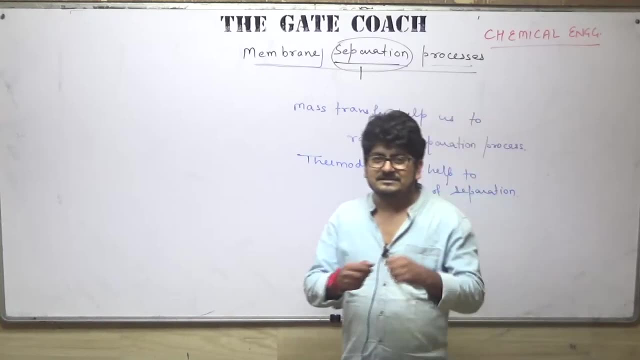 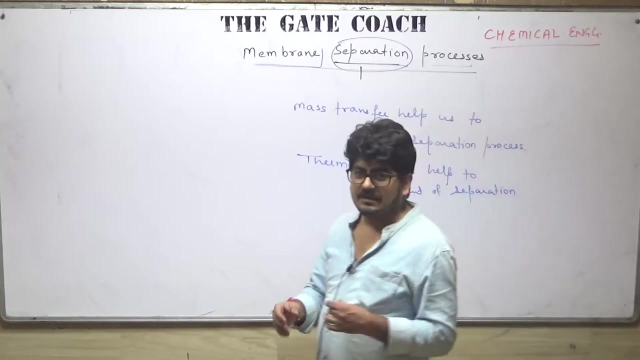 nothing to do with that subject as such directly. okay, but still many people say so. you are a chemical engineer, you must be good in chemistry. so what is the difference? what is the role of a chemist and what is the role of a chemical engineer in separation processes, in a industry, in mass transfer or in general? 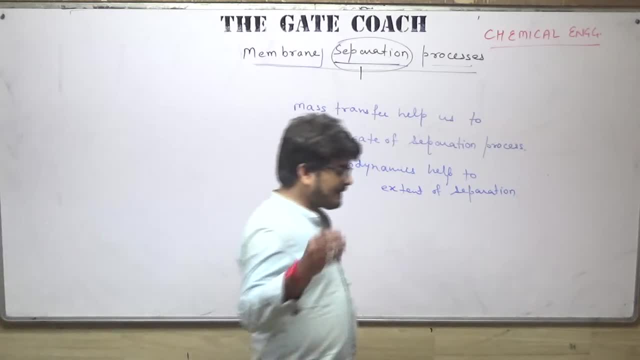 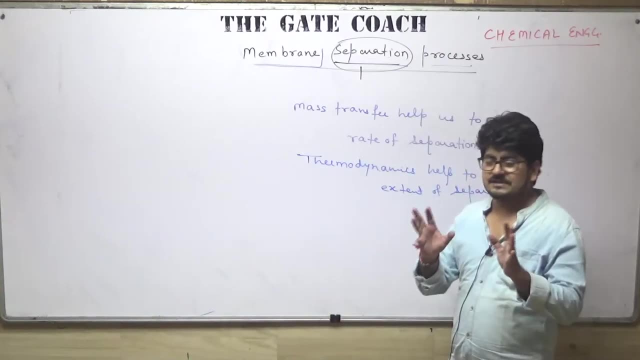 whatever you say, okay, I don't want to discuss that, I'm just telling you the answer. you can note down that or, if you want, you can see chemists, people are basically work inside a laboratory on a small scale. so, for example, you have a computer, you're the guest here, say, at a library. it can say 100 pcs per Everyday. 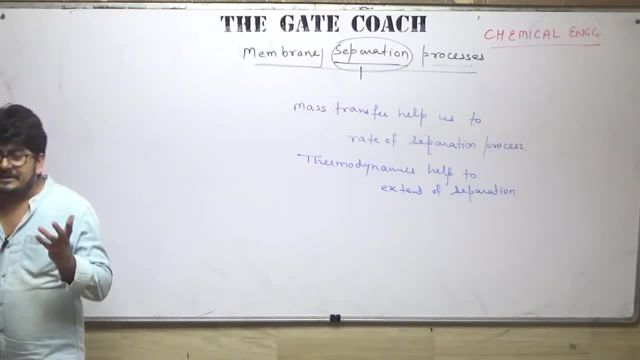 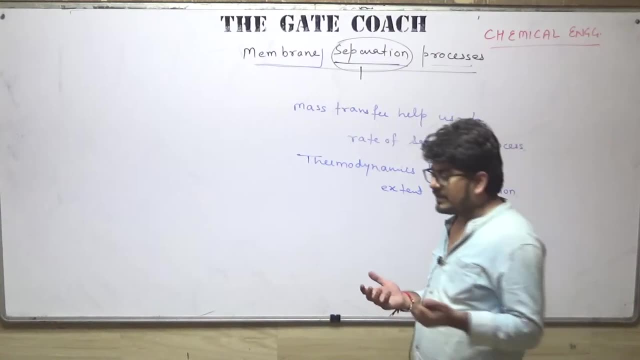 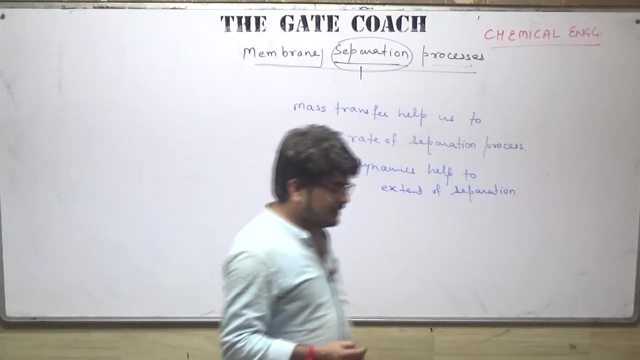 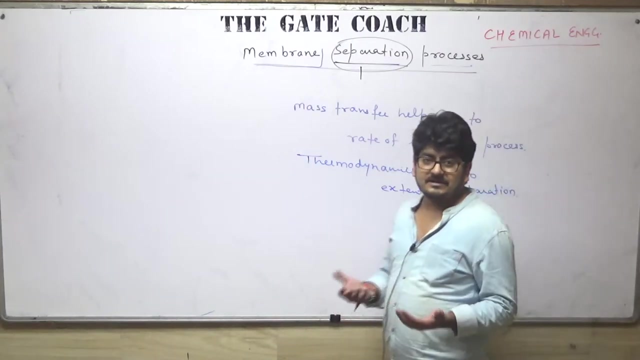 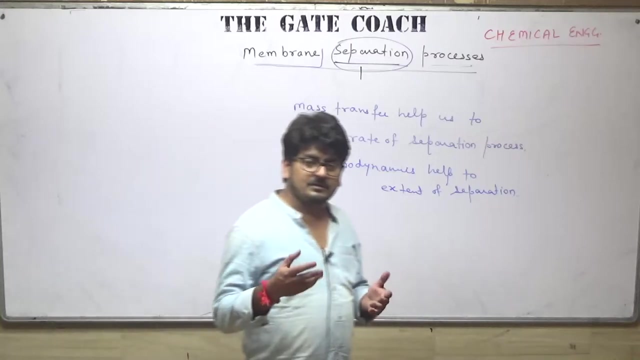 scale basis, they find out the analytical methods, the techniques for the separation, the suitable conditions for the separation. okay, for example, if i talk about the hydrocarbons, light hydrocarbons. so chemist people inside a laboratory on a small scale use chromatography methods to separate the light hydrocarbons to find out the composition of constituents. 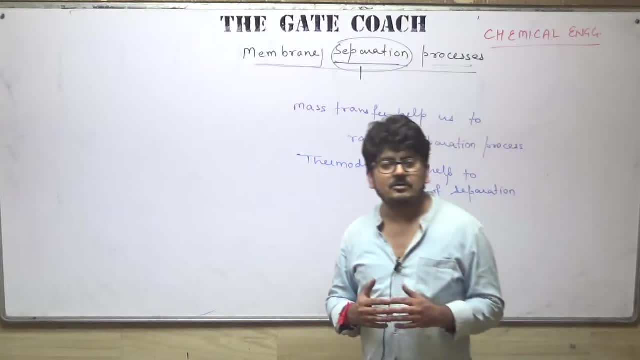 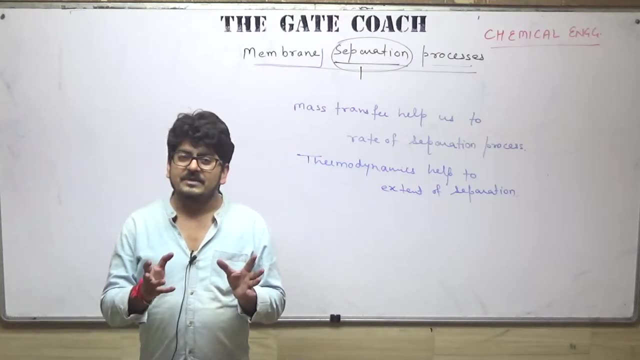 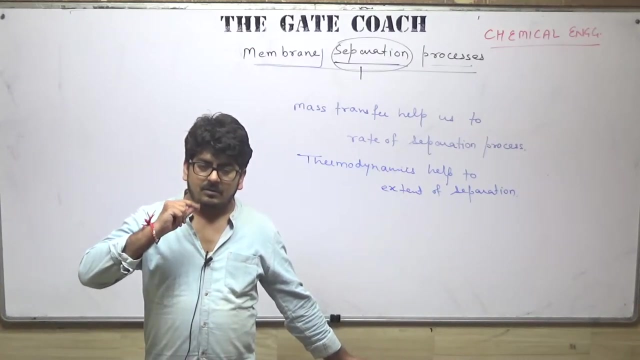 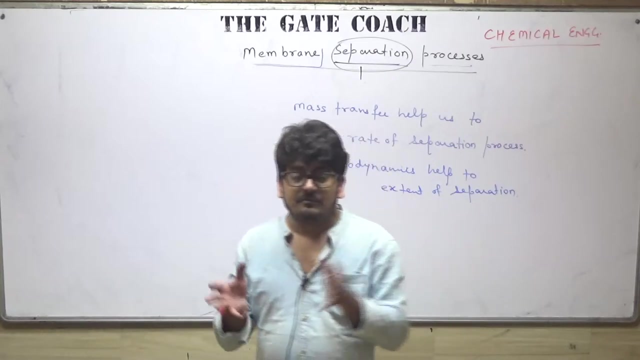 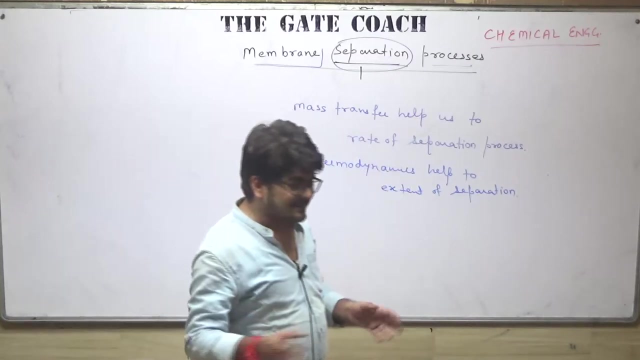 in light hydrocarbons, while if i talk about a chemical engineer, so chemical engineer, the role of a chemical engineer is to make everything commercially on a large scale. okay, if you have anything like there are so many researchers, scientists, nowadays working on the corona vaccine, okay, vaccine which we can use for the covid 19 pandemic and for all these virus and all. 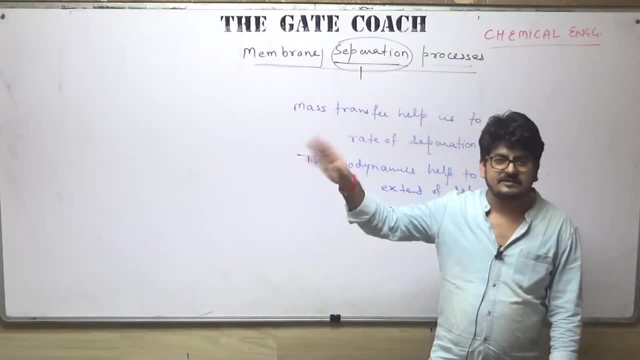 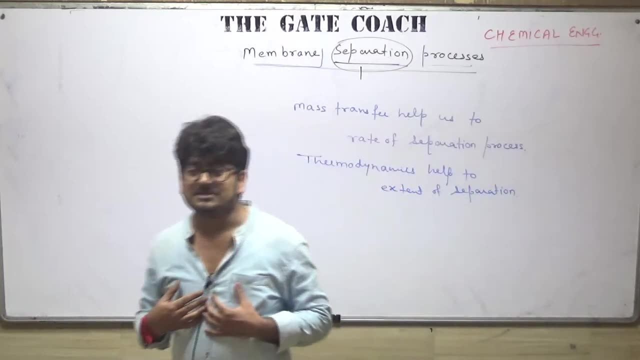 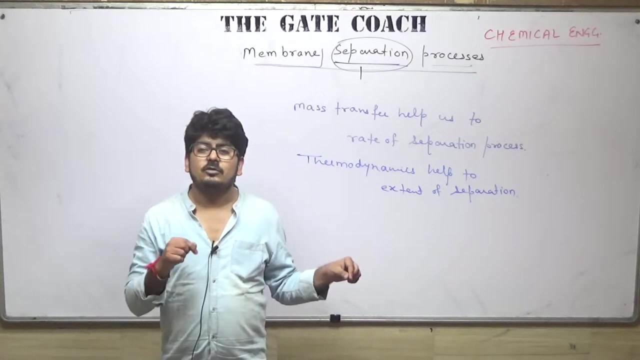 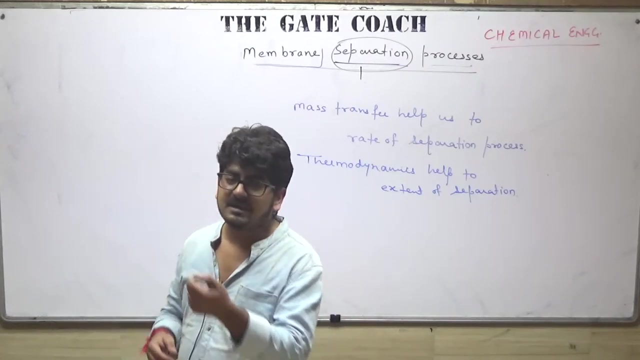 this stuff? okay, do chemist people, researchers are doing that. but when the method will be developed, when we will have the that vaccine? so, as a chemical engineer, what will be our role? our role is not to develop that vaccine at our home or in a laboratory. our role is to provide commercial value to that vaccine so that a normal middle class 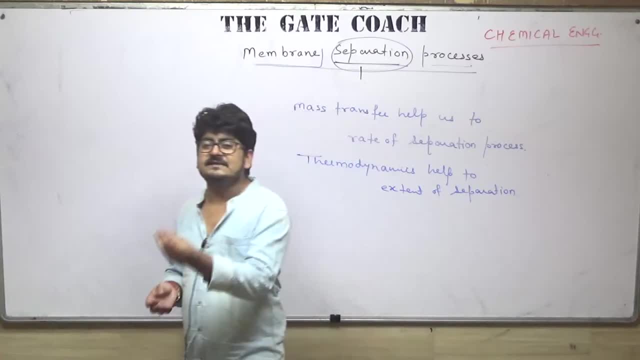 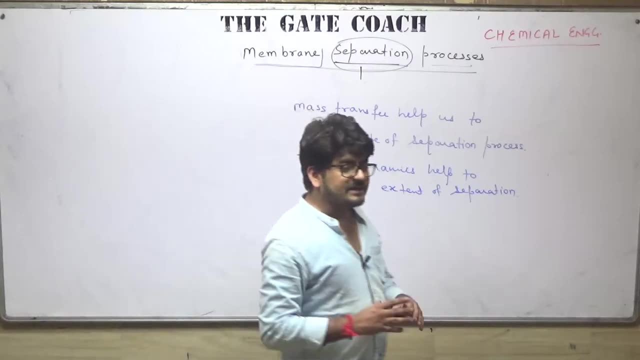 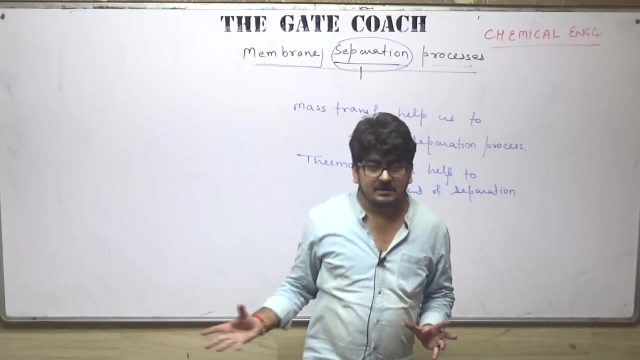 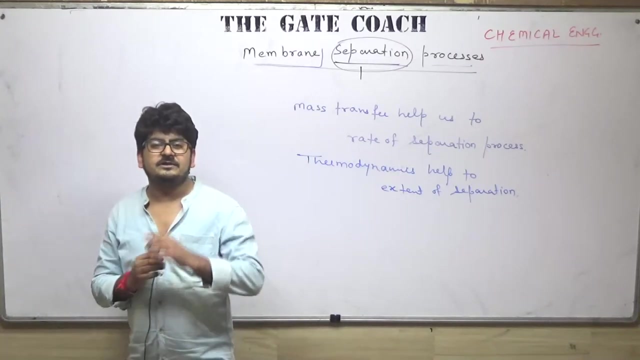 poor class, lower class, upper class, any person can easily buy, easily use that vaccine for themselves, okay. so for that we set up the industry, we set up a plant, we scale up the process, okay, like if i talk about the light hydrocarbons. so for light hydrocarbon separation we don't go with chromatography as a chemical engineer, what we do. 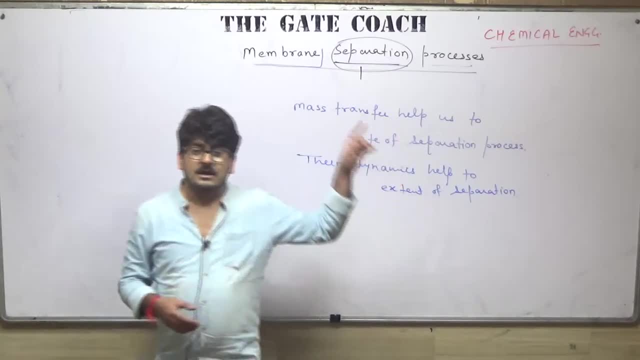 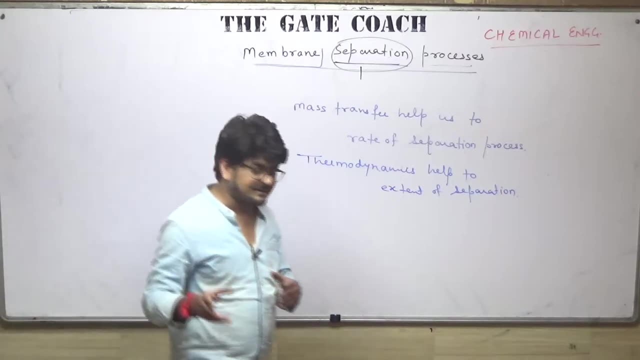 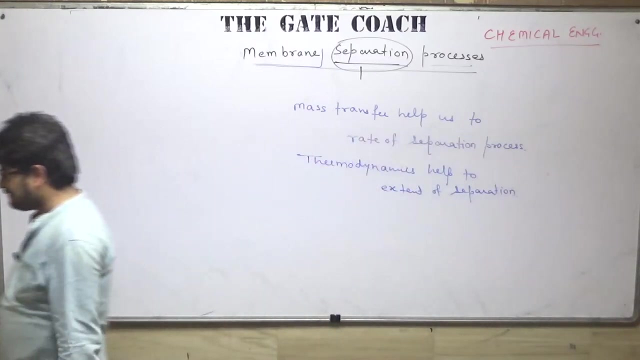 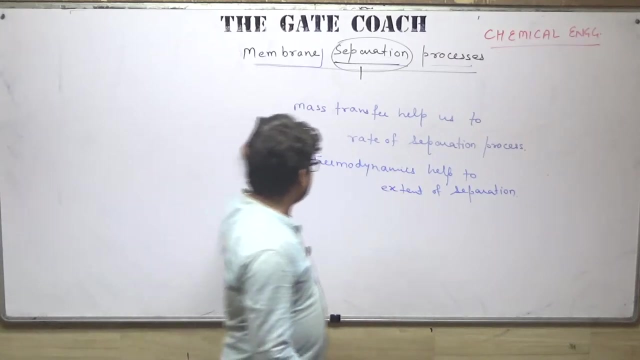 we set up an industry where we use the distillation columns, fractionating columns, for the separation of light hydrocarbons. so i hope now you can understand the difference between a chemist and a chemical engineer. yes, optimum and economical. okay, guys. so this is something about the separation process. now let's talk about the membrane separation process. 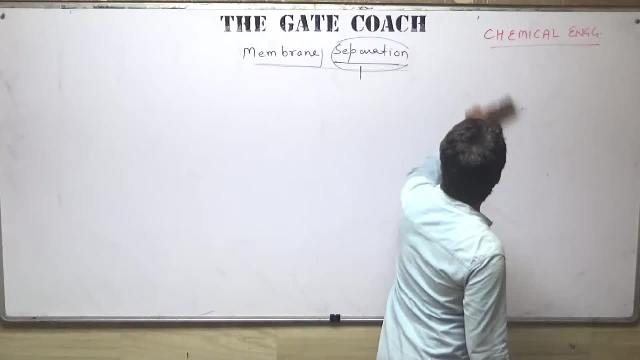 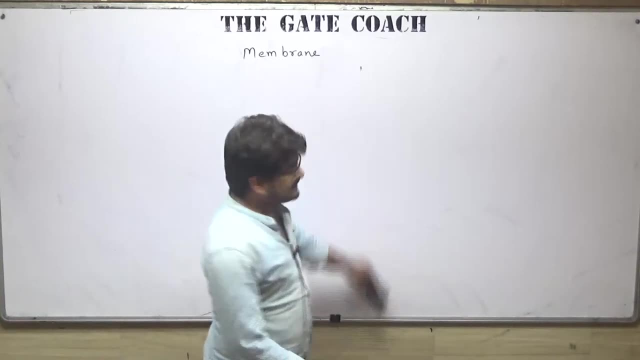 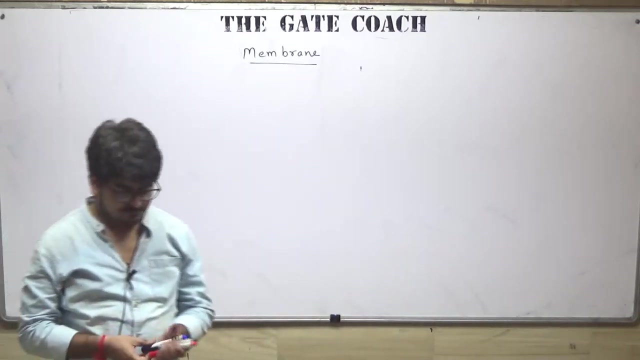 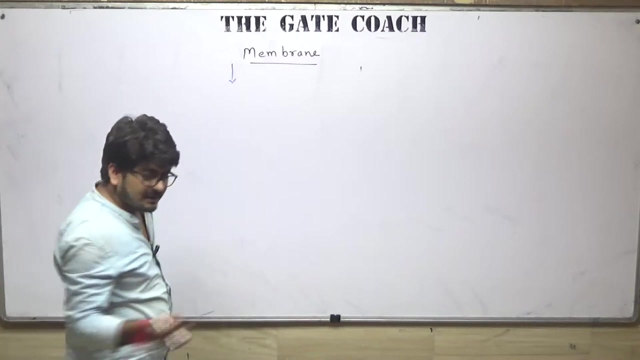 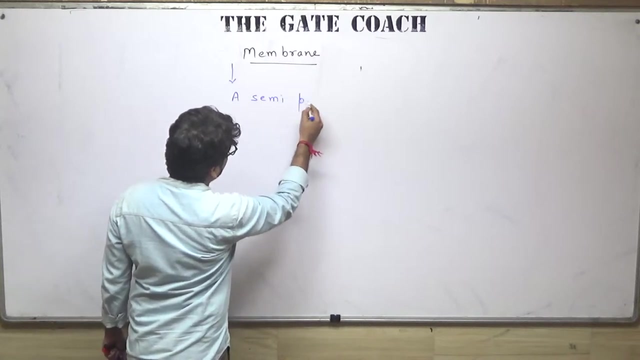 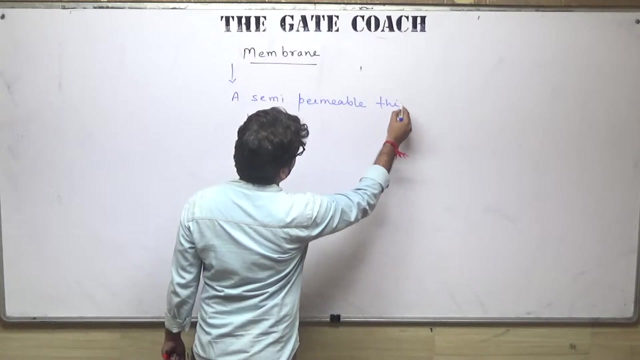 what is the membrane? what is the membrane separation? so first we will talk about the membrane. okay, so what is a membrane? a membrane? you must have known that it is a semi-permeable barrier, semi-permeable thin barrier which is used for the separation. okay, 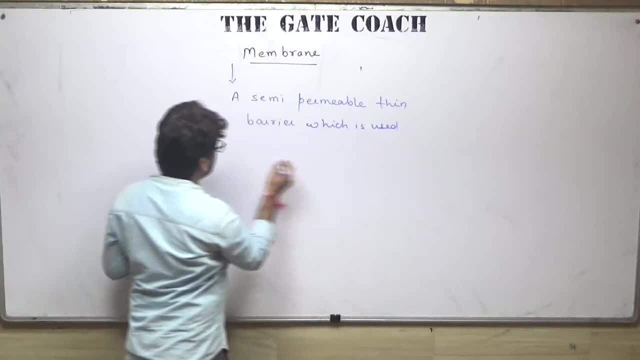 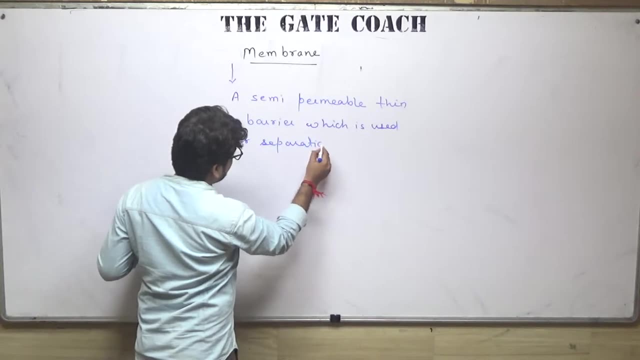 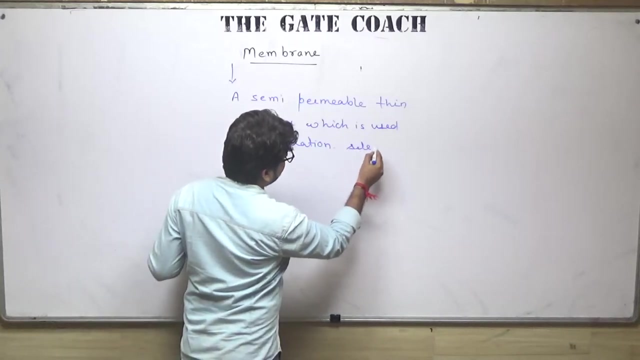 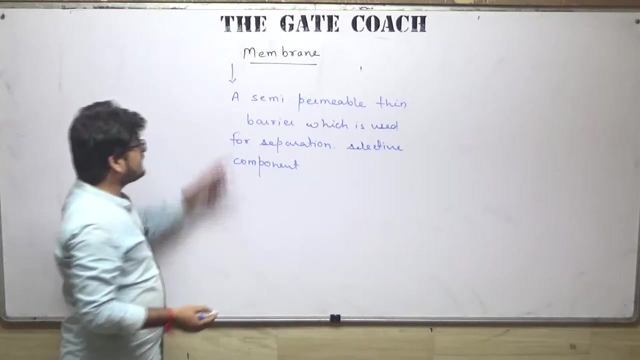 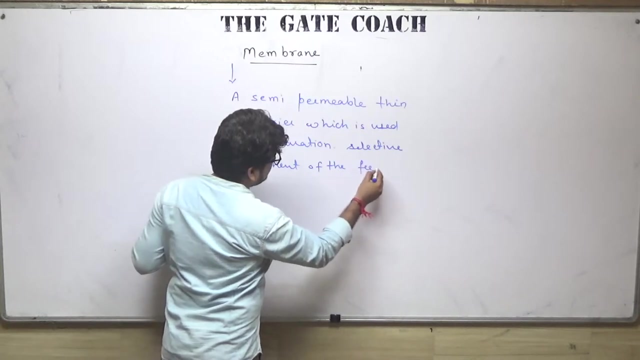 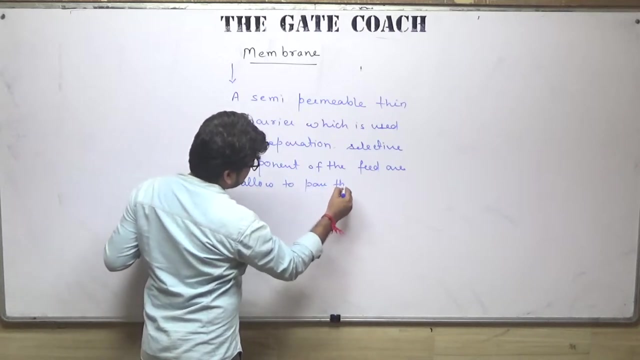 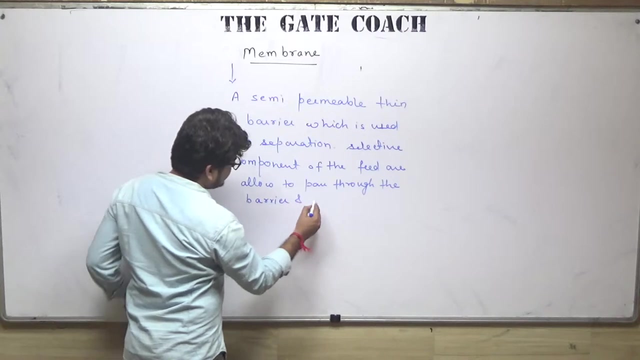 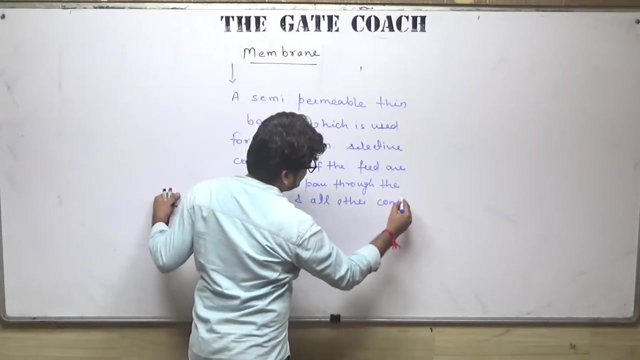 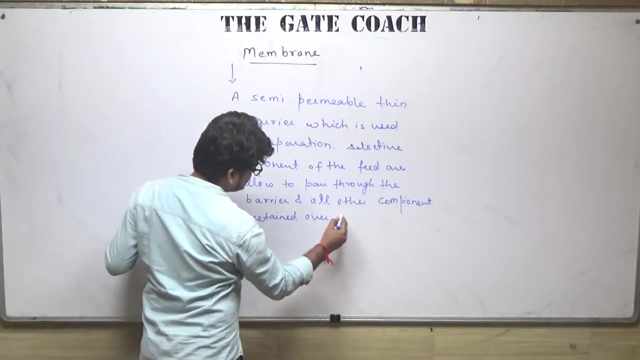 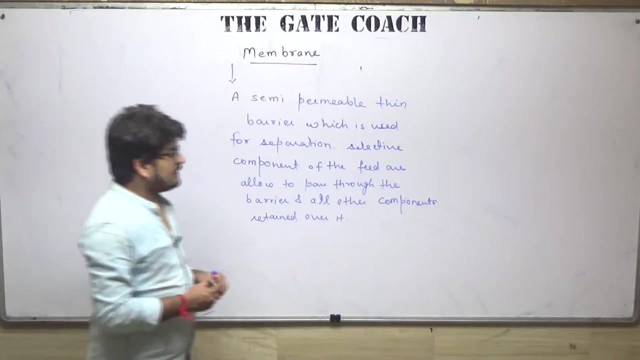 which is used for separation, how the separation takes place here. the selective component of the mixture means of the feed, or you can say molecules are allowed to pass through the barrier and all other, all other constituents or components retained over it. okay means we have a barrier, let's say membrane. 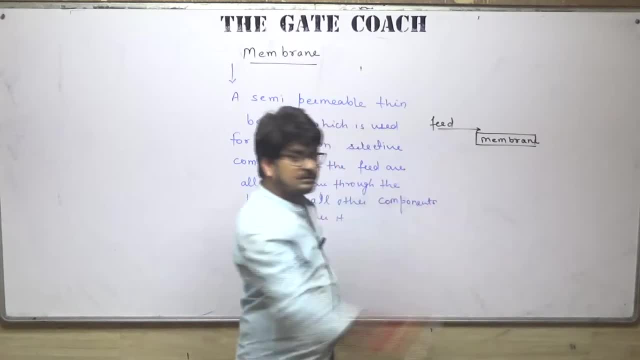 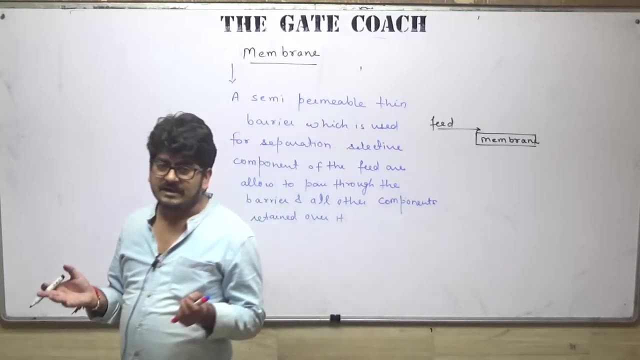 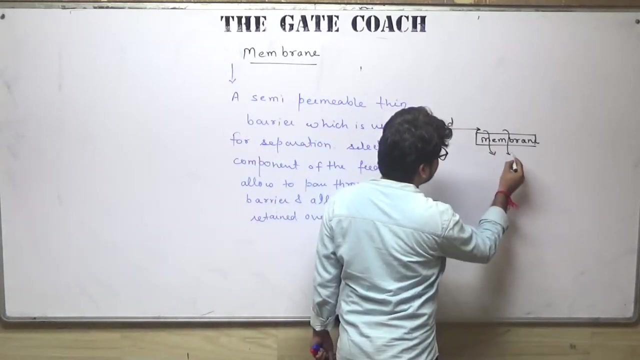 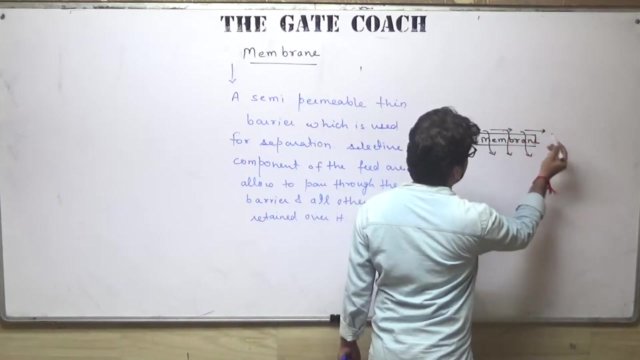 where we send the feed. and when feed moves through the barrier, through the membrane, then out of all the components which are present in the feed, only selective components will be allowed to pass through this membrane and all other components will remain inside the feed and they will leave as the residue. 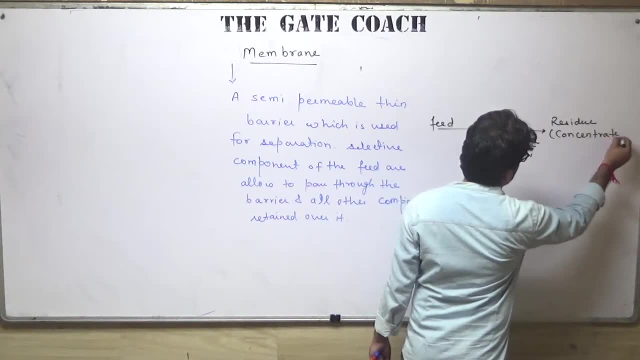 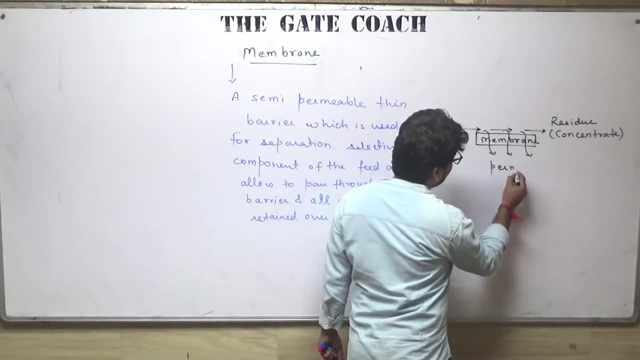 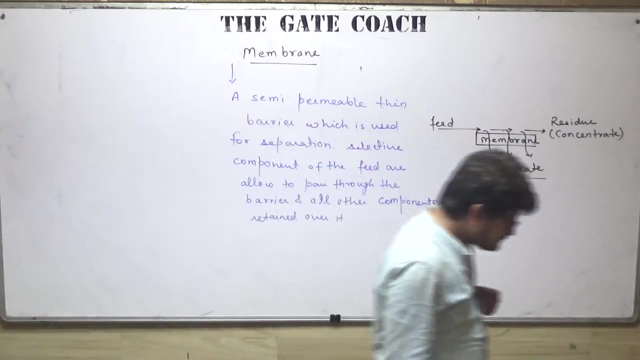 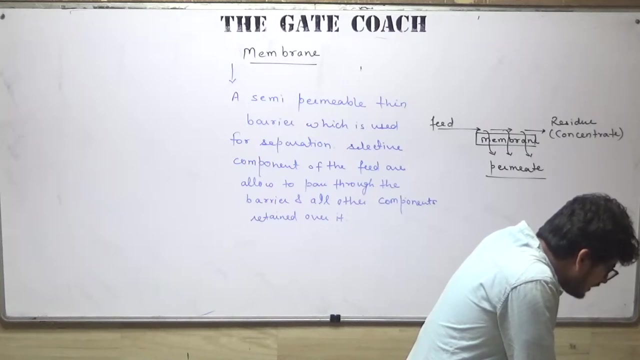 can be called as concentrate and the part which was allowed to pass through the membrane is called permeate- permeate on the inside of the membrane. so on the inside of the membrane, aátm indicating susil will be applied. in thehip to the membrane there is a 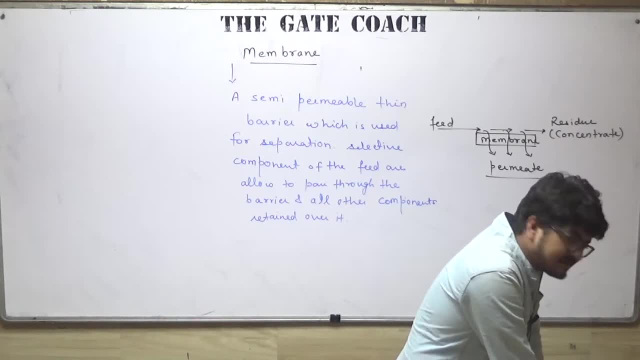 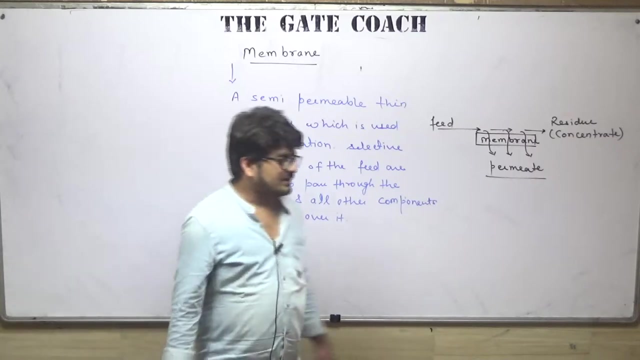 a t and we see the safetyly in this way, which is very devein, or the way closer to the surface of a soil. that's how it is separated from the membrane. we think that's how it works. semi-permeable membrane is just like our skin- yeah, I was about to say that- okay. or, for example, 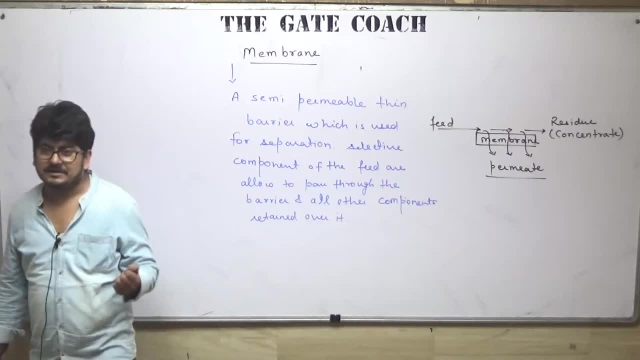 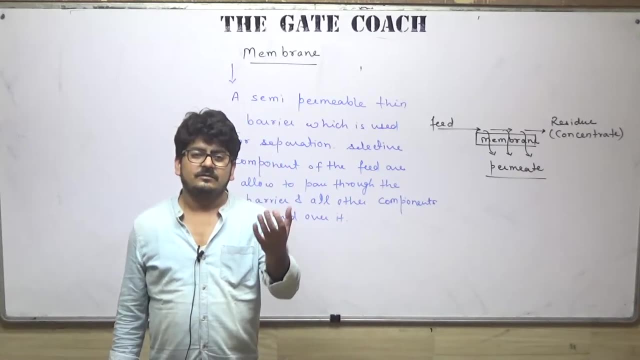 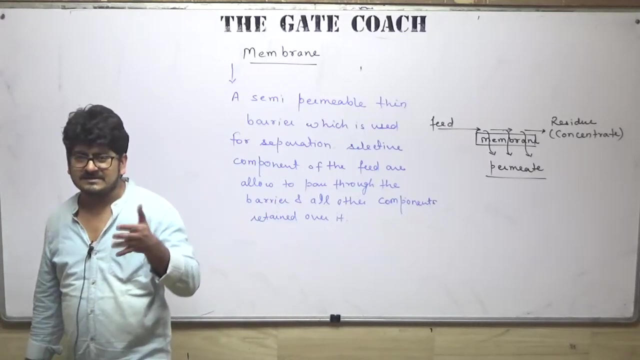 you can say kidney as well. kidney is also like a membrane in our body. we know kidney used to separate the waste water, the waste products, from the bloods. okay, but it is not separating the hemoglobin or the Rh factor, whatever the things are there in our blood. I don't know the name, sorry. 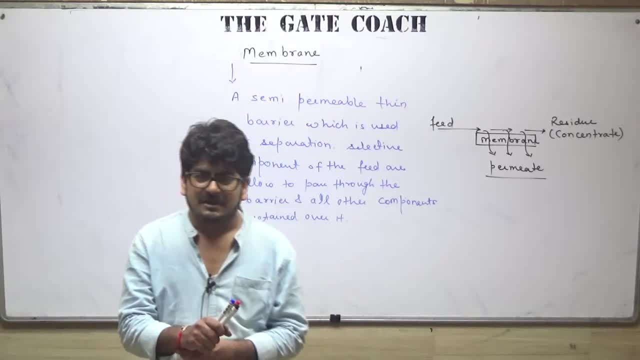 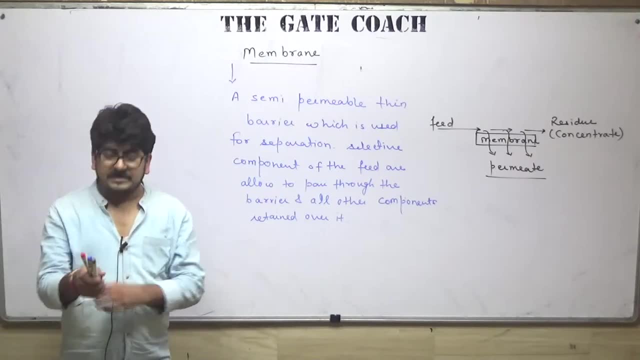 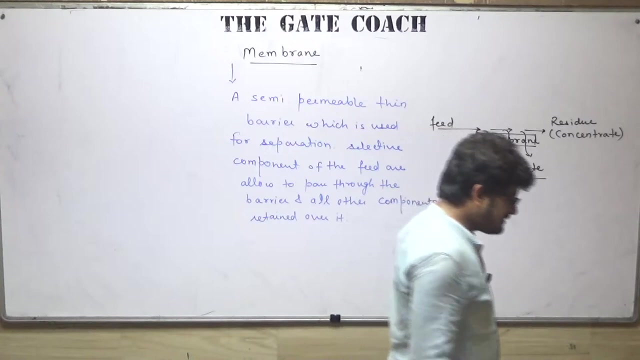 but I hope all of you know that. the W TLC factors. what are those things? WBC, RBC, all those things. so plasma. so kidney does not separate that thing from the blood, it only separates the waste water, the waste products of the metabolism. okay, thought of osmosis ones. 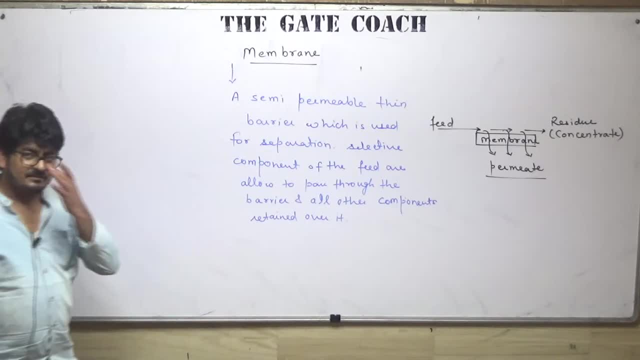 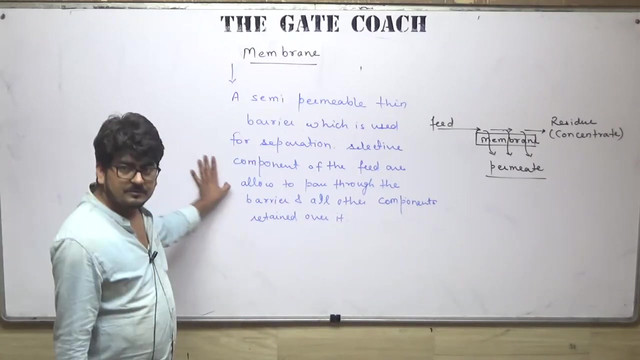 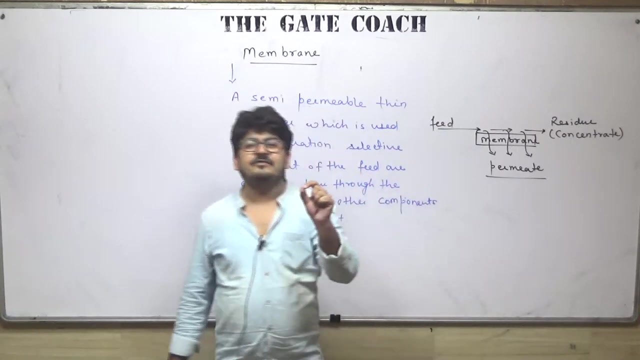 osmosis also comes in the same category, but we will see to it. okay, so, guys, this is membrane. now let's talk about the material of membrane, or basically the classification of membrane. I hope it is clear to you what is the role of a membrane membrane. do feed pass through the membrane? only selective components, selective molecules from the 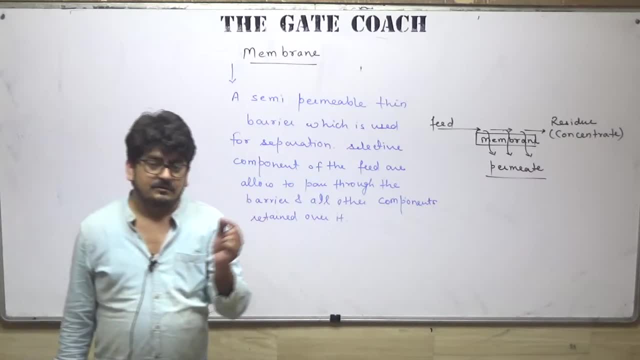 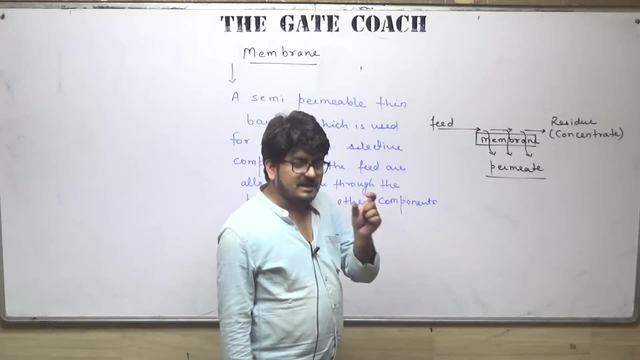 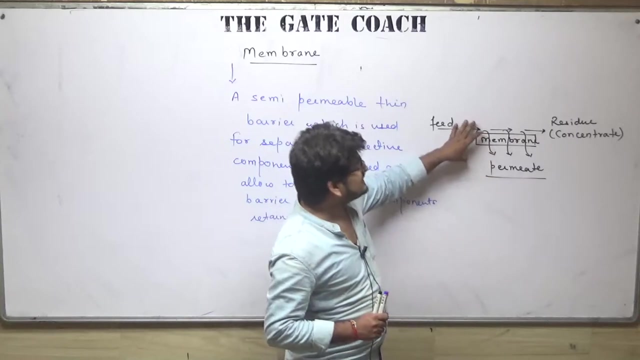 feed are allowed to pass through the feed. sorry, to pass through the membrane, to pass through the barrier. okay, some of our selective means specific components which will pass through the membrane. the rest of the components which are in the feed will remain as it is okay, and the components which 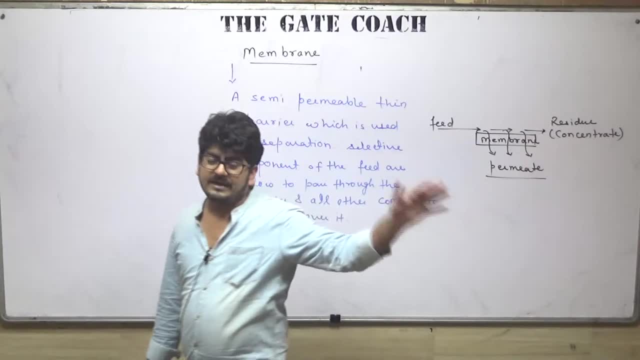 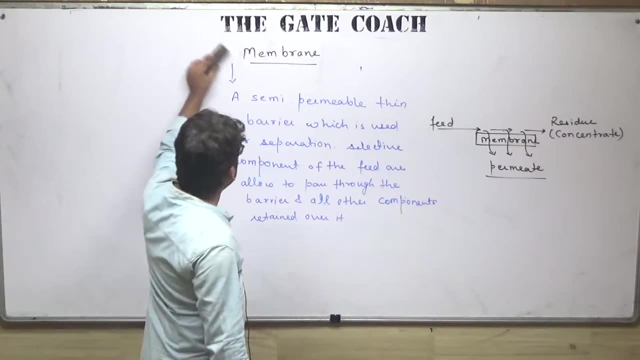 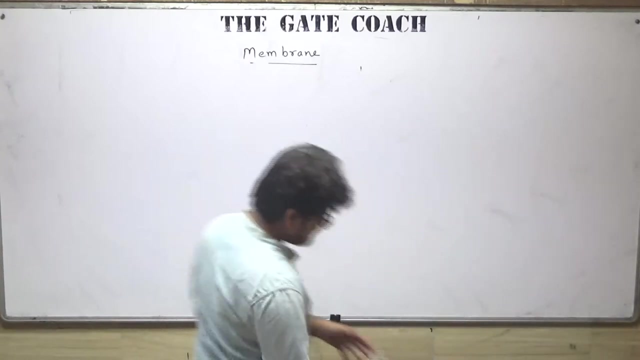 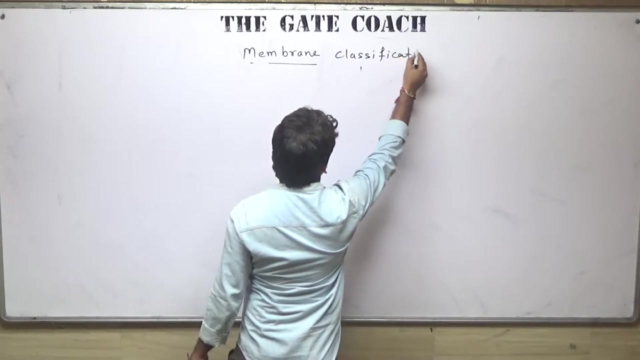 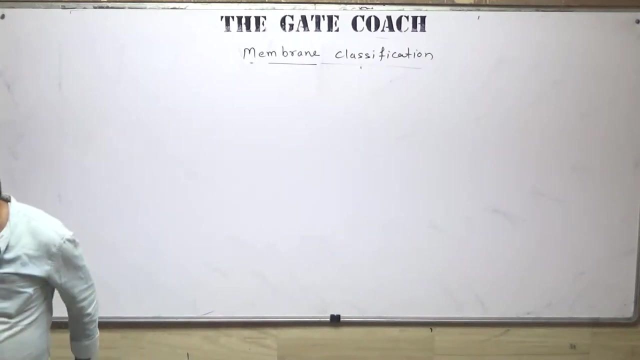 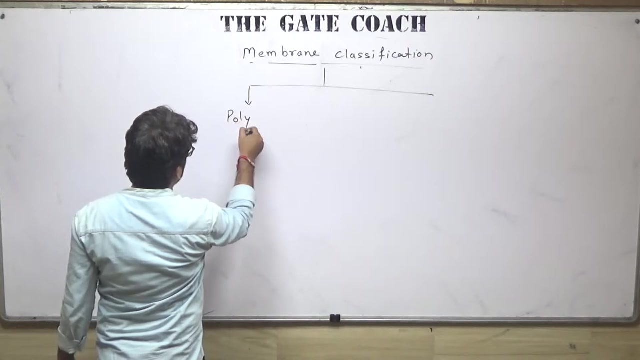 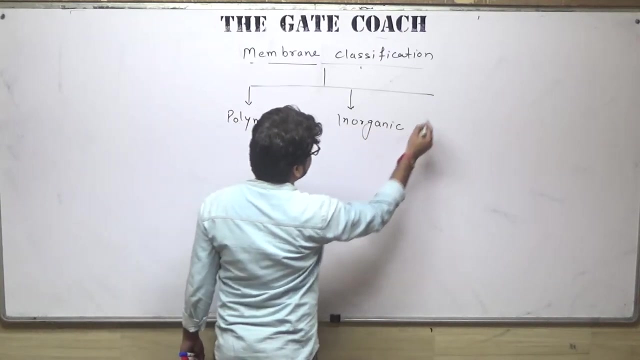 concentrate, residue, retentate- okay. and the part which is allowed to pass through the membrane, that is called permeate- okay. so now, guys, let's talk about the classification of membrane. membrane classification: a membrane can be classified into three categories. first is polymer. second is inorganic. 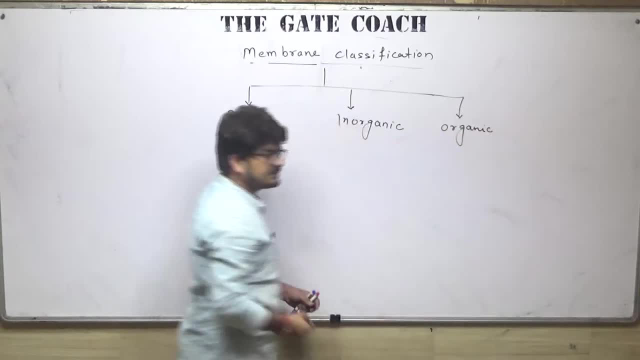 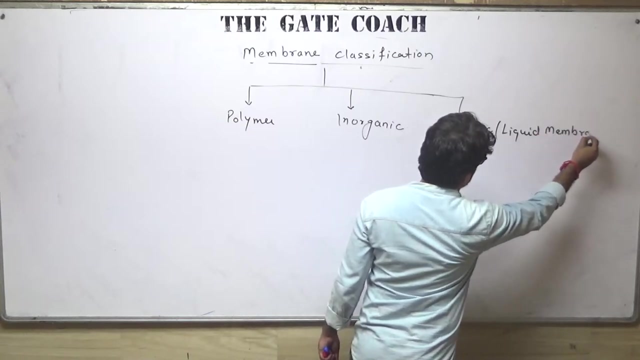 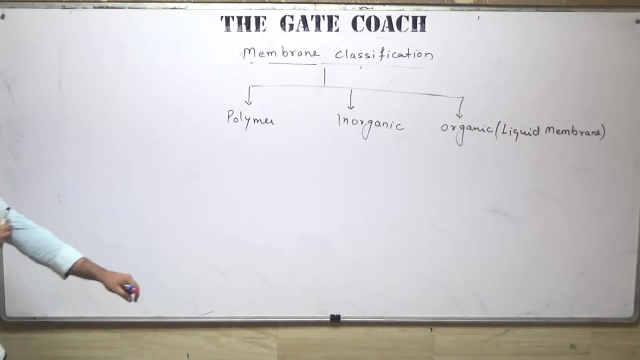 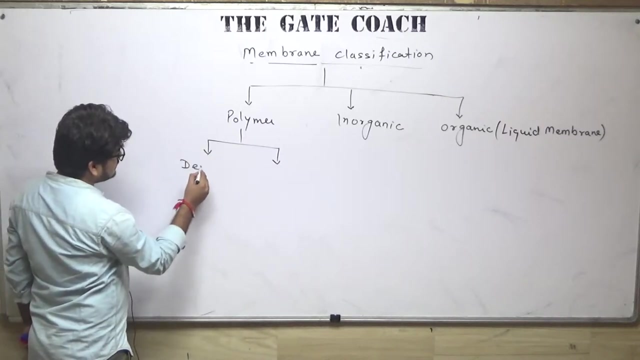 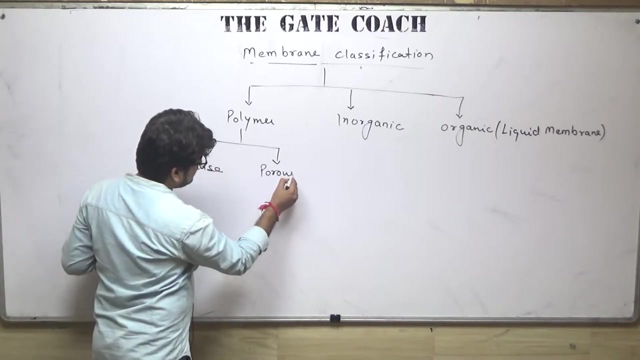 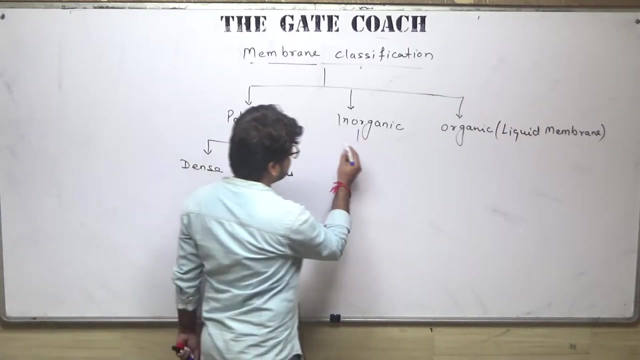 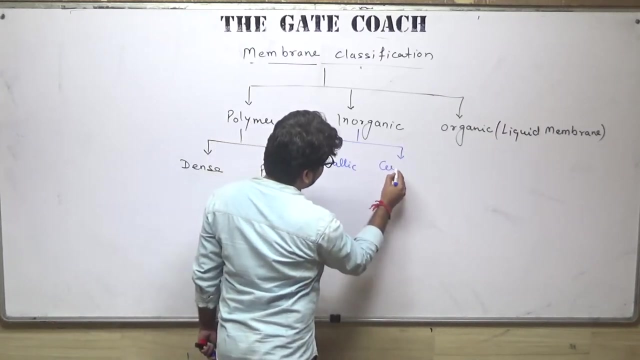 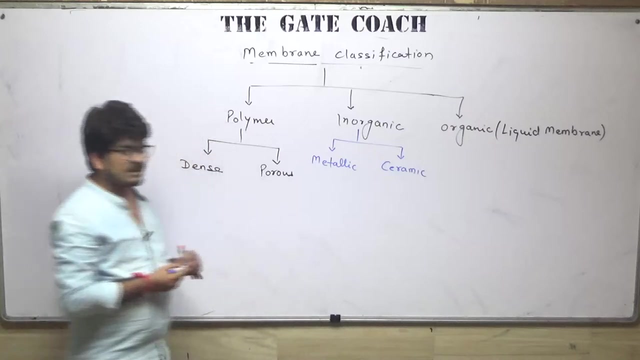 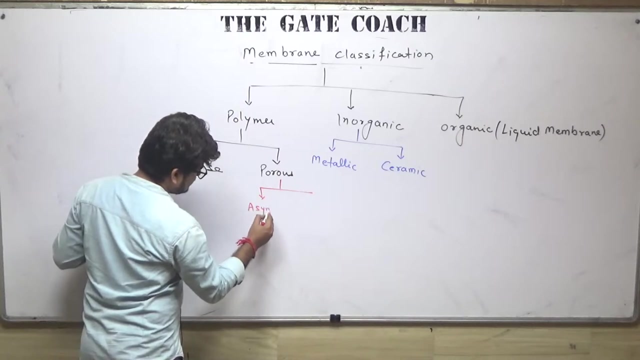 and third is organic, and here organic membranes are also known as liquid membranes. okay, the polymer membranes further can be classified into two categories: dense and porous. The inorganic membranes can be classified into two categories: metallic and ceramic. Here the porous membrane can be classified further into two categories: asymmetric and 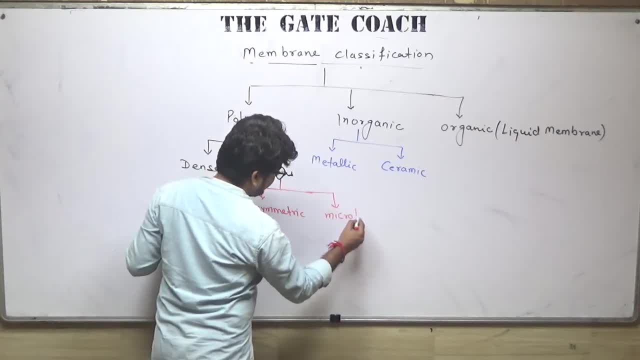 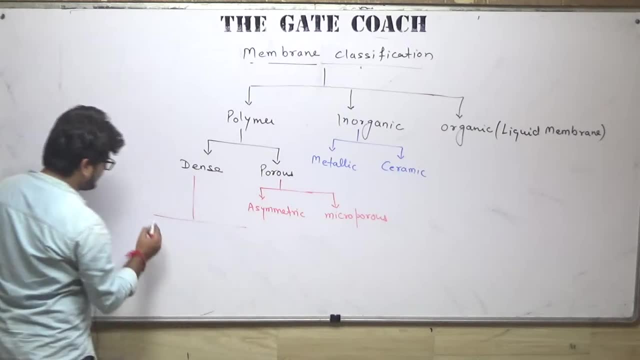 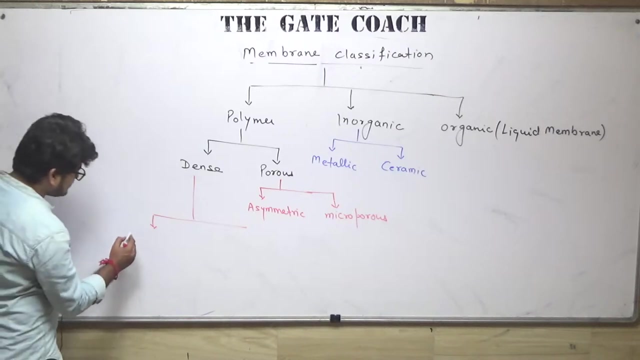 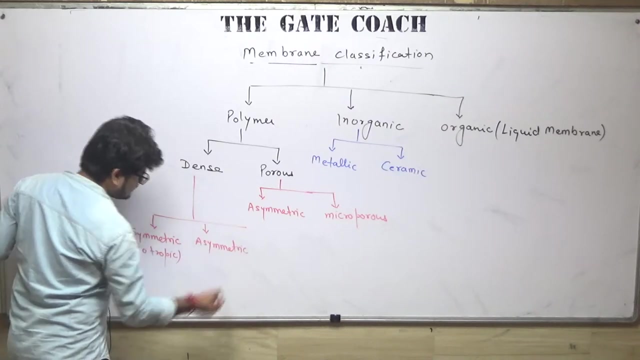 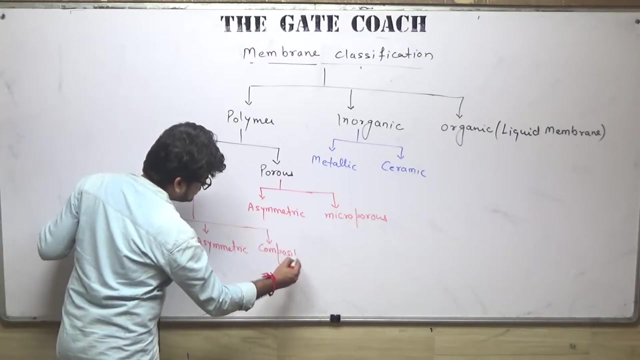 microporous, Okay, While the dense membrane, dense polymer membrane, can be classified as symmetric, also known as isotropic, asymmetric and, last, combination of these two, Composite. Okay, guys. So here we will talk about all type of these membranes. 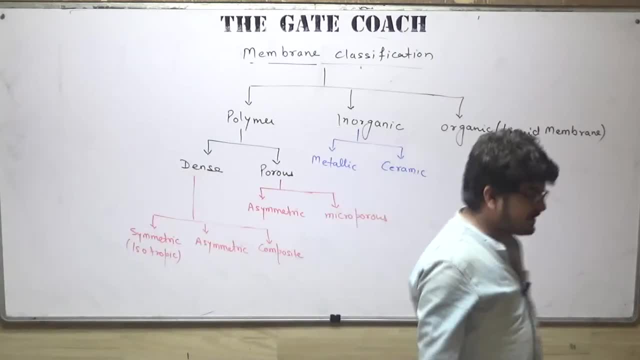 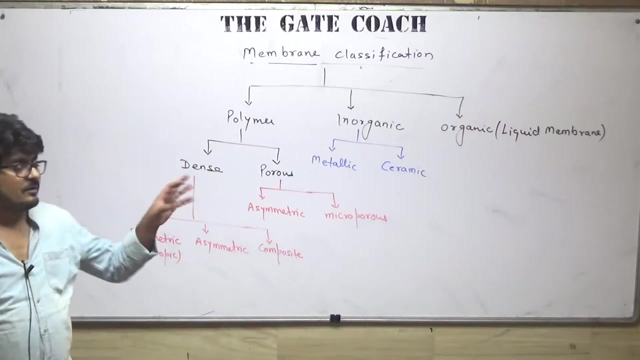 What are the materials we can use for the formation of these, manufacturing of these membranes? Okay, Which membrane has the better quality? and what are the factors we use for the membranes, for the character, for the selection of membrane, To find out the effectiveness of every membrane? 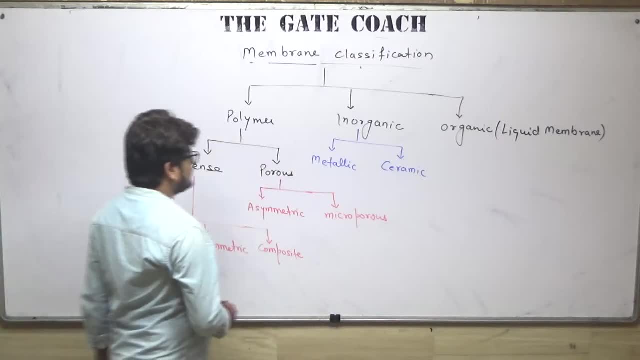 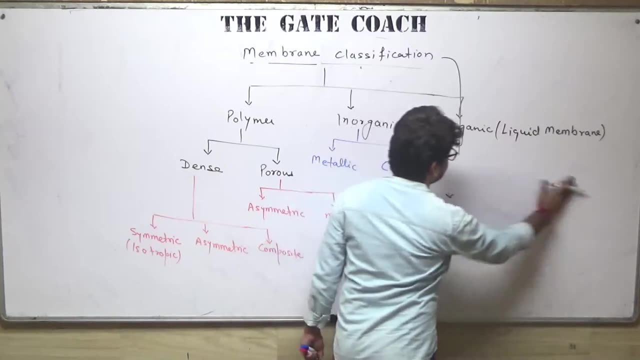 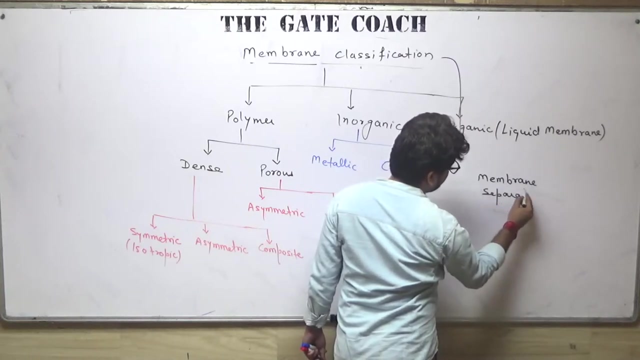 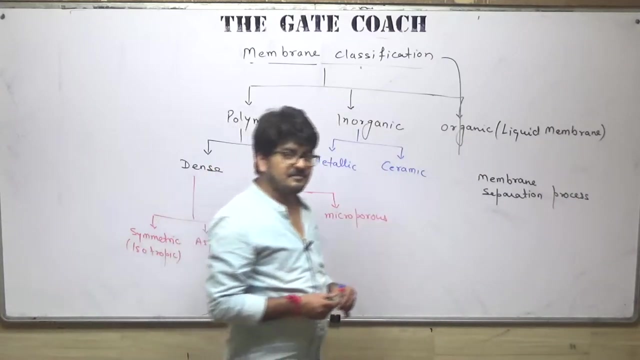 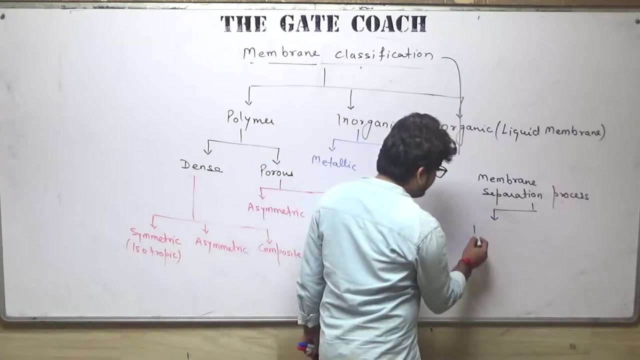 Okay, And membrane separation process. if I talk about the membrane separation process, so membrane separation process can be classified into two categories. Okay, In two ways. First, based on the pore size of the membrane. Based on the pore size of the membrane. 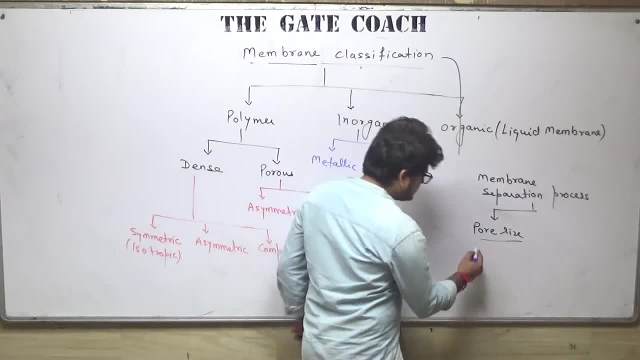 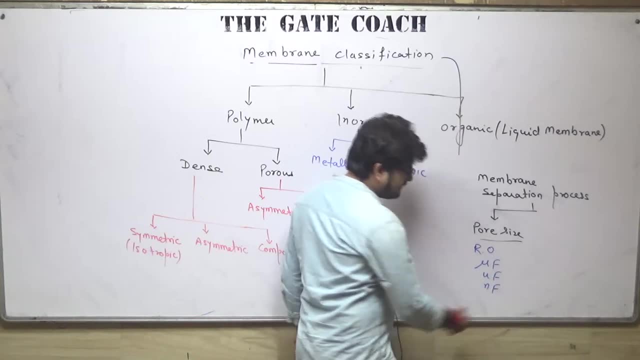 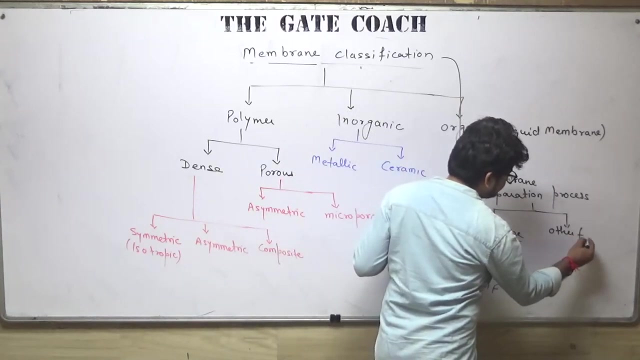 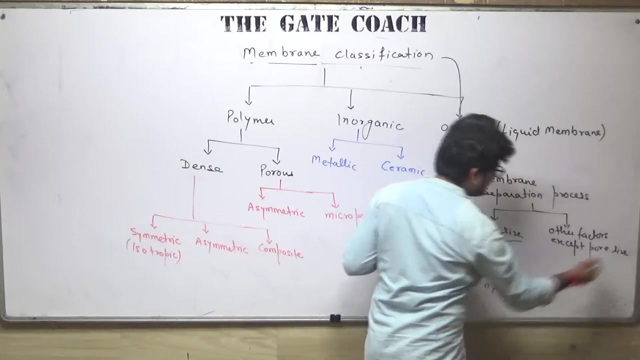 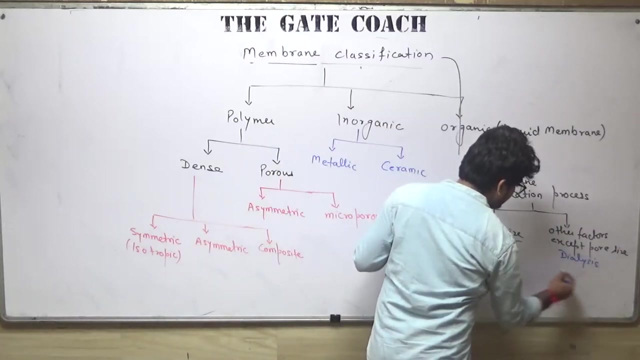 Here we have to study the reverse osmosis, microfiltration, ultrafiltration, nanofiltration, etc. The second basis is all other factors. Okay, Analyzing the pore size, Except pore size, Here the examples are like dialysis, pervaporation, etc. 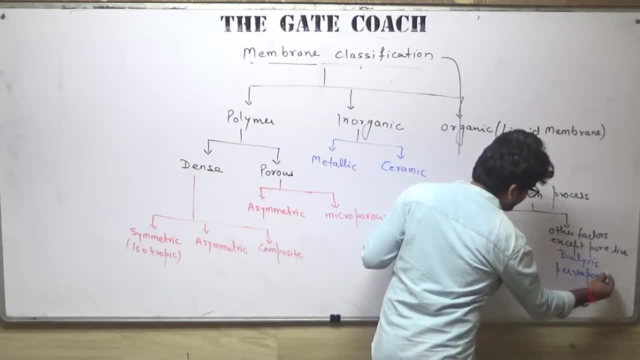 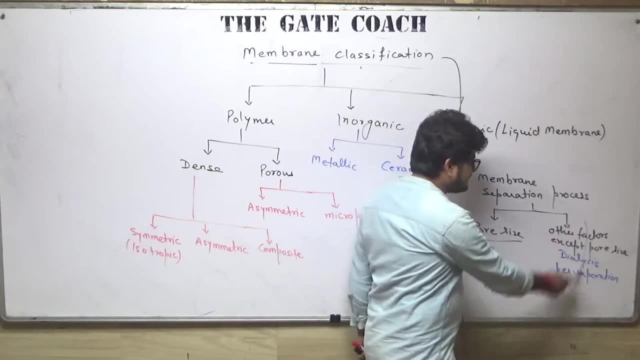 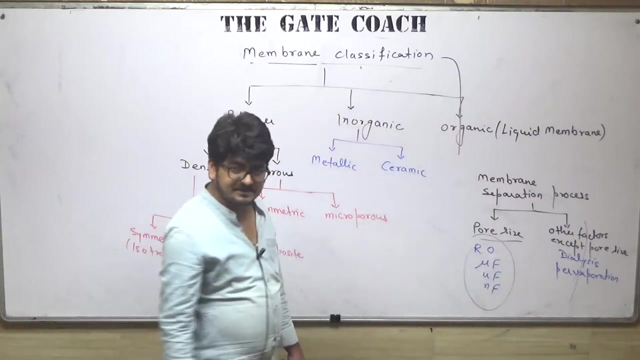 Okay, So I hope you must have studied all that thing in your BTech, But here we will not talk about any of these things, As in our syllabus it was specifically mentioned that we have to deal with these four kind of methods. 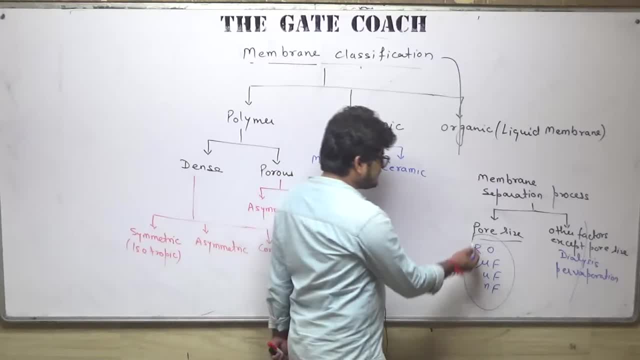 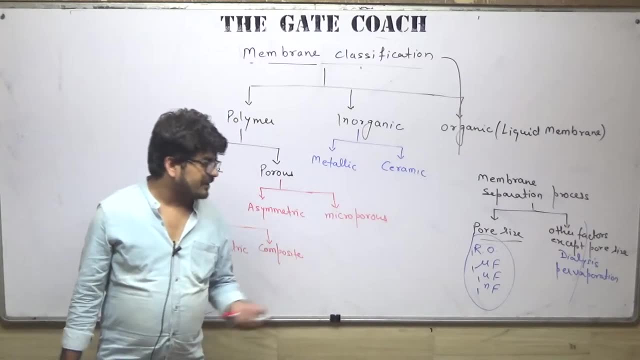 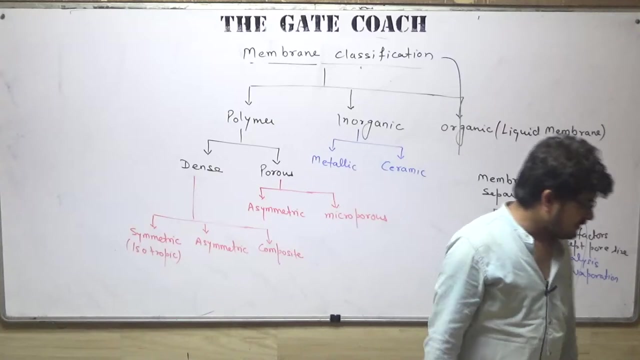 four kind of membrane suppression techniques, So we will discuss one by one for each of them, Okay: Microfiltration, ultrafiltration, nanofiltration and reverse osmosis based on the pore size. So, guys, this is all for the day, as we can have only one hour live class daily. 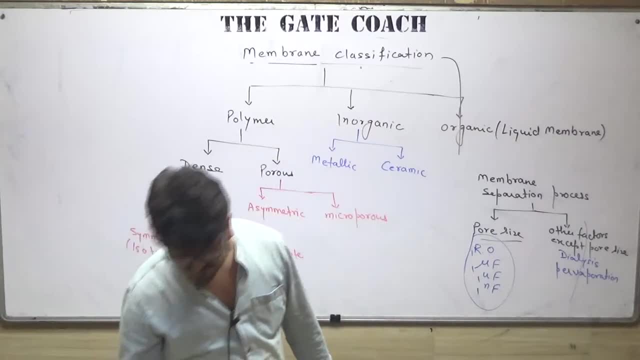 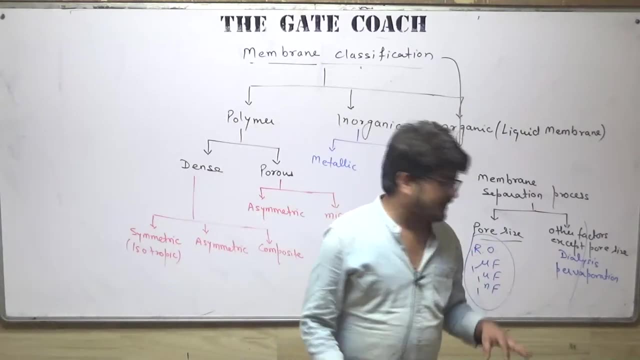 as we already have some classes in our coaching as well, And test days are going on. So many things are to do, So I hope we will be able to complete the syllabus on time in the next week only, So next class will be on Monday. 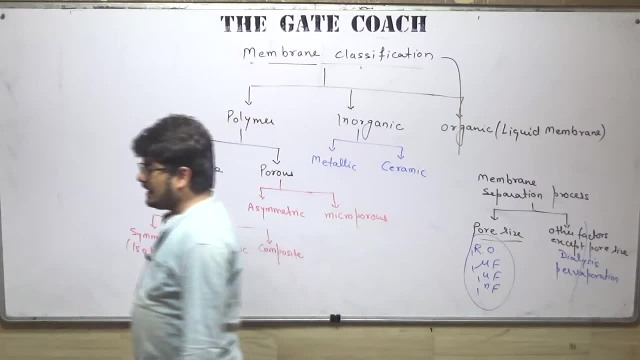 You can check the schedule on our Facebook page. Okay, The timing will be same. Most probably the timing will be same: 4 pm in evening. Okay, Every day. That will be helpful for all of you and for all of us. 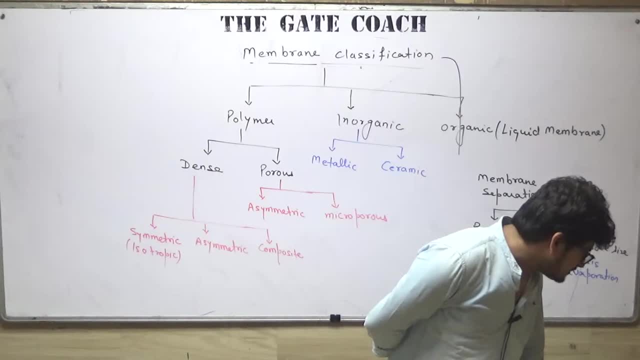 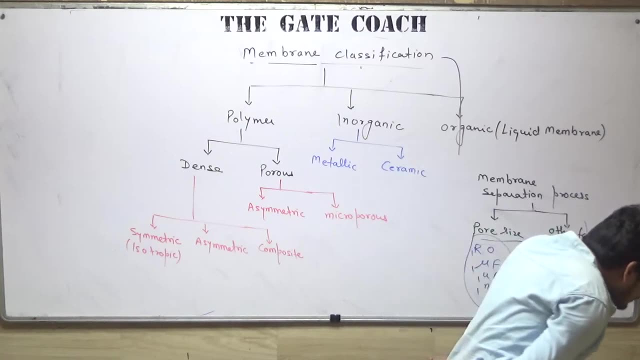 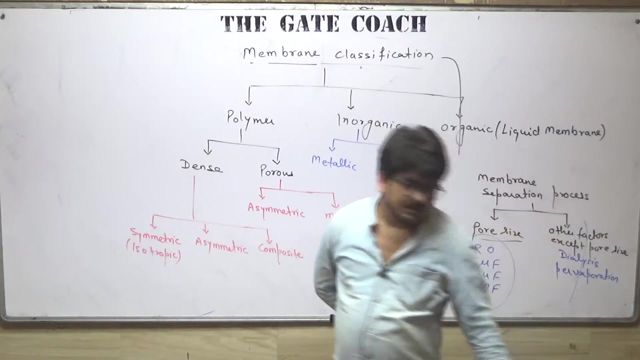 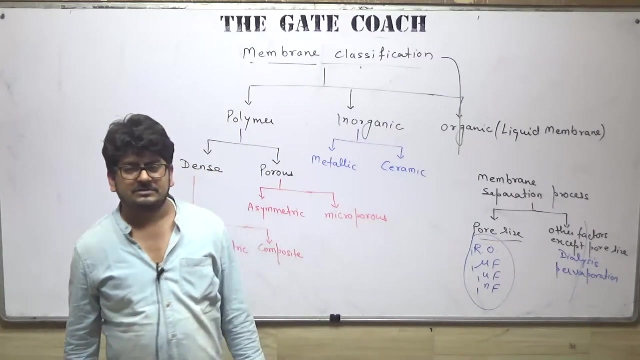 Sir Ritik Gupta. in caustic soda plant electrolysis It is used. Please cover it quickly, Guys. we will cover all the things. Don't worry. This was the first lecture And I already told you this was the introductory lecture. 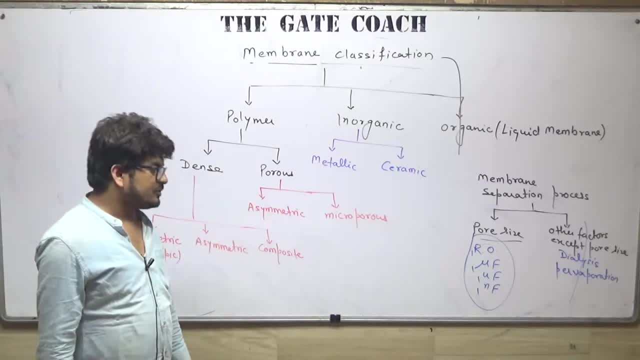 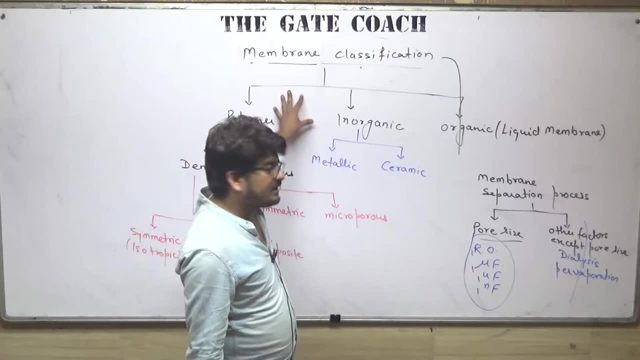 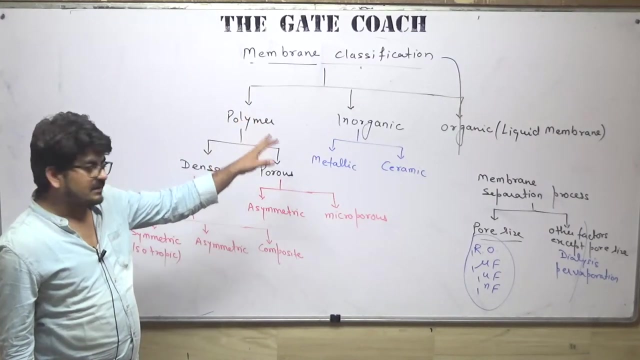 And now on, I think I have already given the introduction part. In next class, we will talk about the materials used for the membrane manufacturing, the advantages, the disadvantages, the industrial applications, as well as some of you are asking in which industries membrane separation method is used. 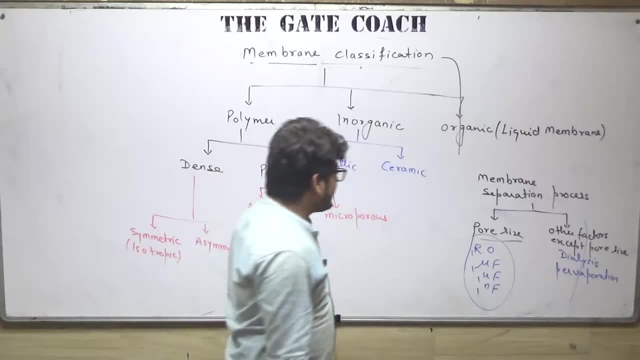 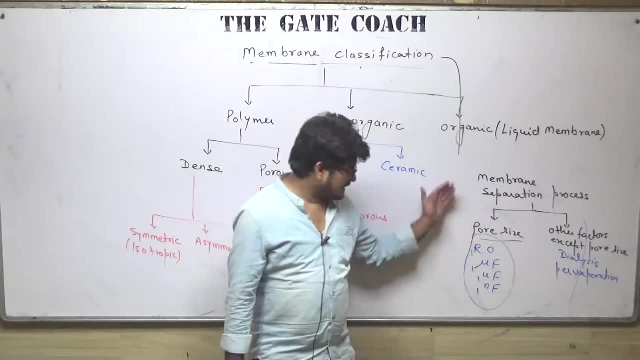 So we will discuss all that thing And, yes, after that We will talk about the membrane separation processes based on pore size, where we will discuss the microfiltration, ultrafiltration, nanofiltration and reverse osmosis. Okay, 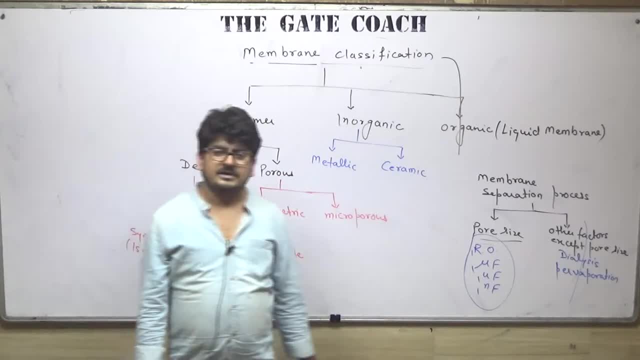 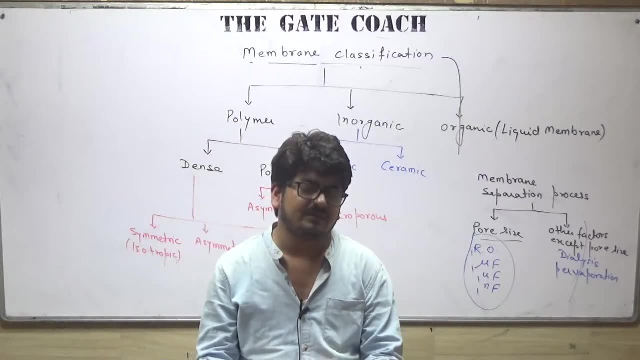 So, as per the literature, it will be covered in next four, five, three, four days at max. So next class will be on Monday, Tuesday, Wednesday and hopefully we will be able to cover the entire membrane separation part on Wednesday or Thursday. 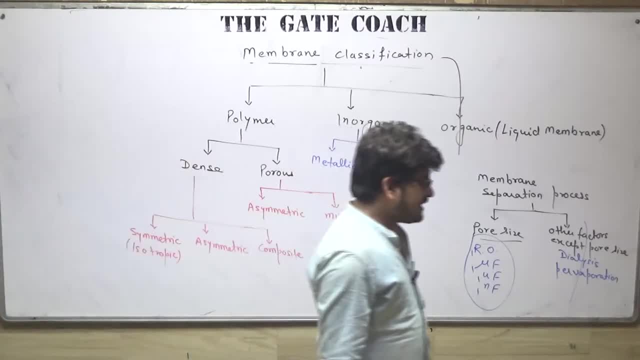 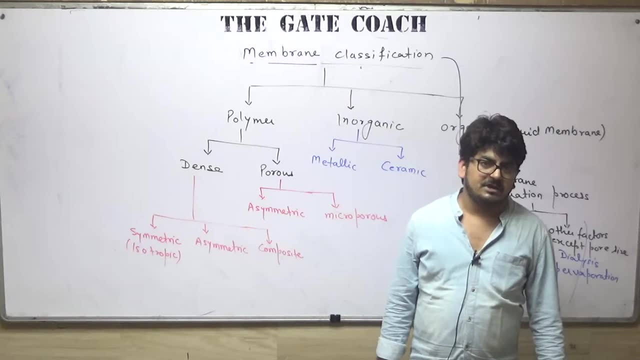 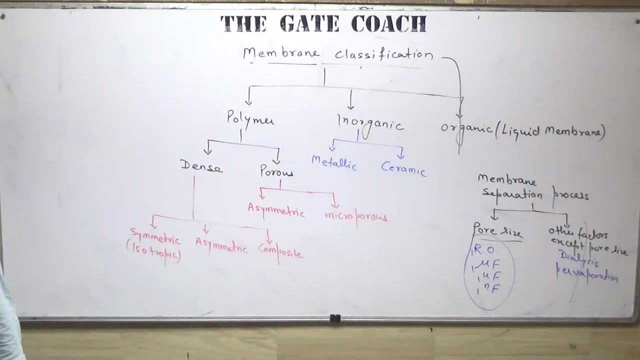 Maybe Okay, So don't worry about that, And if you are in a hurry, then I can provide you the literature, the notes, gate notes for the membrane separation, where you will find some numericals as well on the related topics. 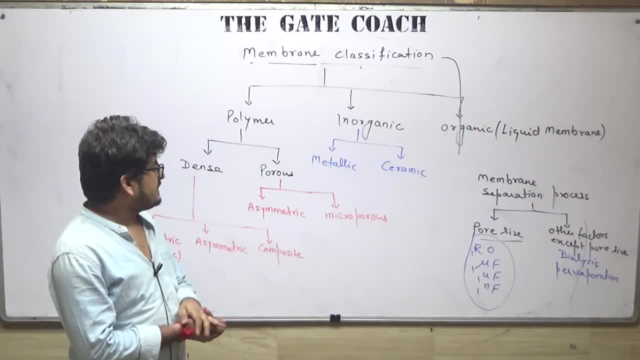 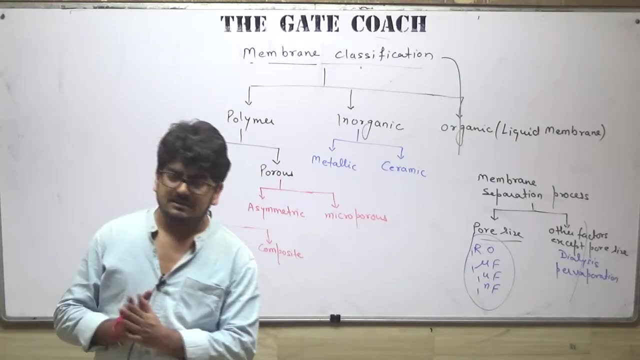 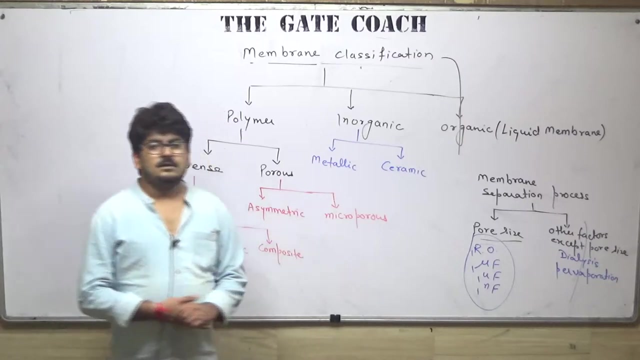 So, guys, that's all for the day. I hope it is good. as the introductory class, We have covered the sufficient part. Now we will discuss the next topics, Next part, in the second class. that will be on Monday. So till then, have a happy weekend. 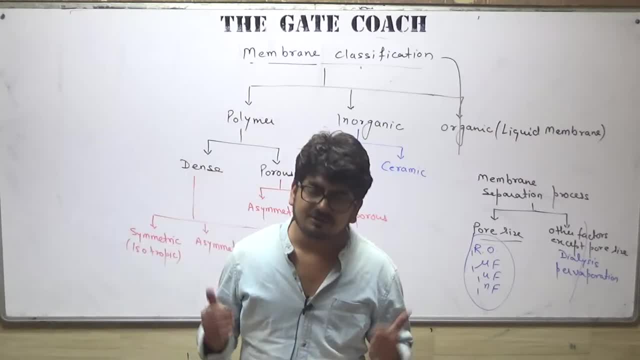 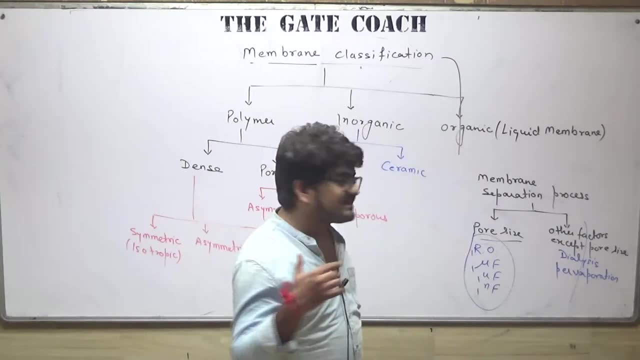 Be safe, be happy, spread happiness and wish you a very happy independence day in advance. Okay, And if you have any doubt from the today's session, then you can discuss that in the next class as well. So see you, guys. 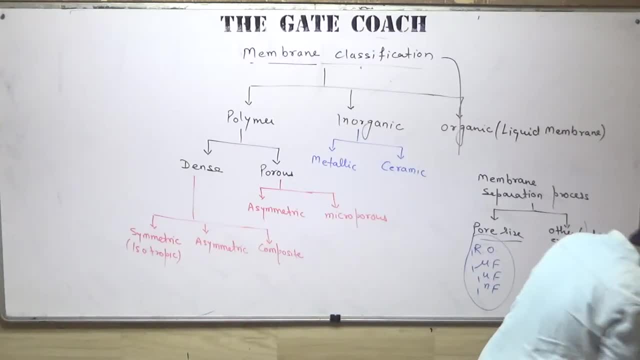 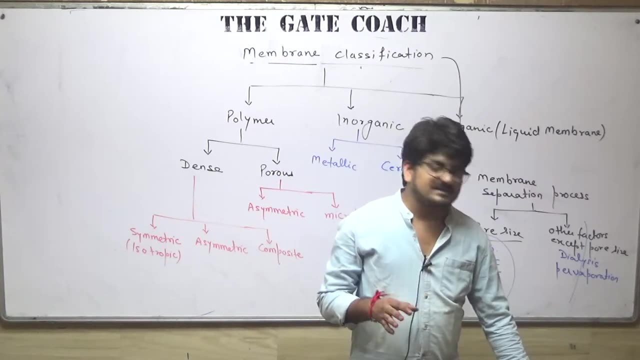 Okay, Thank you so much. Thank you for joining us Now. we'll finish, bro. That will take care of itself. the lecture With the whatnot to take this chapter are as. as such, I am not sure, but whatever literature I have studied, I told you the reference books. 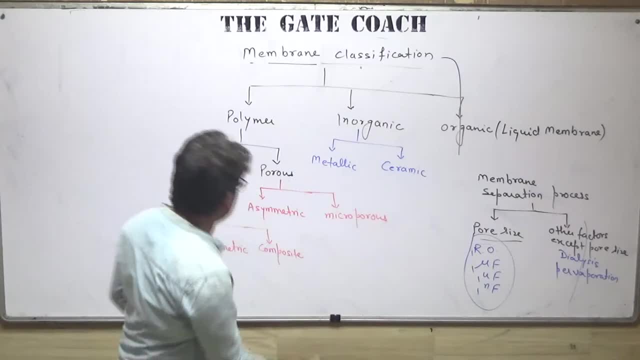 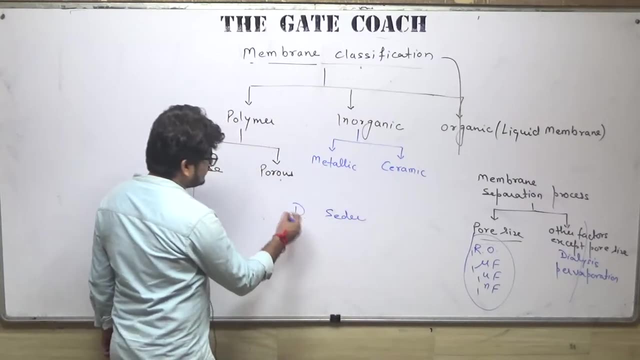 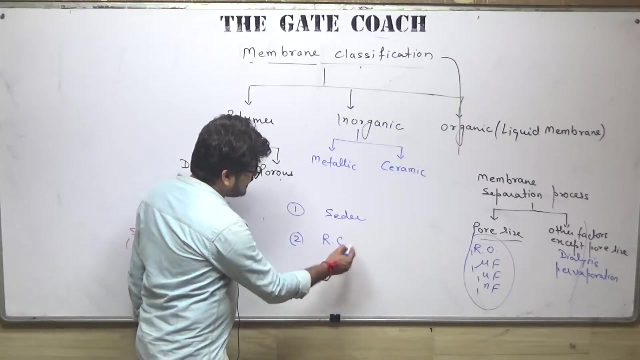 I'm writing once more time If anyone joined late. Okay, For the membrane suppression part, you can go through with Cedar. Separation processes, principles, mais Cedar, We will attend this. cedar, that is one book and second is rc, volume 2. these are the two good books which you can use. 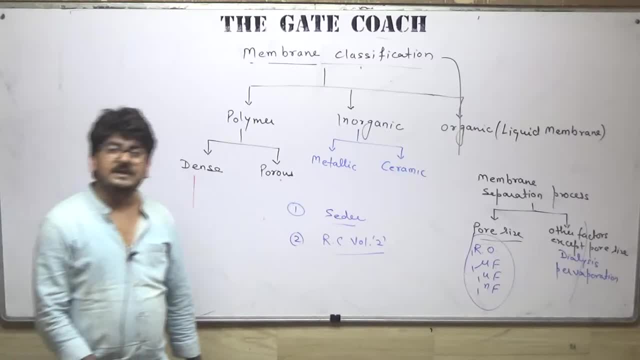 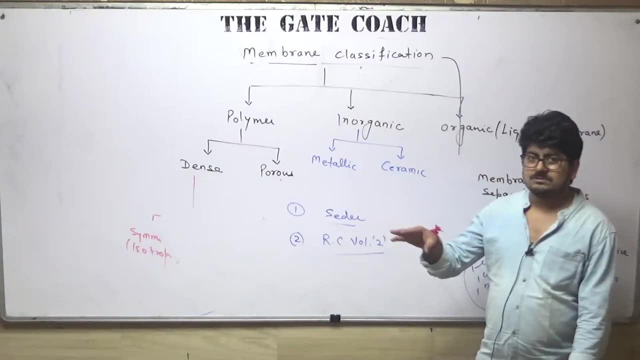 for the reference. okay, there are other books as well, like bk dutta. in that book as well, master membrane separation part is given. but i will suggest you please don't go with that book. okay, initially, for the first time, when you are reading all these things, first prepare all the things from. 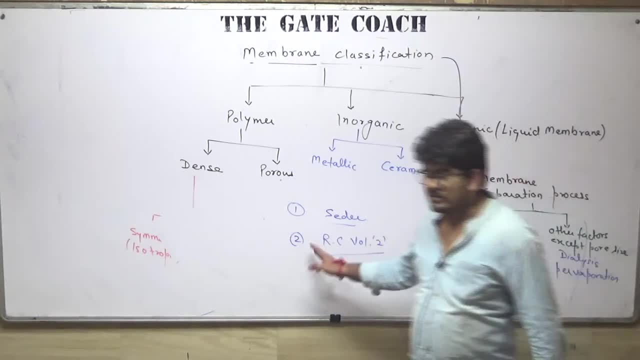 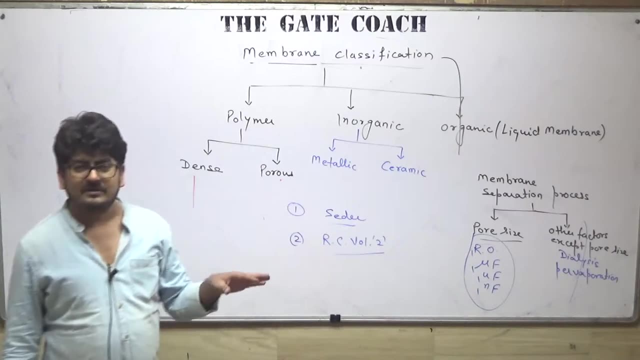 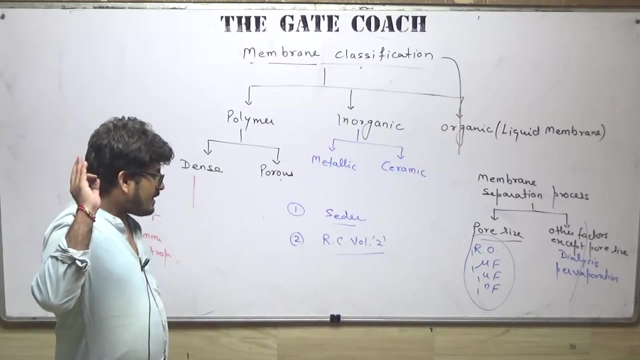 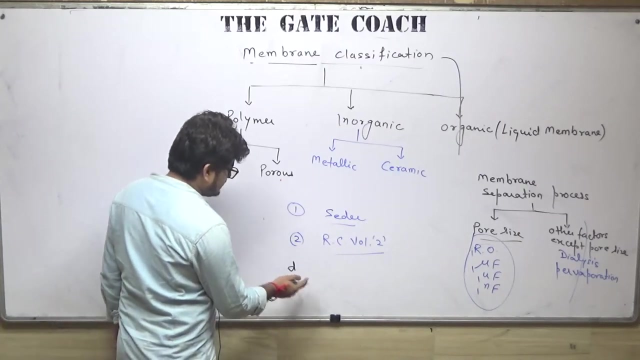 the good books, those are cedar and rc, volume 2. you can refer any one of them, okay, and if you don't have the soft copy, you can download that on from the google. it will be available. and still, if you are not able to do that thing, then you can send your. you can uh what you can do. you can join our.